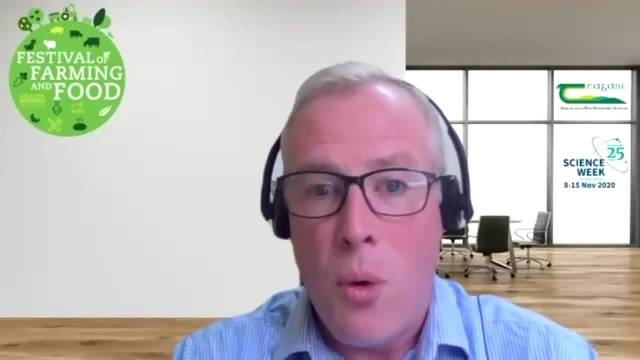 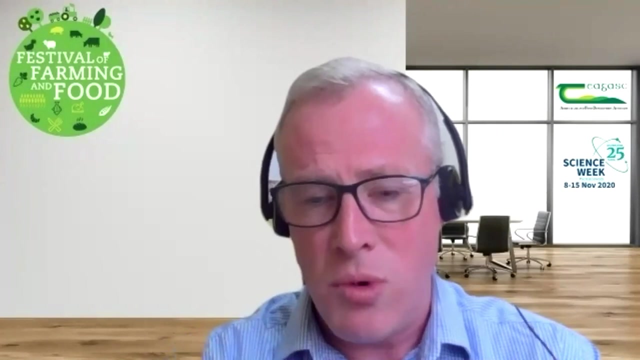 Johnstown to share with us their idea of why soil health is our wealth. We're going to be playing a video very shortly as well to give you an idea of the work that happens down in the beautiful Johnstown Castle Estate. Now you can get involved as well, and we are delighted that all of these 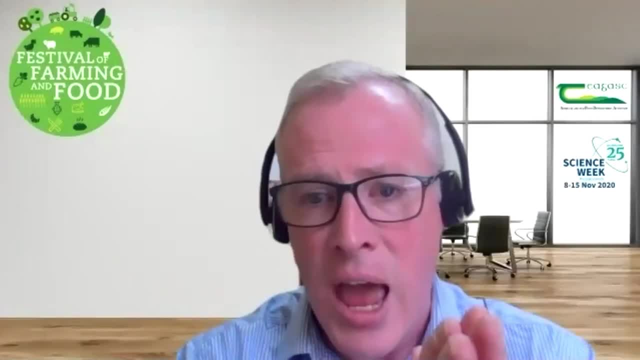 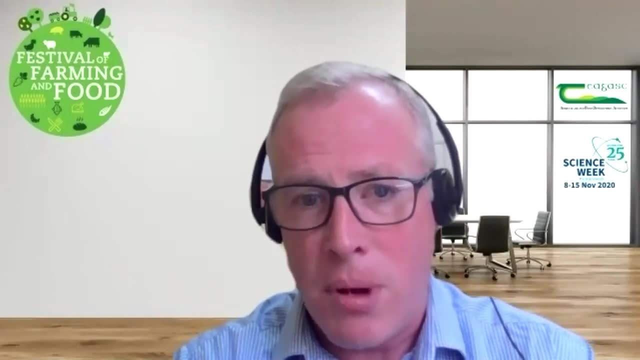 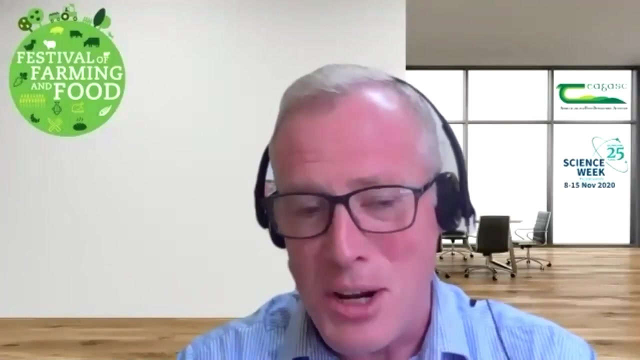 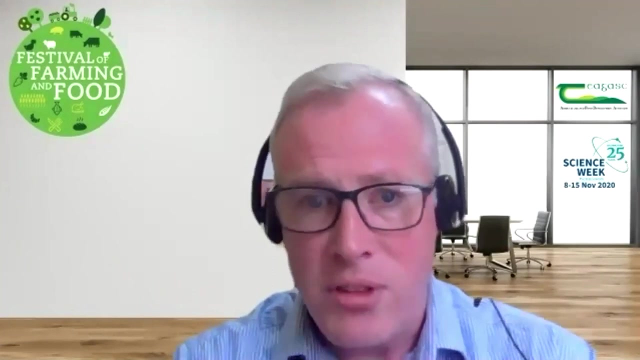 events this week. they're free for you, thanks to Chagas and Science Foundation Ireland, But you can also get involved in terms of asking questions or making points. So if you have any questions, we will certainly try and get to them over the next hour or so, And 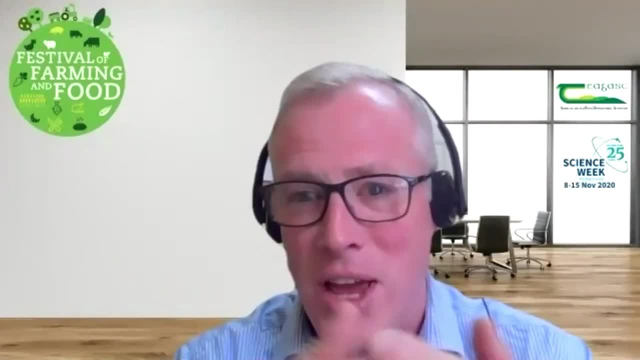 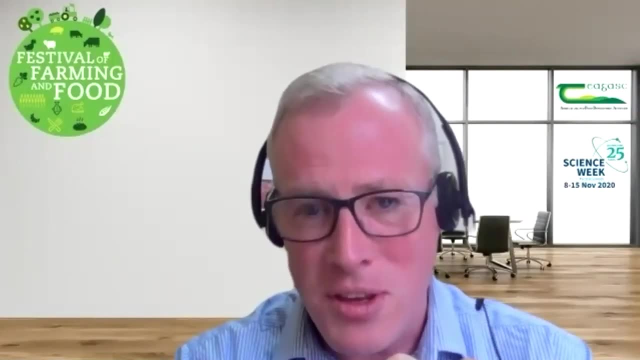 if we don't get to them. we will certainly do our best to try and answer your questions privately as well, And our team of experts are more than happy to share their expertise with you Now. we will also be emailing you a little bit later on, looking for your questions, So if you have any questions, 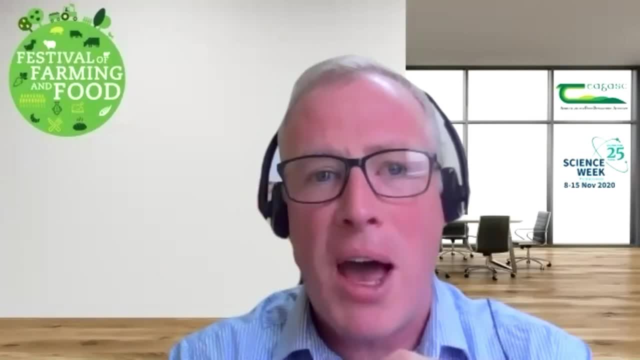 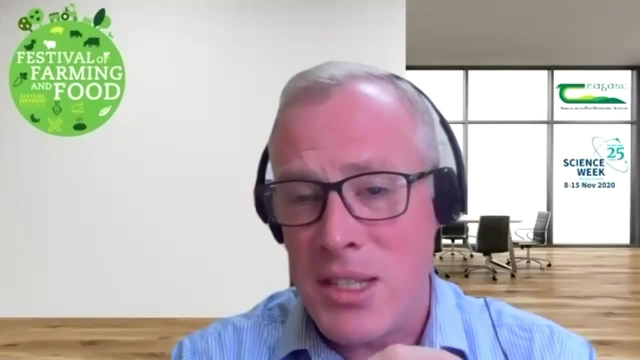 we will certainly try and answer your feedback, So please do help us, maybe tell us how good or maybe how bad I was and how good everybody else was, by answering that a little bit later on, All right, Well, we have been down to Johnstown to film what's going on there And, as I said, 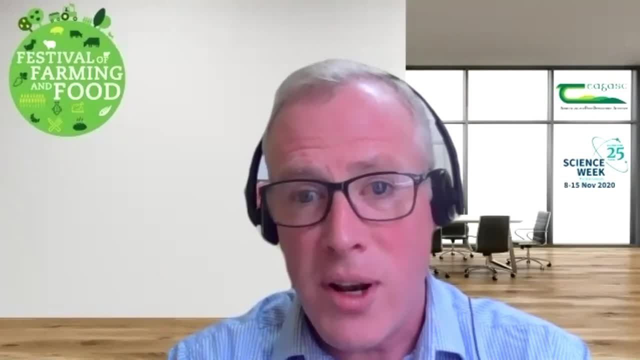 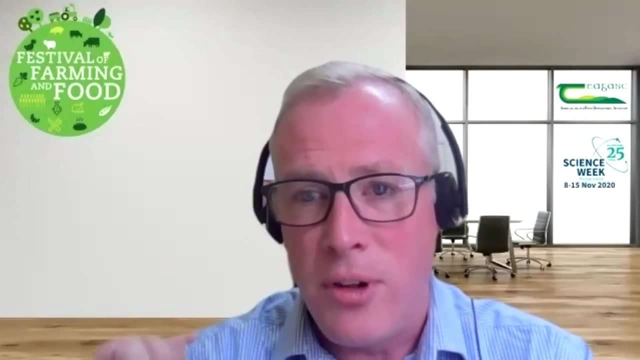 a little bit. later on, we will be going live to the experts, Some of them you're going to actually see now in this video. So for the next 20 minutes or so, sit back and have a look at this wonderful video that we're going to bring to you right now. 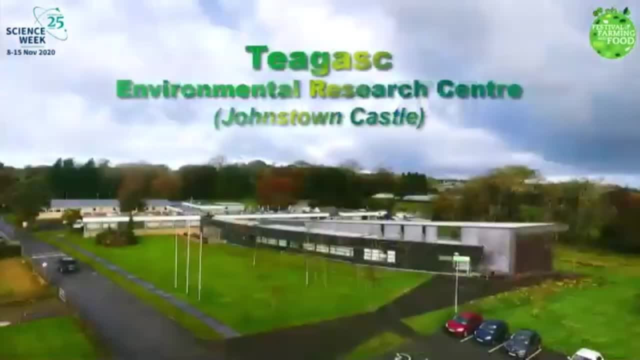 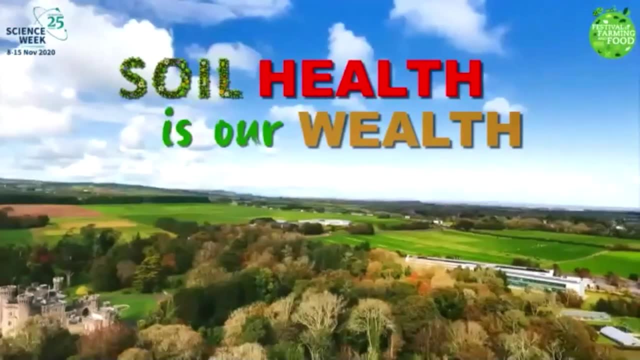 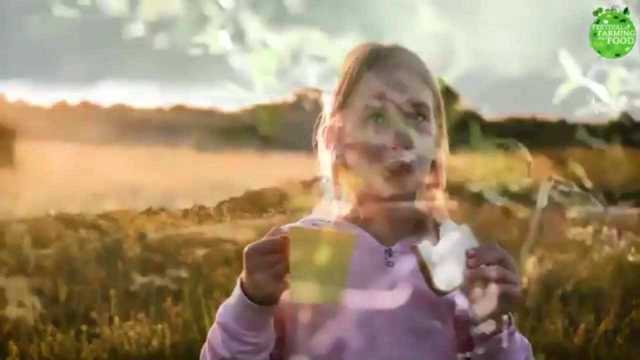 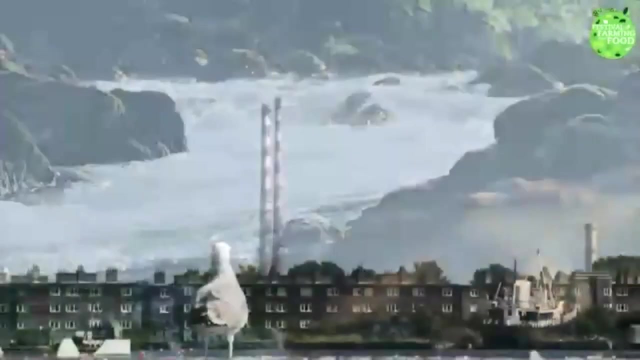 Did you know that soils are the basis of all of the food that you eat? They also provide a range of other services, such as purifying water, storing carbon from our atmosphere and providing a home for biodiversity. They also support all of the buildings and homes that we have on the 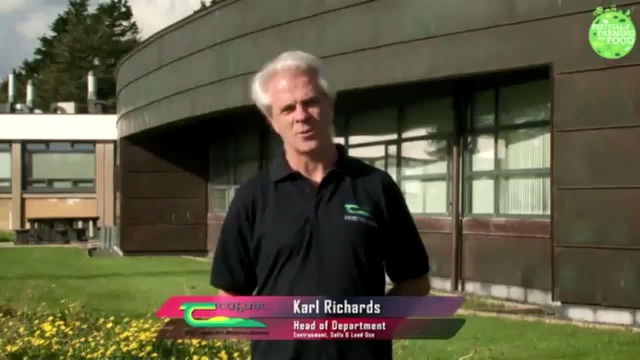 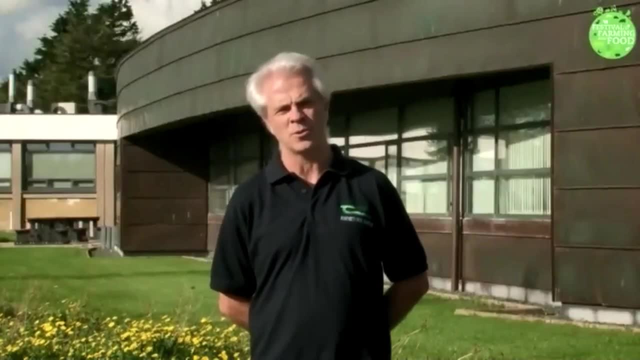 planet. Here at Chagas Johnstown Castle we've been working with the experts on a number of issues. We've been working on soil science for the past 50 years. The initial focus was how to improve our soils to increase food production after World War II. Our focus has now changed to 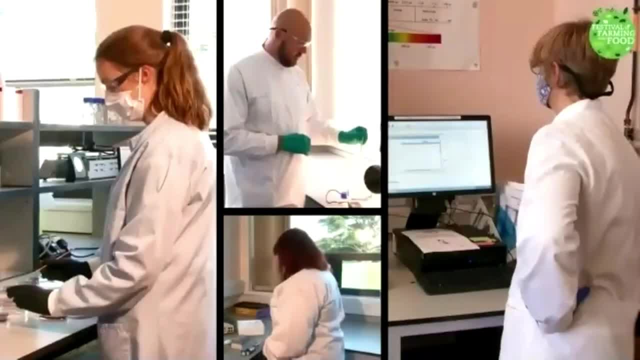 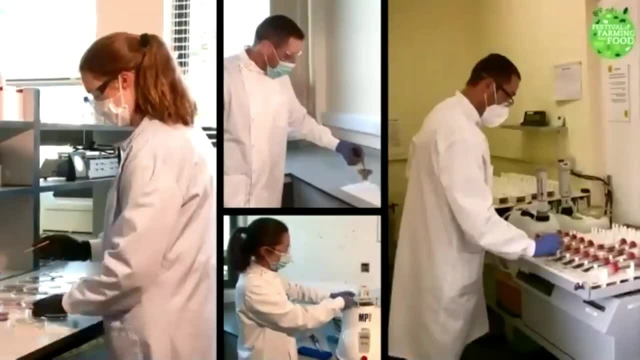 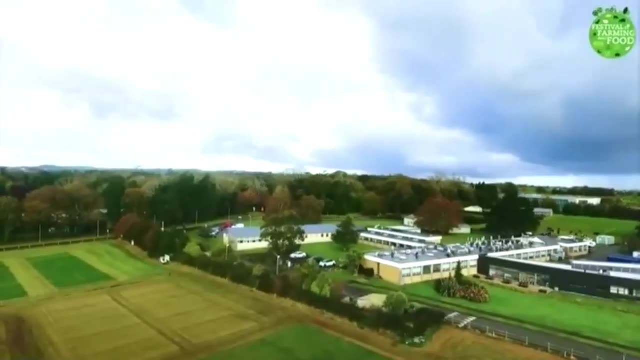 more sustainable food production systems. In our center we have a range of scientists working on different themes such as biodiversity, carbon sequestration and greenhouse gas emissions, water quality and on soil science itself. Our research here focuses on soil health and 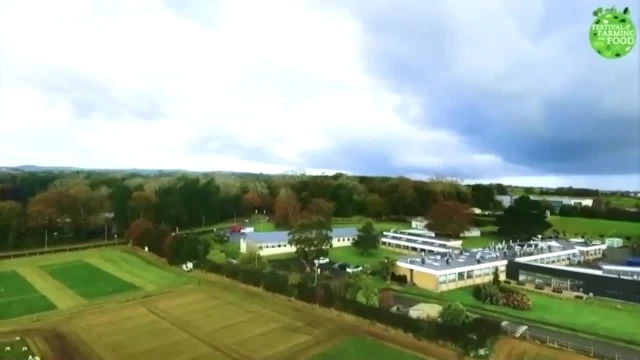 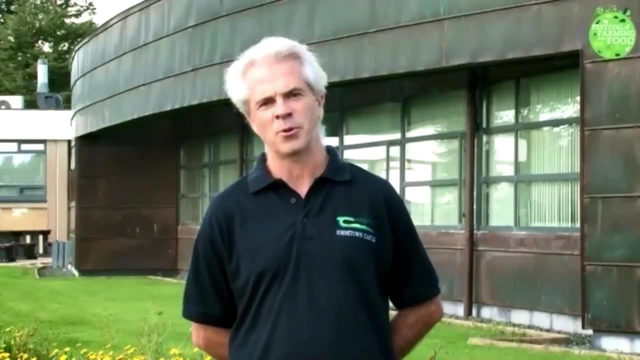 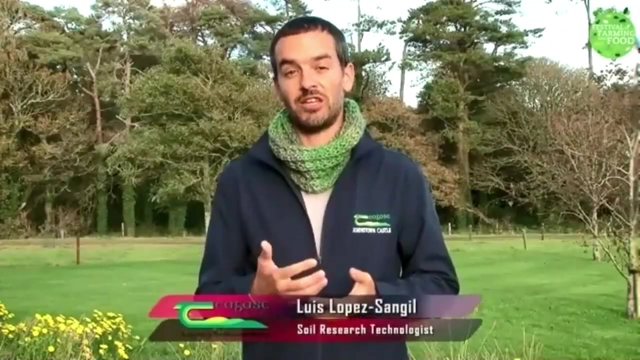 its importance in both underpinning sustainability and producing food. In this video, our scientists will give you an overview of the various research projects that they're carrying out on this very important topic. Historically, healthy, fertile soils have been the main reason behind the rise of civilizations. 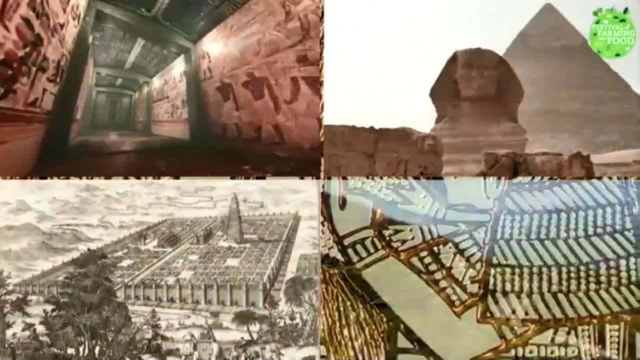 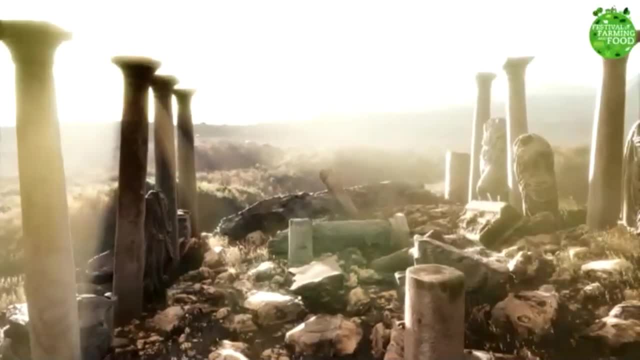 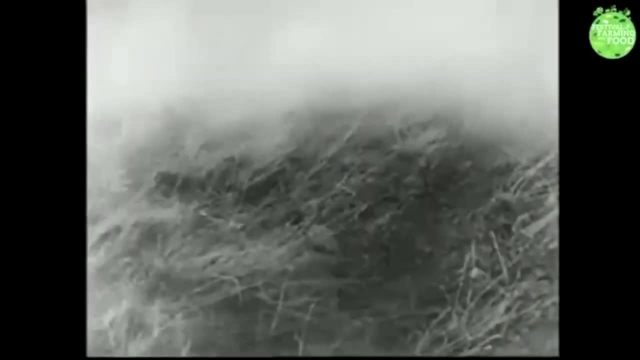 We have the Egyptians, the Mesopotamians, the Indo-Bale, the Incas and many more. But likewise, soil degradation has also been the trigger for the collapse of societies. We have the example of the Greeks, after central countries of soil erosion, Also more recent disasters, For instance the Dust Bowl in the 30s. 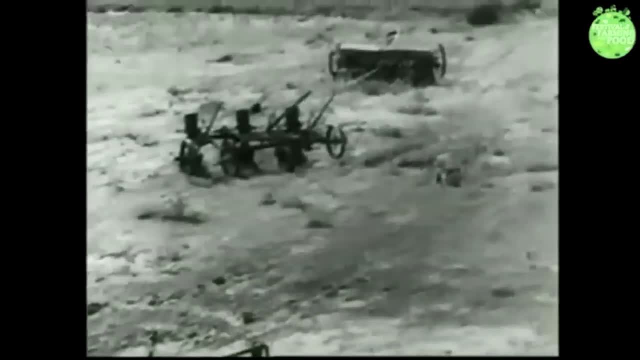 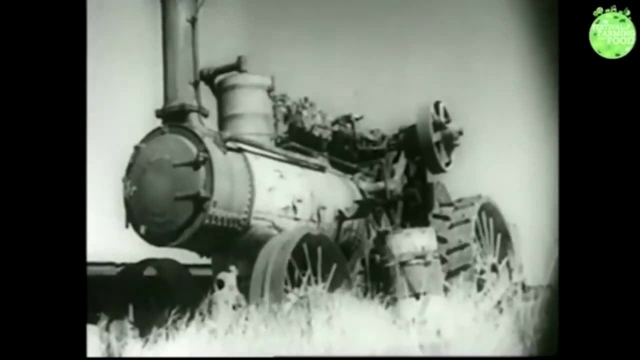 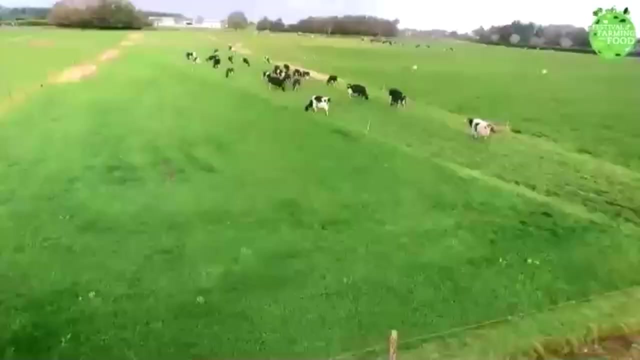 with massive dust storms due to wind erosion of bare soils. This was after just a decade of overfarming, deep plowing and loss of organic matter. These poor soil management practices ended up causing enormous economic and agricultural damage. Human well-being relies on healthy 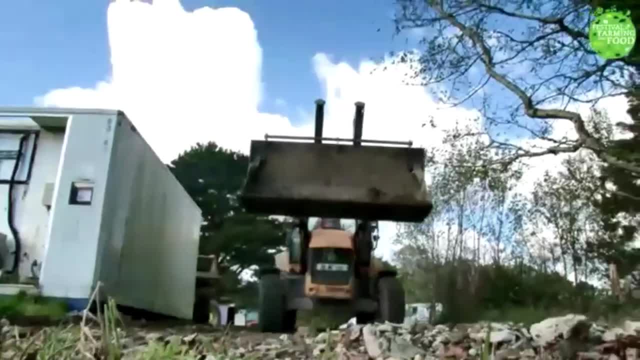 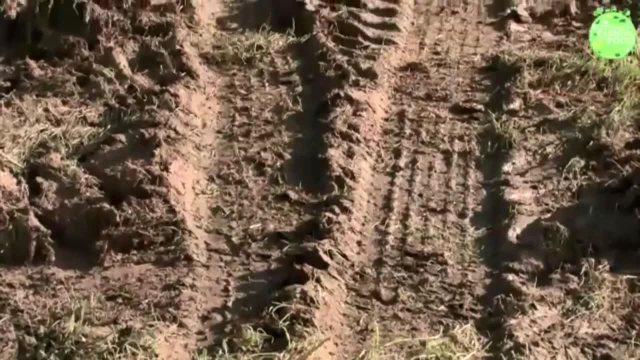 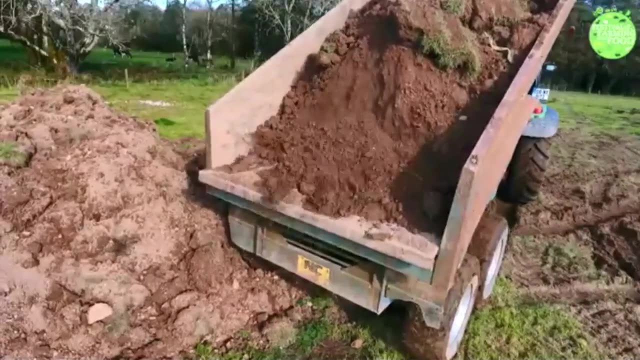 non-degraded soils. To put this in context, soil degradation is globally responsible for the loss of 12 million hectares of productive fertile agricultural land. This is more than the area of the whole of Ireland being lost every year. so it's important to treat soils as valuable resources and manage them sustainably for future generations. Healthy soils can be defined as multifunctional living systems with a continued capacity to sustain plant, animal and human life. Only living things can have health, so it's important to see soils as living and diverse ecosystems full of life. Soils are multifunctional: They produce 95% of all the food and fibre for humans and livestock, but they also provide other important services for society. 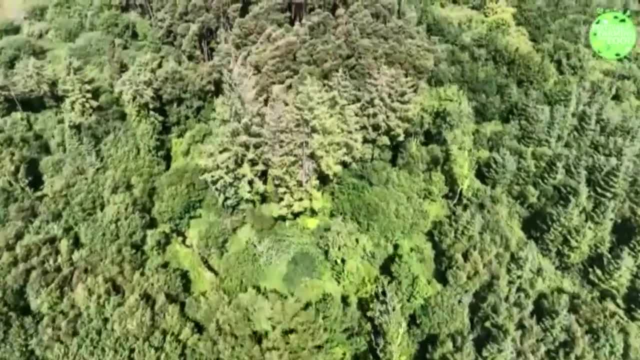 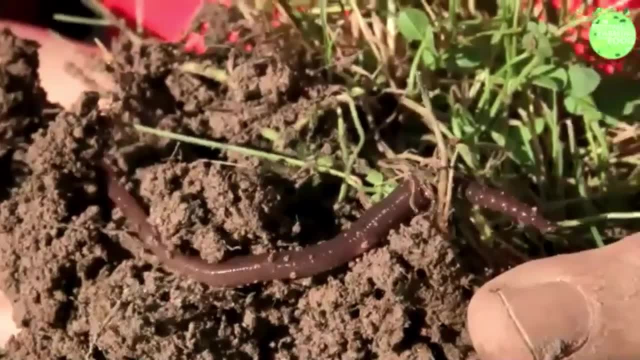 They regulate climate by carbonation. They capture CO2 through plant photosynthesis and keep that carbon in the ground as soil organic matter. Soils are the place on Earth with the highest biodiversity and they are the source of many useful chemicals and medicines. 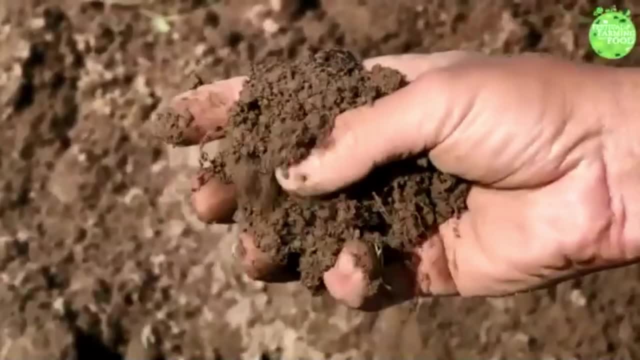 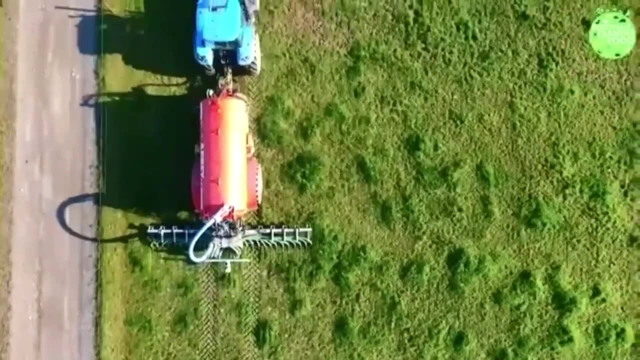 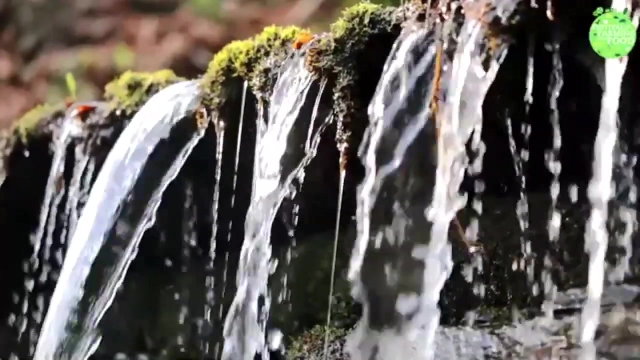 There are more living organisms in a handful of healthy topsoil than all the humans who have ever existed on Earth. Soil microorganisms also recycle our waste byproducts from food production into useful nutrients for food, And healthy soils also purify water and minimise the risk of flooding downstream in our towns and cities. 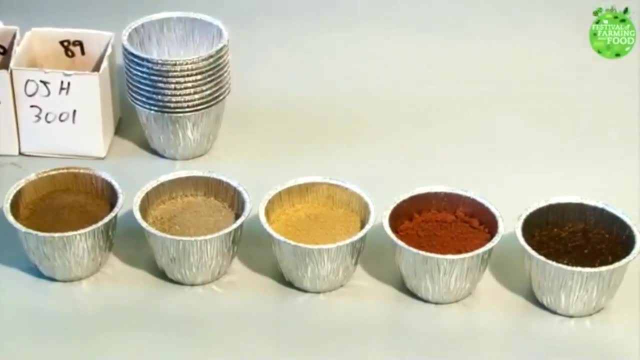 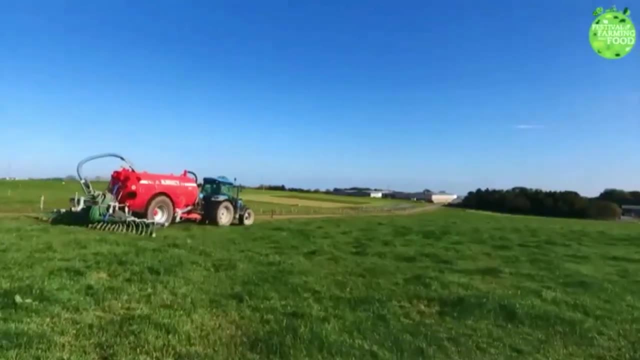 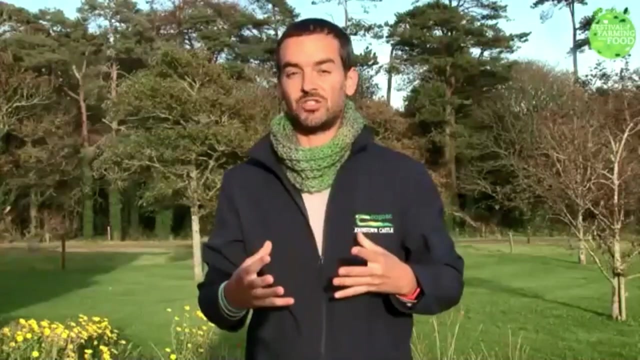 There are many different types of soils, each one with a different ability to carry out these functions. Here in Ireland, our main issues with soil degradation are compaction, mainly from farm machinery, loss of nutrients, contaminating our water streams, and erosion. Society needs to better understand the practices that lead to soil degradation and also those that are harmful to the environment. 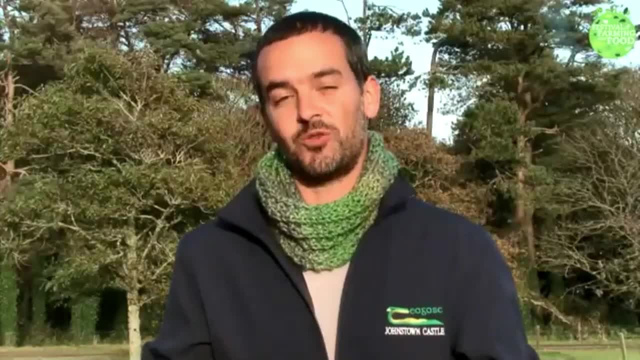 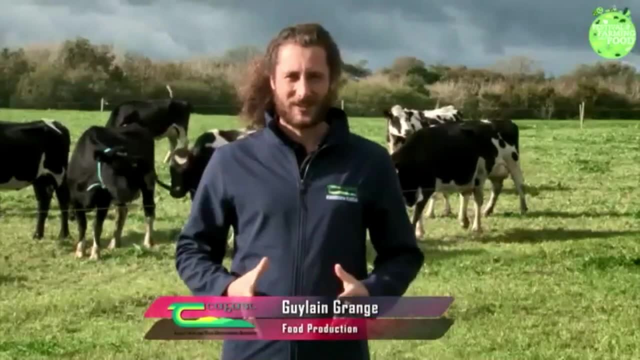 Soil is an essential resource that can heal and improve our soils. That's what we are here for at Chagasque. Hello, I'm Guylain Grange. I'm a third year PhD student here in Johnstone Castle and I'm working on plant biodiversity in grasslands. 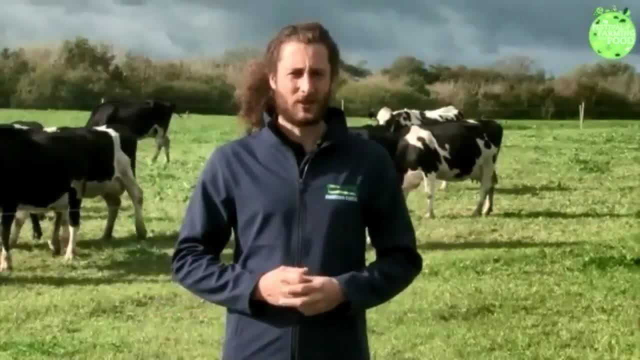 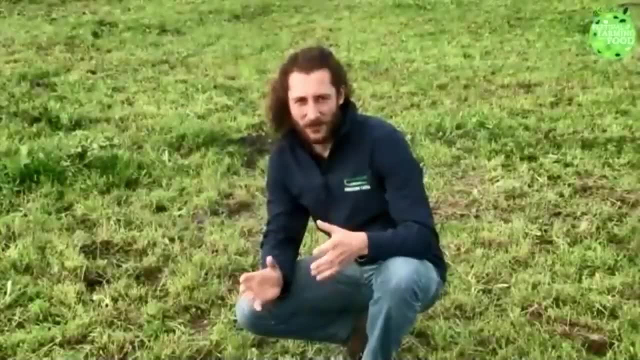 I'm going to talk to you today about the productivity function of the soil, illustrated by these animals here that produce milk to feed the humans. Can you imagine growing vegetables, barley or wheat without soil? It is actually the same for the grass. It is actually the same for the grass. 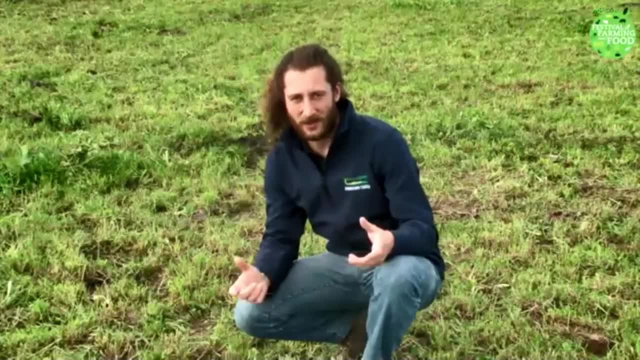 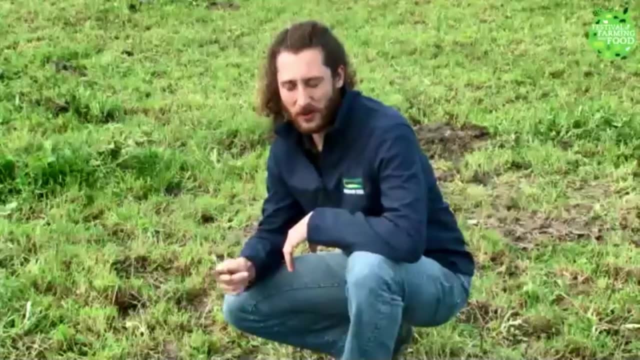 The grass needs good soil for growing. What is a good soil? A good soil would be a soil providing them with nutrients and also that can hold the water. So with good water retention you can balance the periods without rain or with too much rain. 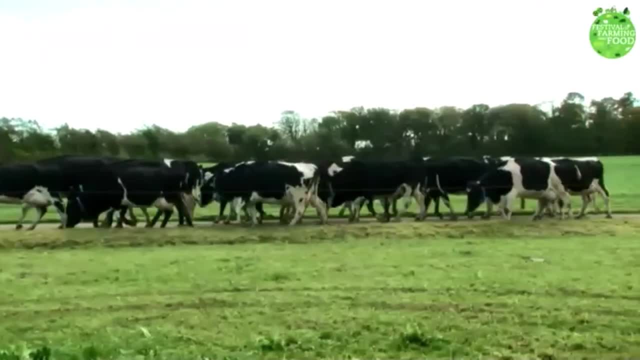 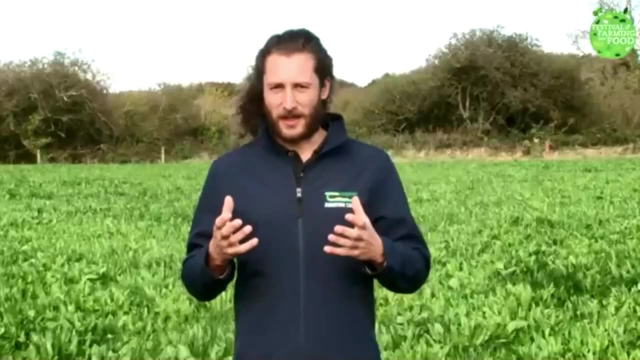 The best experts we have today to take care of our soil are farmers. Every day they take decisions to keep the soil fertility high. This way they are sure they will have good grass to feed the animals. This way they are sure they will have good grass to feed the animals. 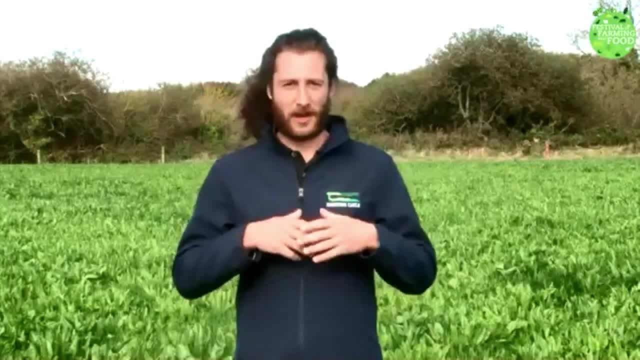 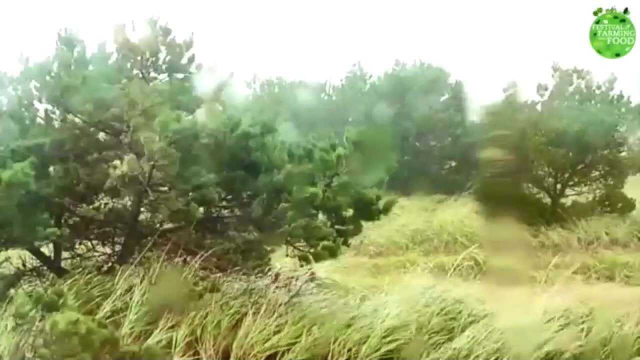 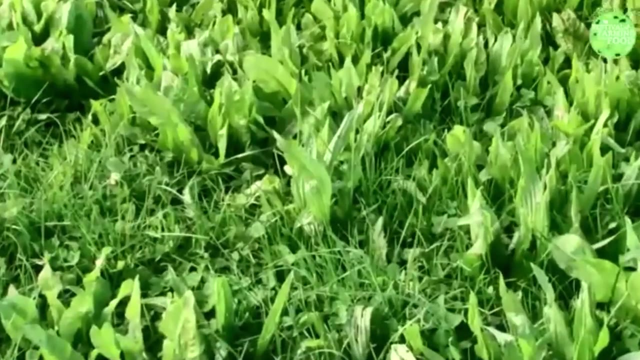 And so they can sell good milk or good meats for everybody to eat. well, But the climate is changing. We expect less rain in summer, more rain in winter, and there are concerns raised about the use of fertilizer that could produce greenhouse gases. To answer these questions, then, we are trying to develop here in Johnstone a grassland that could cope with that. 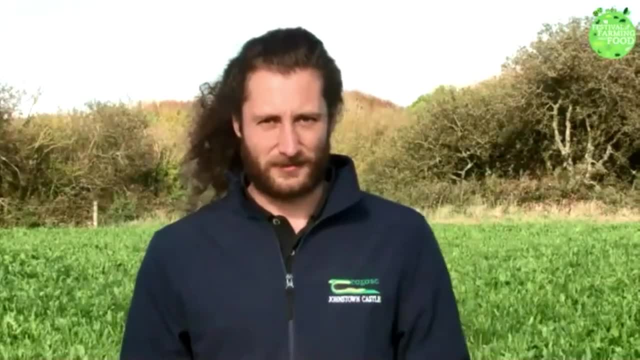 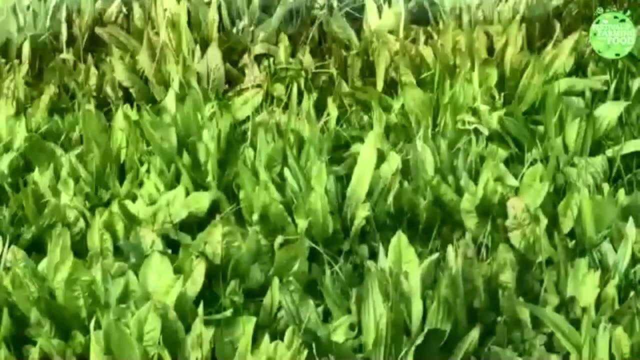 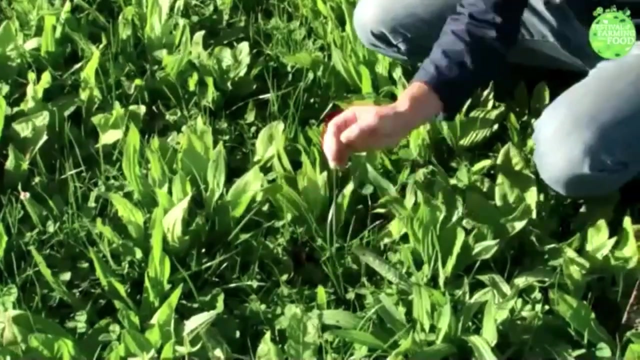 So cope with less fertilizer and less rain in the summer. So cope with less fertilizer and less rain in the summer. We are testing the ability of multi-species swards to cope with droughts and also with reduced fertilizer use. To do so, we mix grass, herbs and legumes like clover. 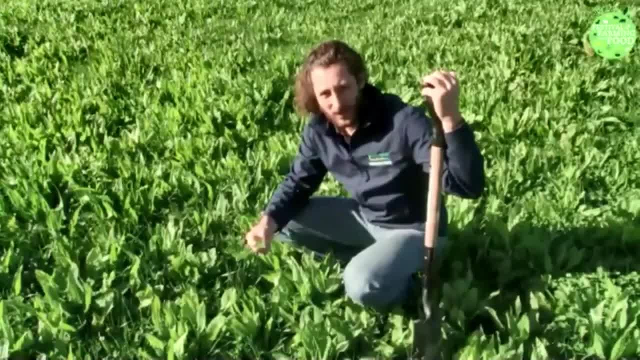 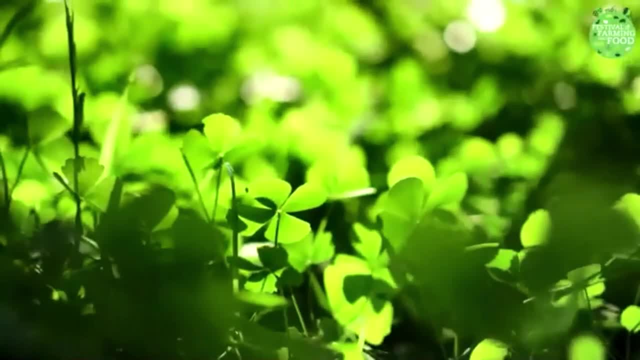 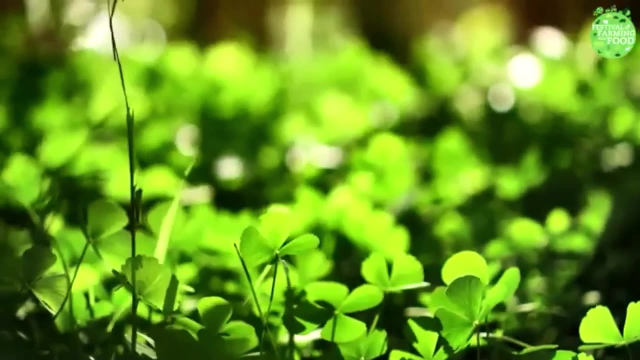 And so interacting together. they can benefit to each other and maintain good productivity with low inputs. Clover, for example, can increase soil fertility, And other species like herbs have long roots That can bring carbon deeper into the soil. We will now see why carbon storage is an important thing. 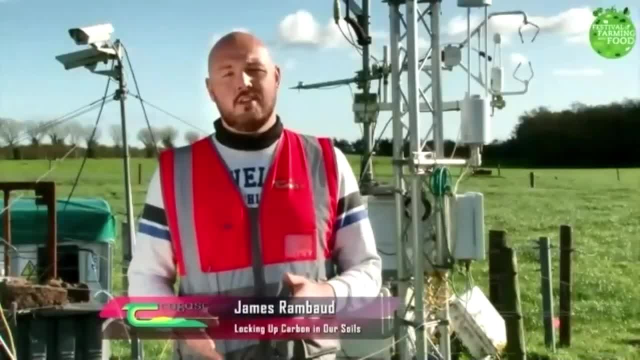 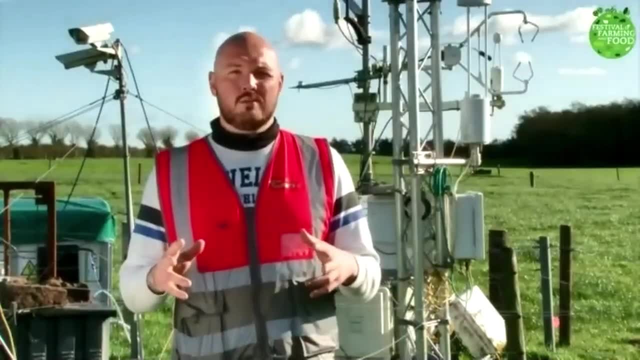 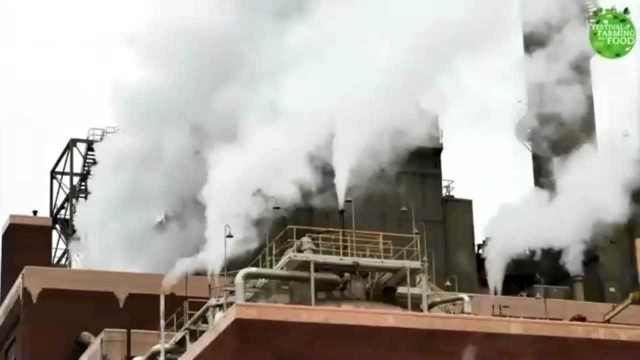 Hi, my name is James Rambo and I am the soil carbon sequestration technician here in Johnstone Castle. The great environmental challenge of this century is the need to stabilize atmospheric concentrations of greenhouse gases. In order to achieve this, we, the caretakers of this planet, need to reduce our dependence on fossil fuels and find ways of removing greenhouse gases. 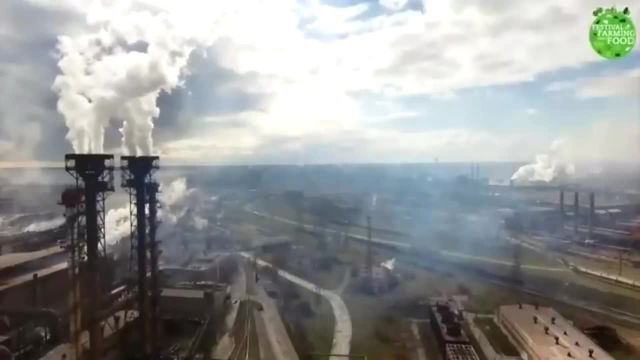 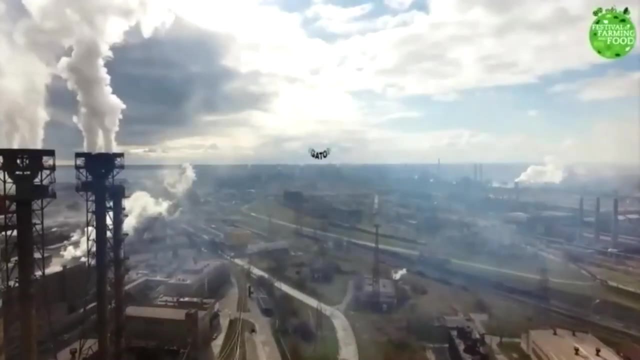 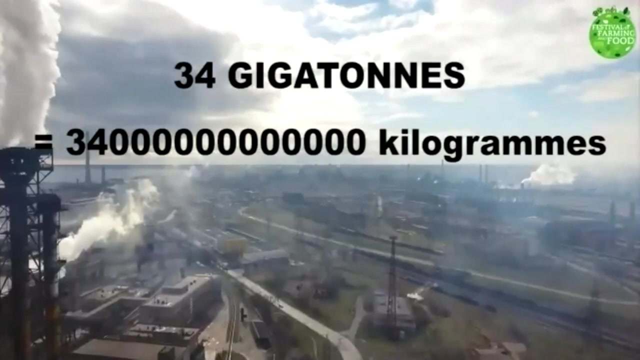 from our atmosphere. The scope of the issue we face is very challenging. Currently, sources of greenhouse gas emissions from human-related activities release 34 gigatons of CO2 into the atmosphere annually. At present, there is no hope for a radical reversal of these rates of emission. 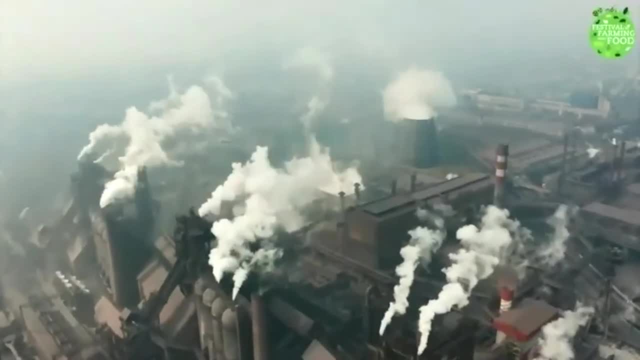 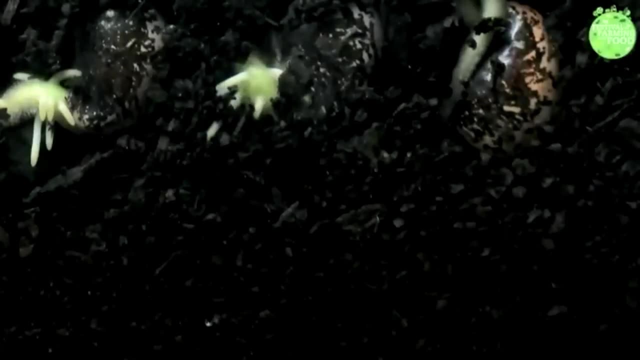 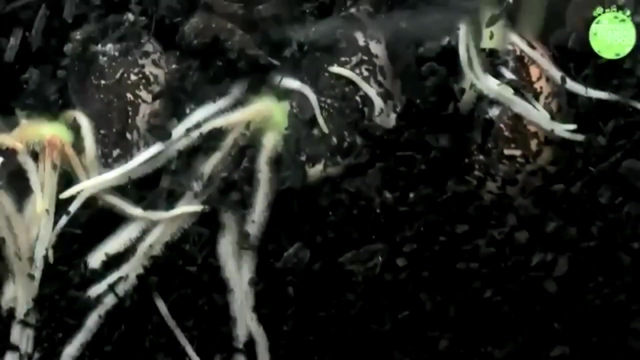 Aside from reducing our fossil fuel use, there is one method we can all use to try and stem the rate of greenhouse gas growth. This involves the sequestration or capture of atmospheric CO2.. CO2, as organic carbon in our soils. Carbon stored in soils is very beneficial. 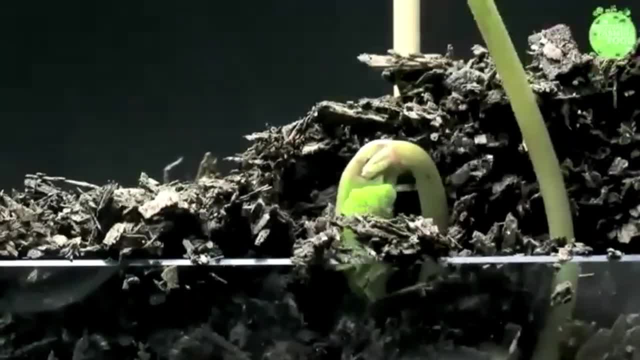 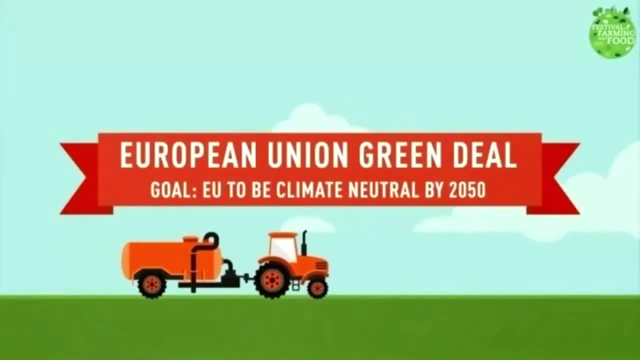 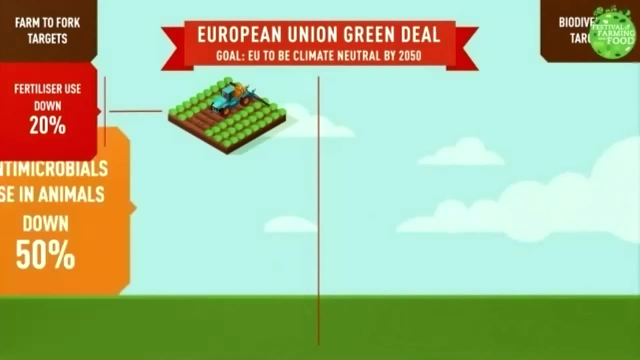 It improves their structure, their water holding capacity, their productivity and their biodiversity. Europe's recent Green Deal aims to prevent climate change by bringing down carbon emissions significantly by 2050.. Beef and dairy production are the largest Irish agricultural industries and the main cause of the sector's emissions. 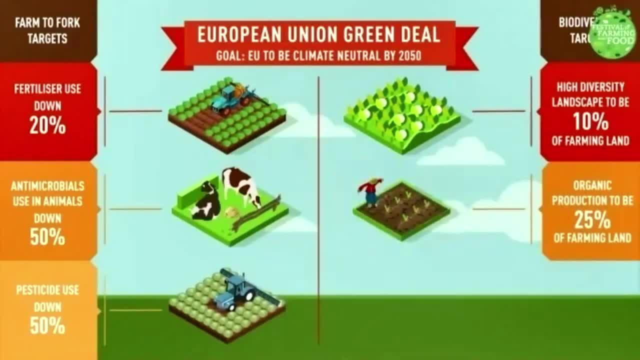 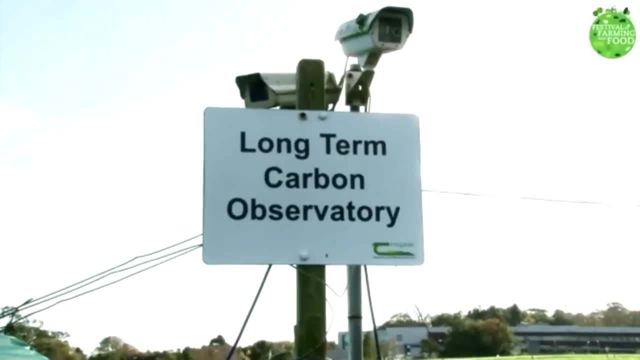 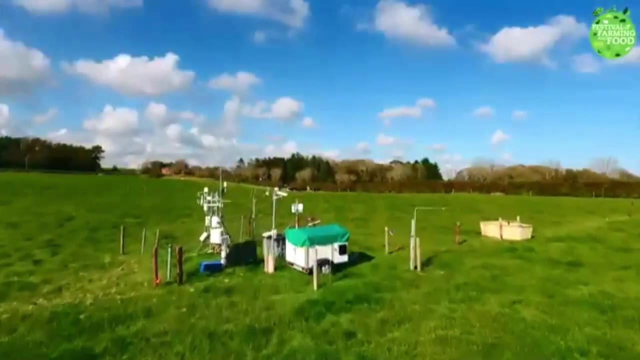 Reducing the national herd's carbon emissions as much as possible, while feeding a growing population is going to be very challenging. Here at Chagas Johnstown Castle, we use a range of equipment to monitor and track CO2 and soil carbon, such as eddy covariance towers, elemental analysers and pneumatic soil corers. 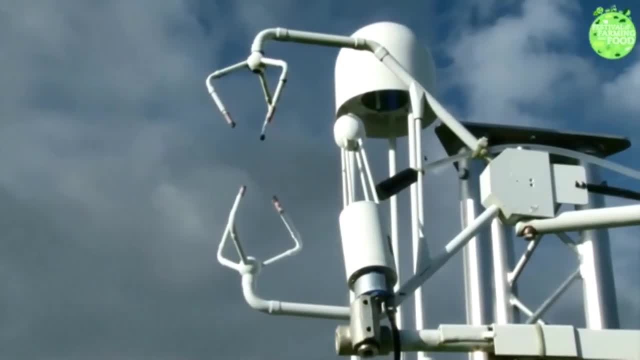 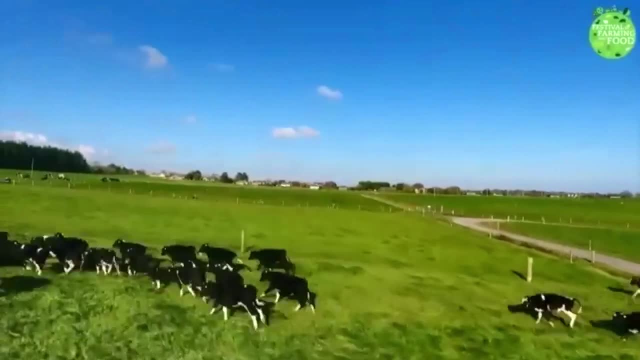 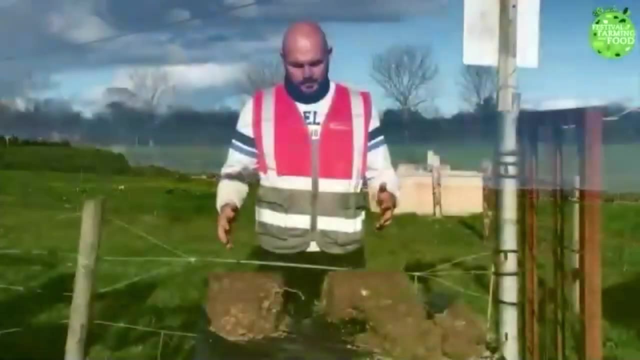 These enable researchers to look into improving the national herd's carbon footprint. The main strategies being investigated in order to achieve this include improving efficiencies, adopting low emission technologies and carbon sequestration. Okay, so I'm going to talk to you briefly about what exactly soil carbon sequestration is and how it happens. 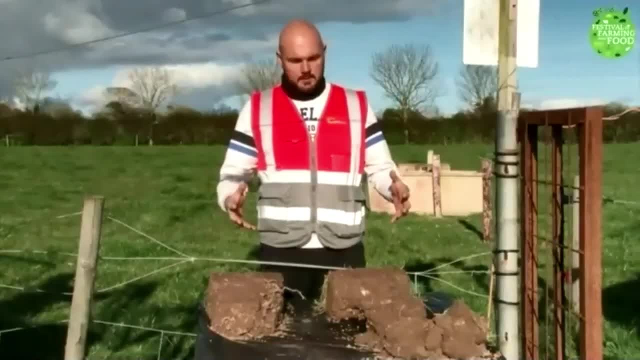 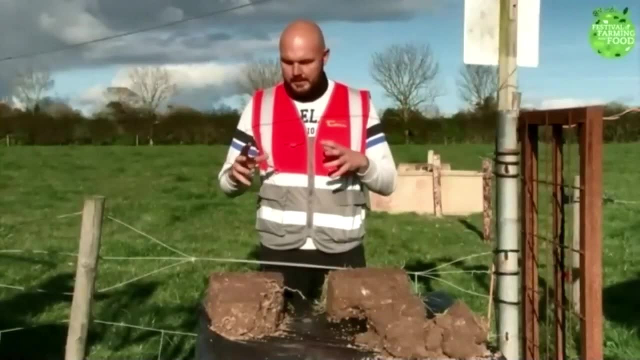 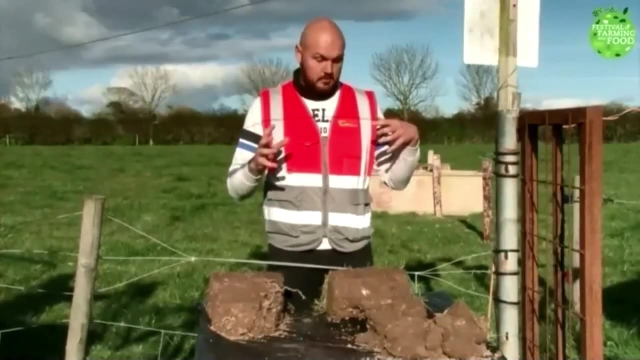 So we have our plants which, as we all know, photosynthesize. They use solar energy combined with carbon dioxide- which is our big problem word at the minute- and water to create simple sugars such as carbohydrates. So they use these simple sugars to grow biomass. 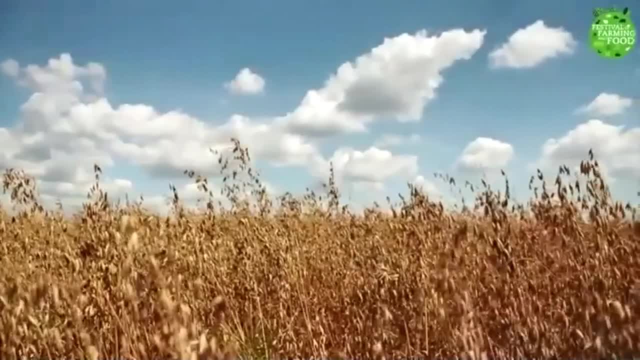 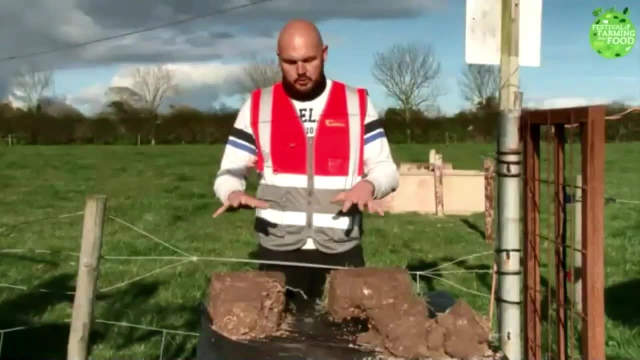 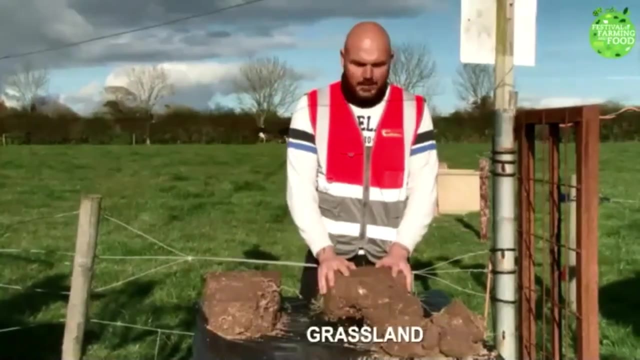 This biomass is above and below the soil. Now, following decomposition, it eventually becomes a stable form of carbon in the soil. I'll just demonstrate here three types of sod that I have: One from a woodland, one from a long-term grassland and one from a tillage soil. 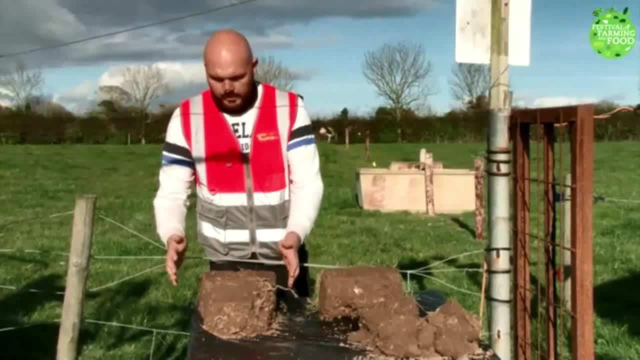 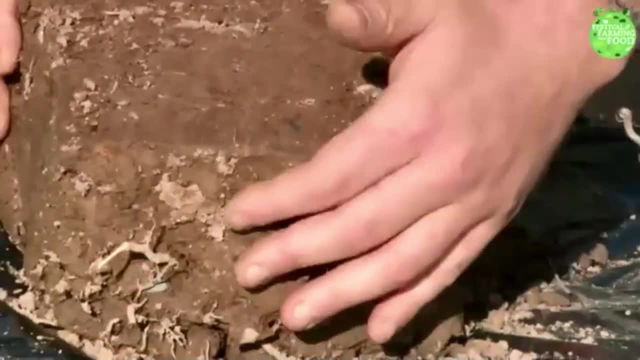 So we see here, with the woodland which has been woodland for 20 plus years, we have deep, deep roots which go right to the bottom of the sod. You can see it's very stable, It's in one piece. The water is well held within the soil. 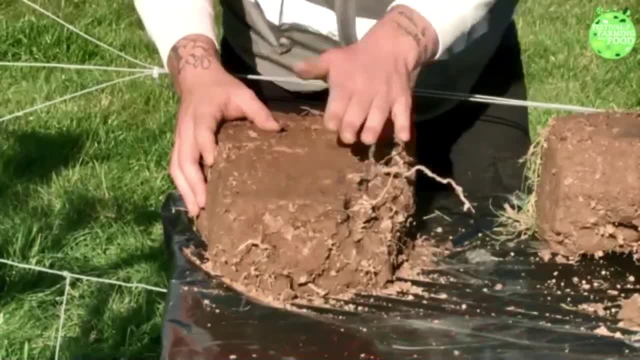 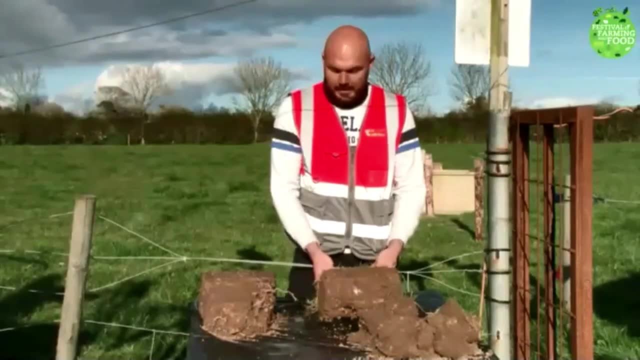 There is ample pore space for water to move through, but not enough pore space for water to wash away the soil. Here we have our grassland, which again, has been grassland for 10 years plus You can see it's much shallower. 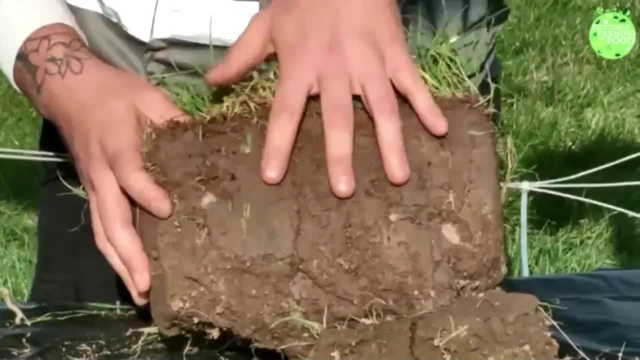 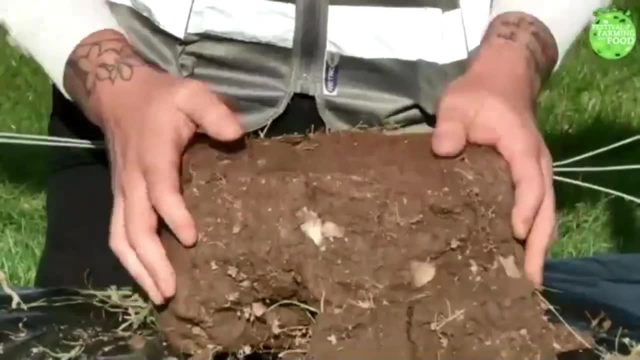 There's quite a dense biomass on the top here. They're quite deep rooted, not as deep as the woodland, but it holds firm together. It's well structured. Again, another very good method to sequester carbon. And then we have our tillage. 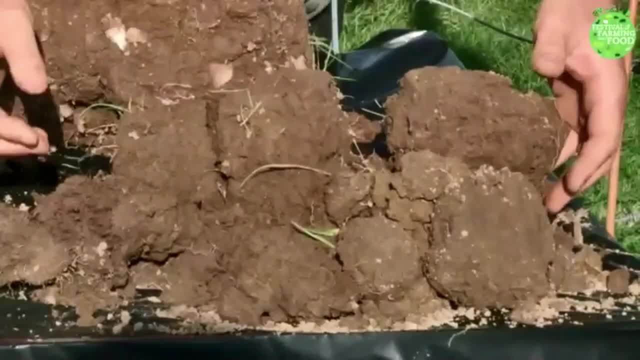 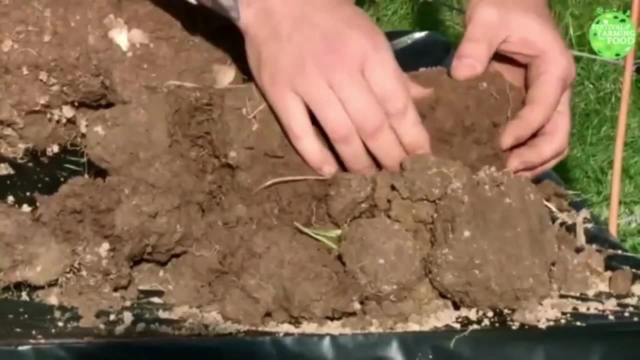 And the tillage. as you can see, it's very crumbly. It doesn't really hold its structure too well. There's not really a great root mass, very compared to the woodland. There's very little biodiversity in the soil. 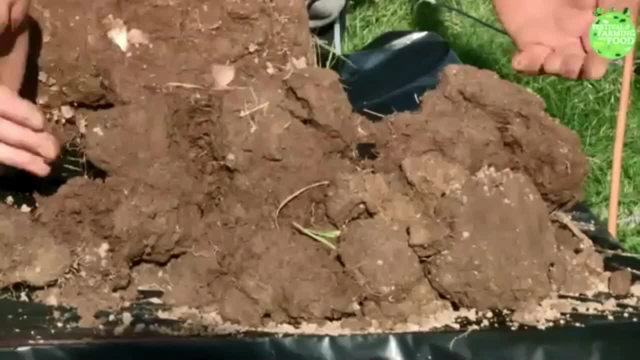 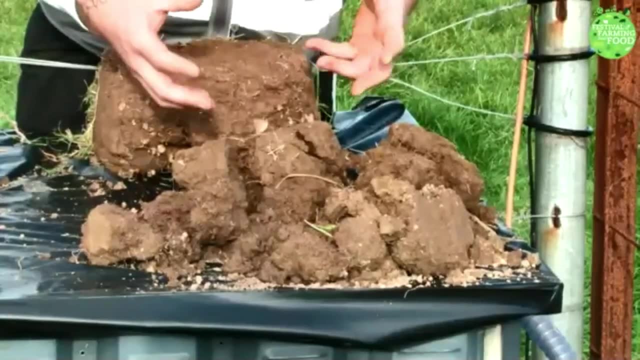 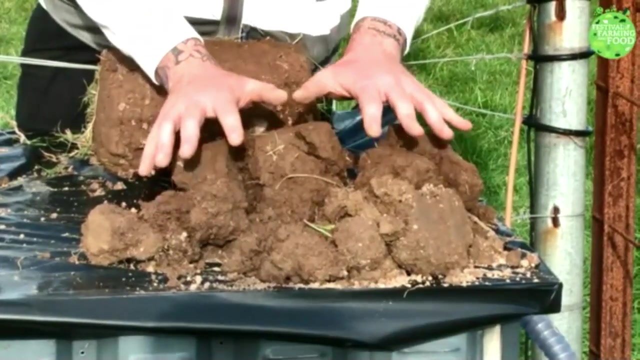 However, this is the sod that has the most potential to sequester carbon. With careful management, such as minimum tillage or we're looking into very deep plowing, etc, etc. there is an awful lot more potential to sequester carbon long term in tillage soils. 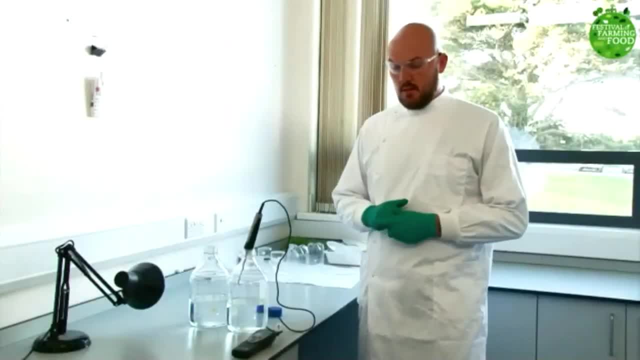 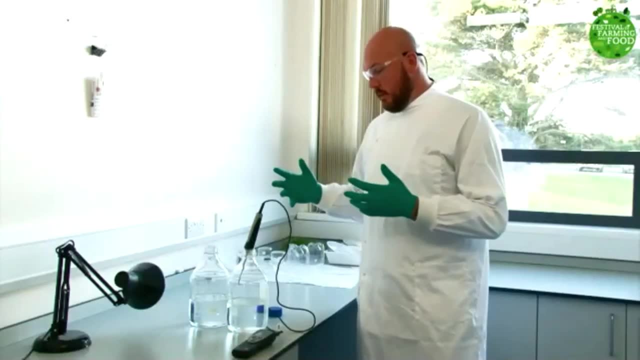 Okay. so when we hear carbon dioxide, the majority of us think of it as being a bad gas, But in actual fact, it's a normal constituent of the atmosphere. The issue is where there's too much carbon dioxide, So I have set up a little bit of an experiment here. 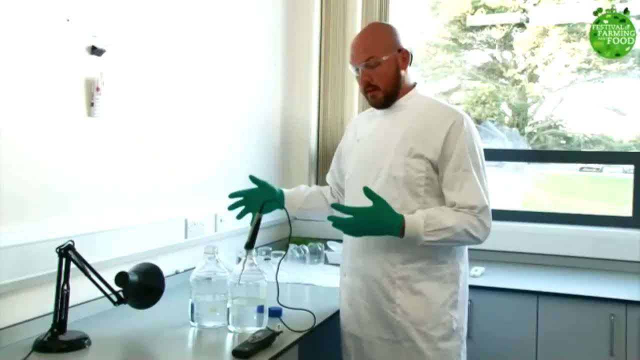 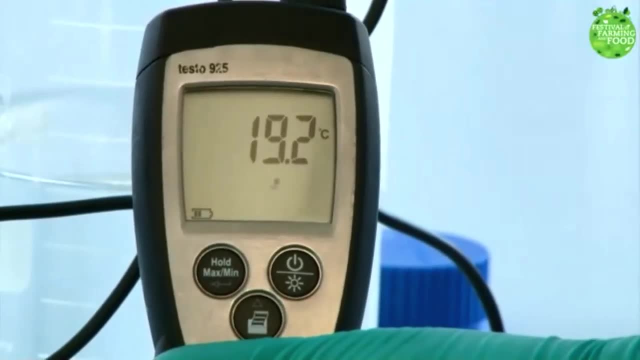 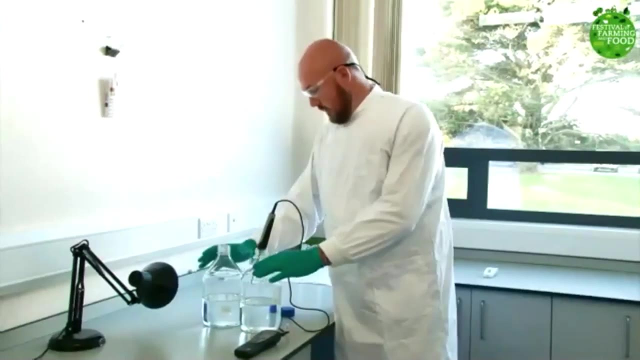 just to demonstrate exactly what happens when there's too much carbon dioxide present in the atmosphere. So we have a little temperature sensor here that's reading 19.2 degrees at the minute. Both these bottles have distilled water and are filled with ambient air. 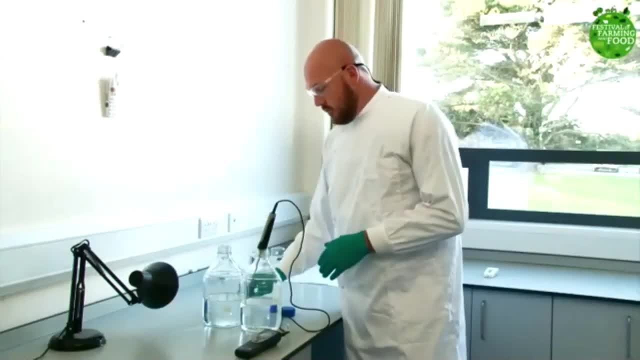 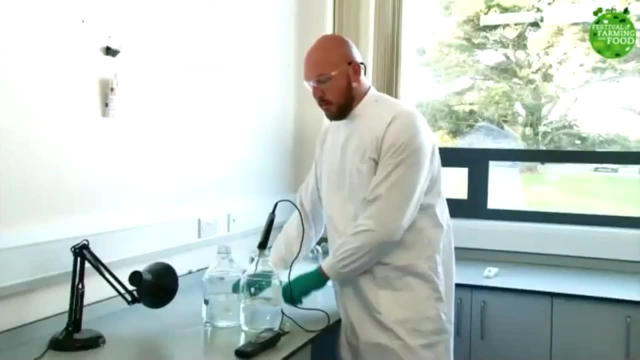 So they have normal levels of carbon dioxide. I have two effervescent tablets here that I'm going to drop into one, which will release carbon dioxide. I will close the lid on both and then add a heat source, And normally what we should see is: 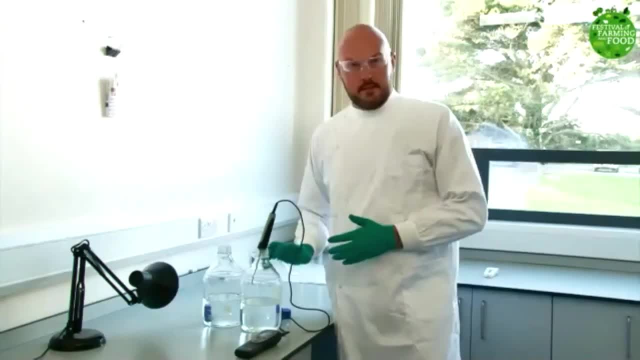 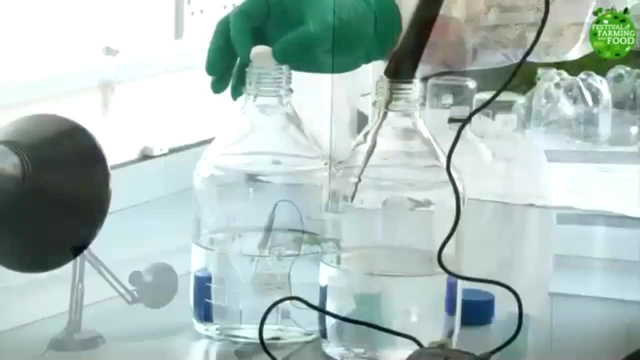 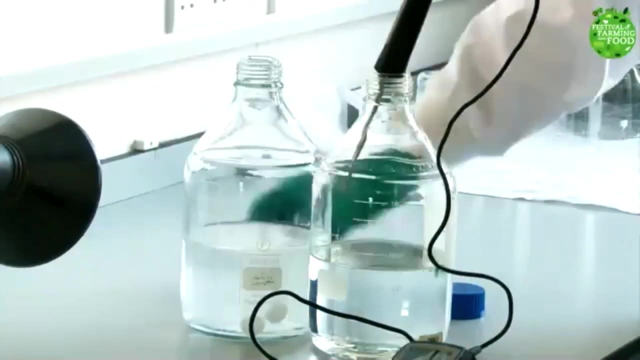 an increase in temperature over the standard in the carbon dioxide bottle versus what is normal ambient air. So I've just dropped the effervescent tablets in. You can see it's starting to fizz. now I'm just going to place the lid on top. 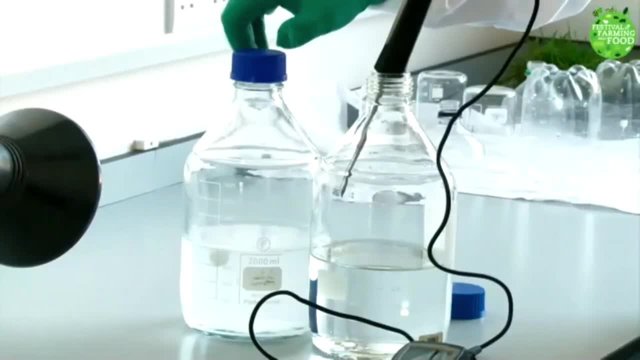 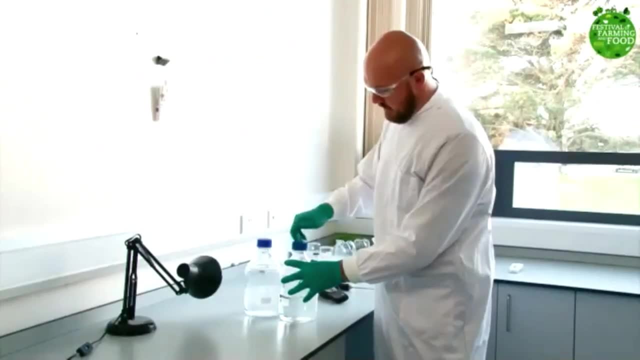 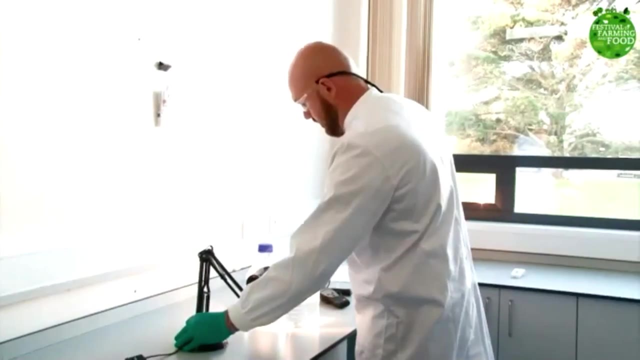 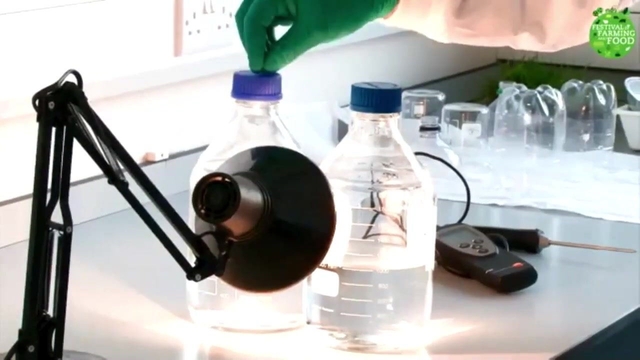 and let the carbon dioxide build up inside the bottle. Okay, so I'm removing the thermometer, adding the lid to our control, clicking on our heat source and placing it in front. So now, in theory, our carbon dioxide bottle should heat up faster and to a higher temperature. 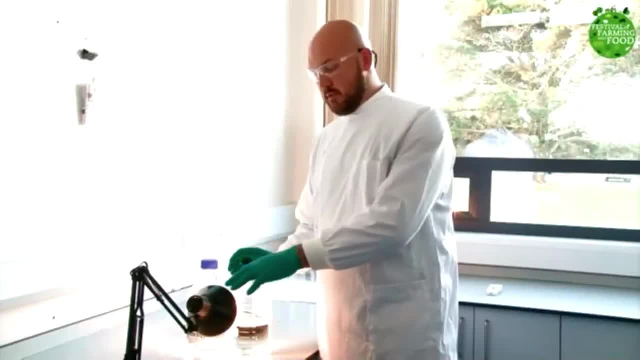 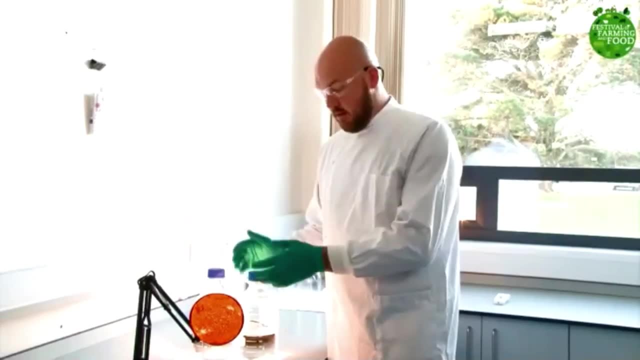 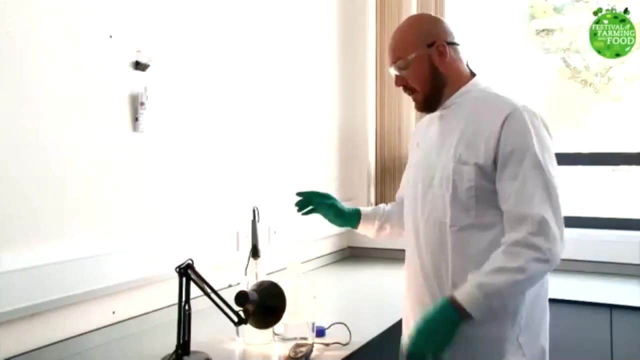 than our control. The lamp here actually represents the sun, which was both a light and heat source, And the two bottles represent our atmosphere under normal conditions and under exaggerated carbon dioxide conditions. Okay, so we've left the experiment overnight. It's actually got a bit cooler in here. 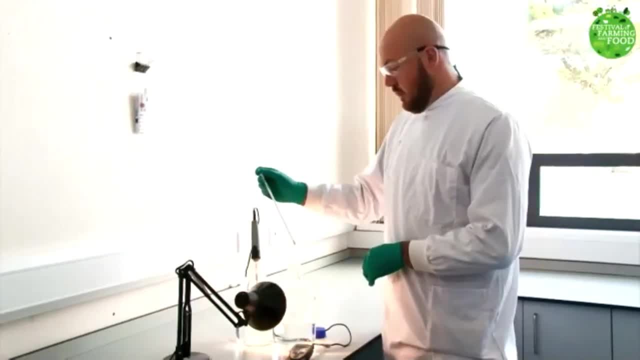 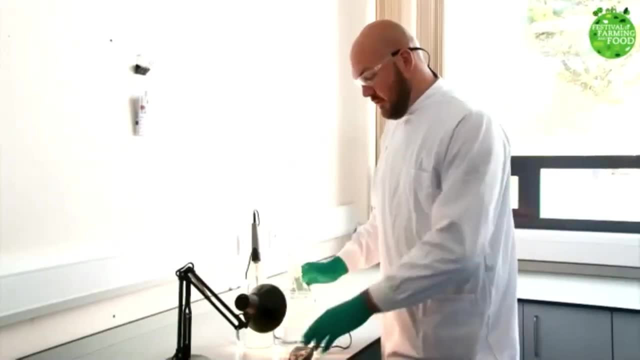 The heating's been off, obviously. So this is our control. We are now just about 17.5 degrees Celsius in our control, And if we look at our CO2 bottle, then we are up around 26.7 degrees or so. 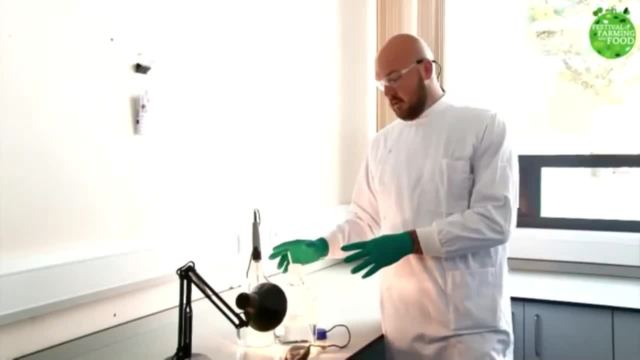 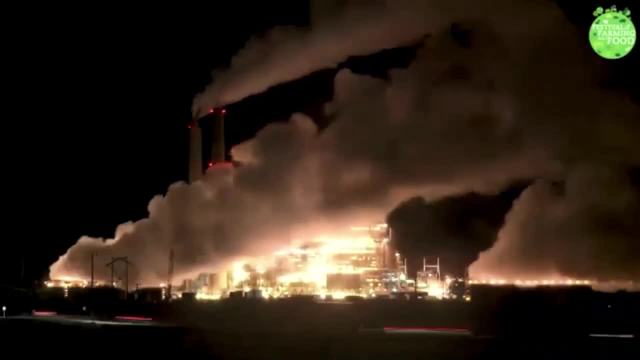 That just goes to show a temperature difference of 10 degrees Celsius, And that's just here in the lab in front of us. That's what's happening in our atmosphere at the minute, when we are emitting such amounts of carbon dioxide into the atmosphere. 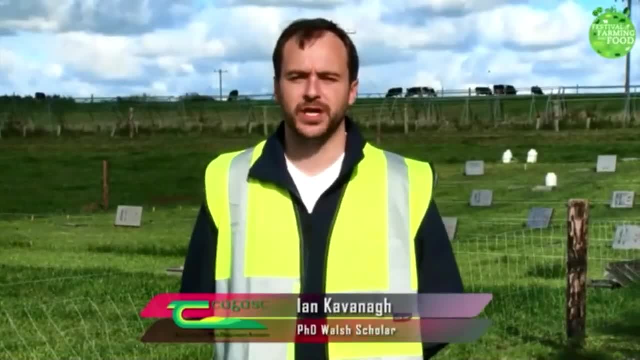 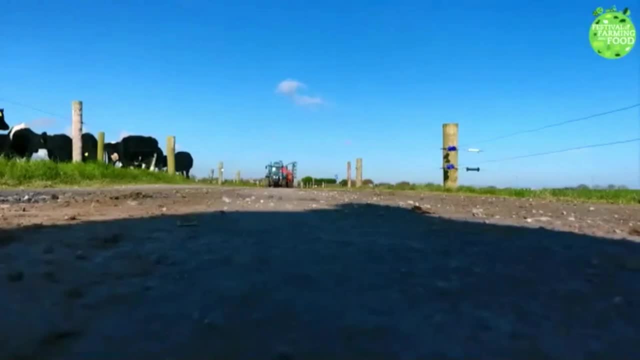 Hi, my name is Ian Cavanagh and I'm going to be talking to you today about the importance of soil and its role in nutrient recycling. Irish agriculture, be it animal or crop production, produces a lot of organic residues in the form of animal slurry. 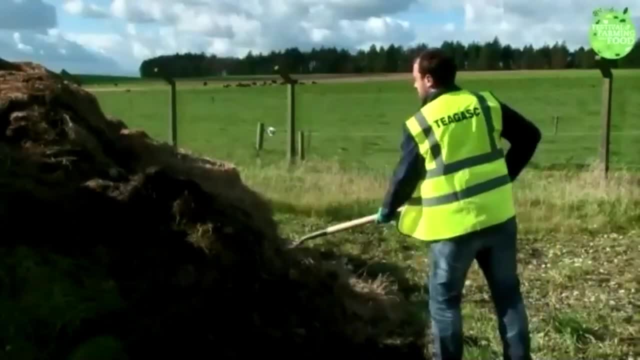 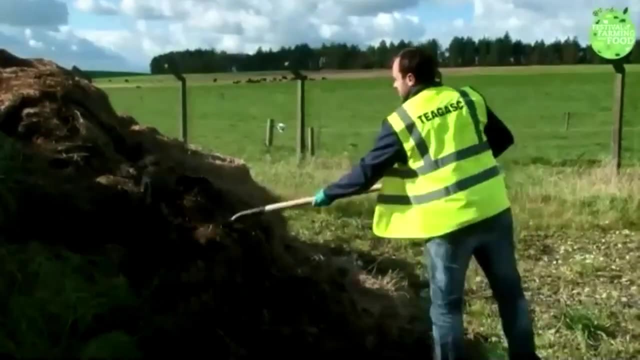 or incorporated into bedding to create farmyard manure. However, other byproducts such as food processing, waste management and industrial residues also have to be dealt with. The incorporation of these organic residues into the soil is one such method to reduce the organic residues. 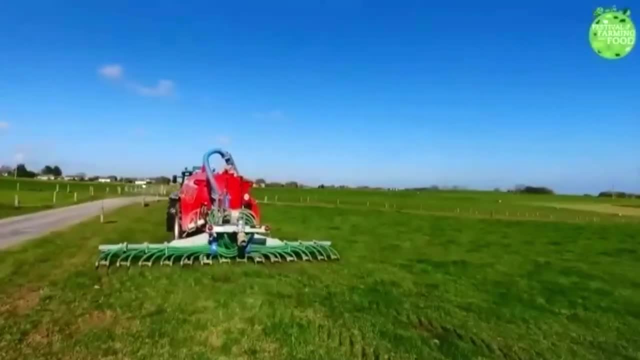 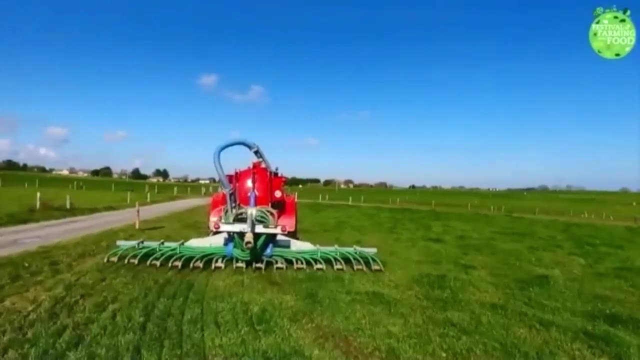 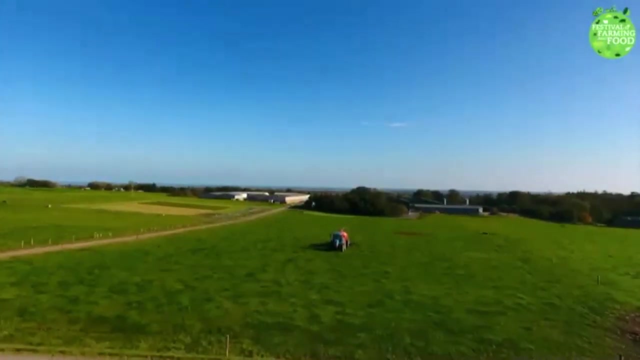 from animal farming and food production. These organic residues are a good source of organic matter, carbon and nutrients in the form of nitrogen, phosphorus and potassium. These feed soil biodiversity and help sustain healthy crop production. This is of vital importance, as this nutrient recycling helps close. 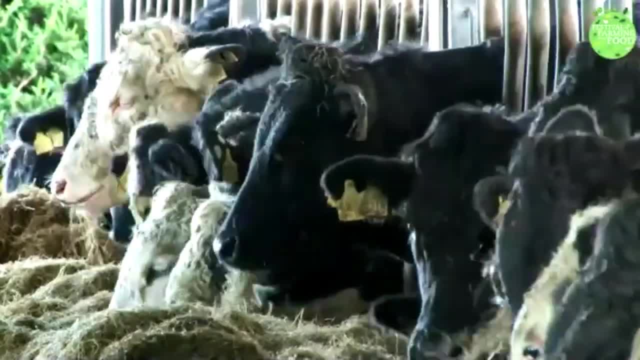 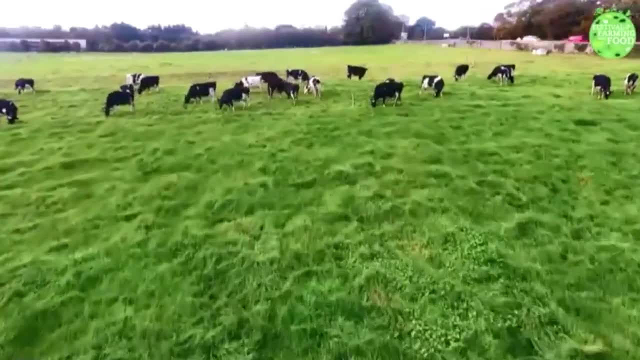 the carbon nitrogen and phosphorus loop and promote the farm-to-fork cycle, while also helping to reduce the use of artificial chemical fertilisers. With this in mind, Chagas is running a number of experiments and field trials to assess the impact of these residues. 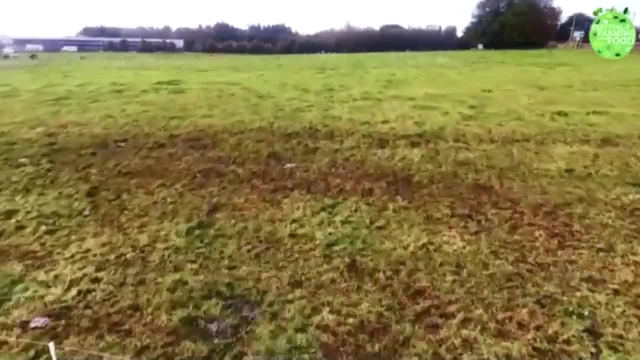 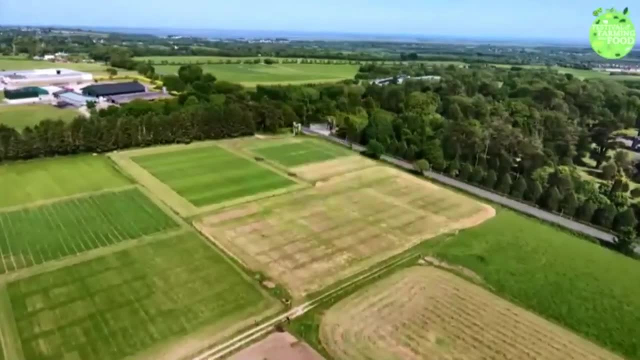 and the best way to utilise the nutrients available in the soil. Trials such as the EU-funded project Nitri2Cycle is investigating new bio-based fertilisers for their efficacy in grassland and arable crops. They also examine their benefits to soil health, such as 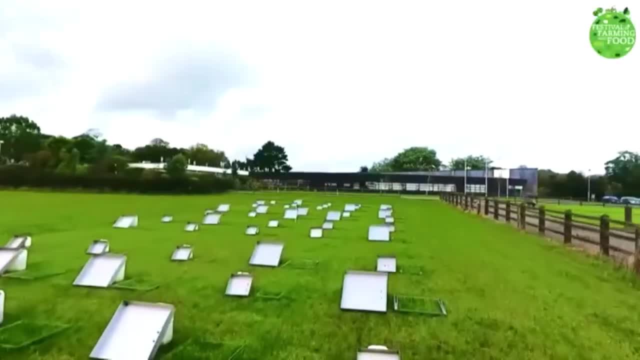 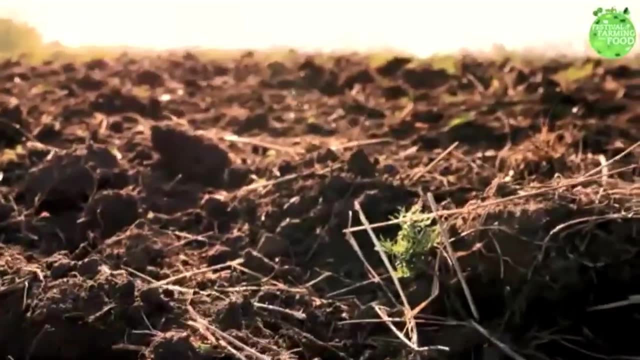 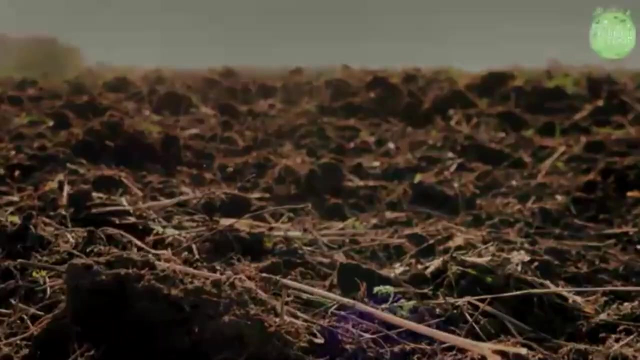 increasing soil organic carbon. Other field experiments have also looked at acidified and amended cattle slurry and its utilisation and incorporation into the soil. However, none of these residues would be advisable if it wasn't for the wide variety of microorganisms that call the soil home. 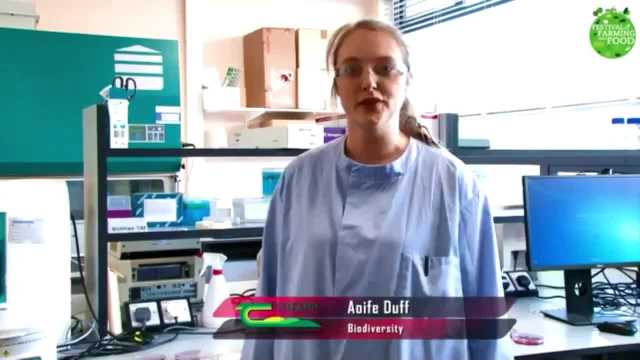 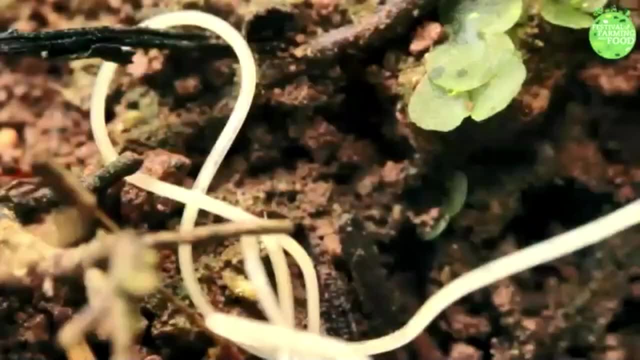 Hi, my name is Aoife Duff. I'm a soil microbiologist here in Chagas and today I'd like to talk to you about soil biodiversity and how it contributes to soil health. As you've already heard, carbon sequestration, nutrient cycling, 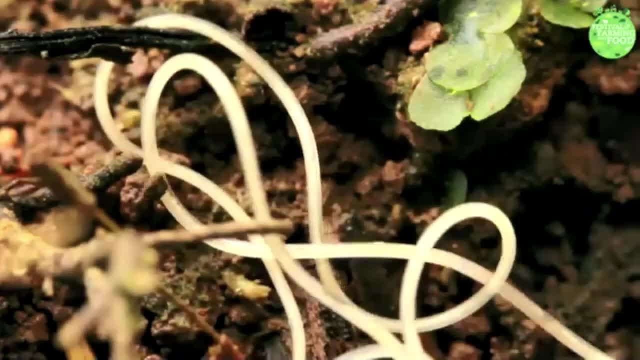 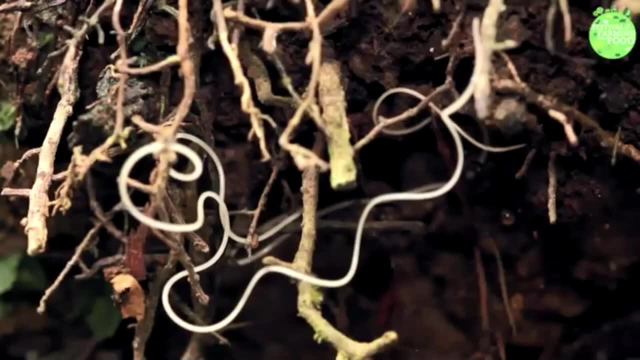 and all of the processes mentioned so far are very important for soil health. But what makes these processes happen in the soil? Well, some of the processes take place via chemical reactions and the majority of the processes are driven by what we call microorganisms. 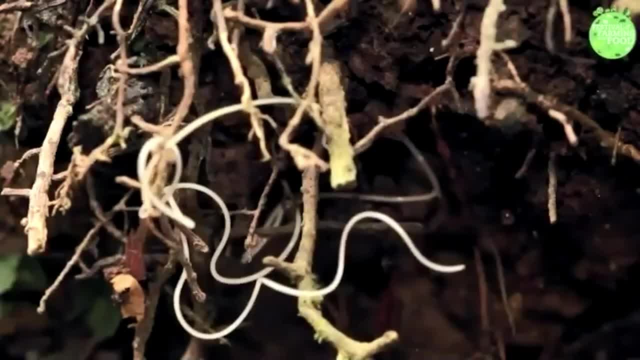 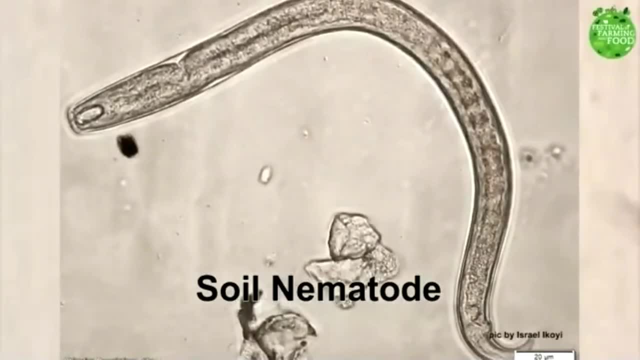 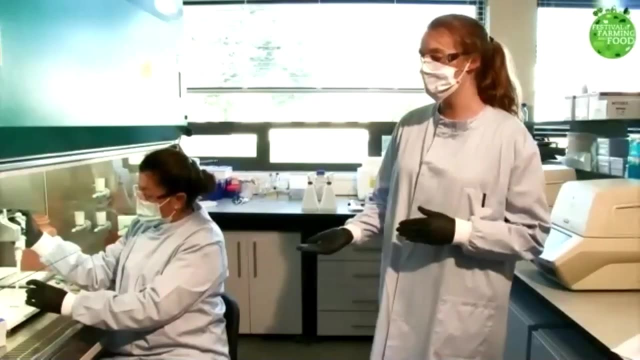 In fact, in one teaspoon of soil you can find millions of species of microbes and together it contains billions of microorganisms. So essentially, the soil is teeming with life. So here in Chagas we are doing lots of projects to work on soil biodiversity. 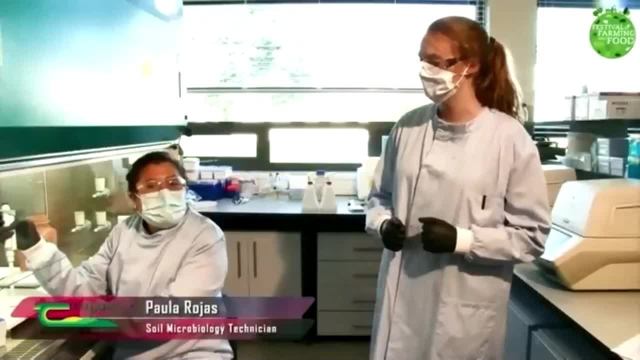 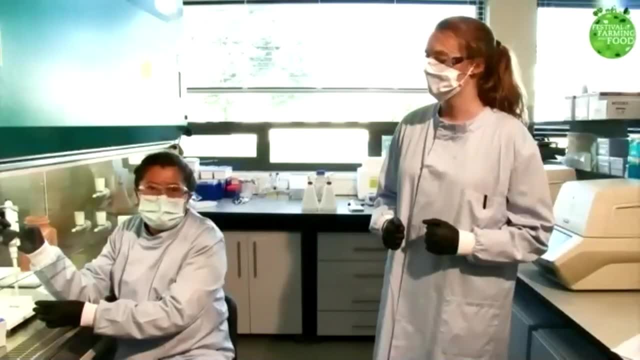 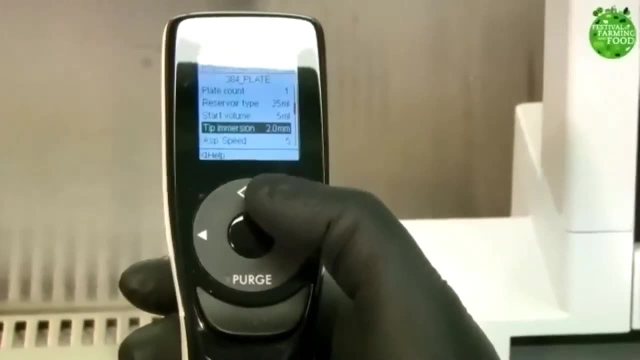 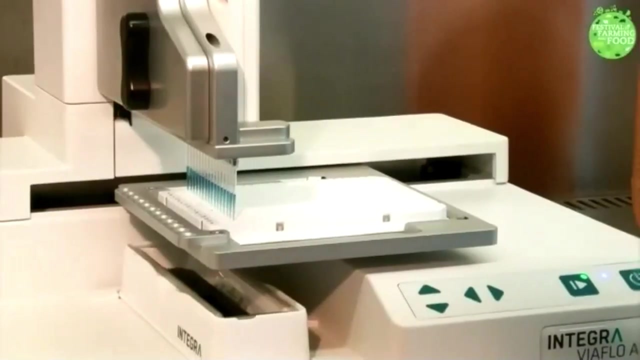 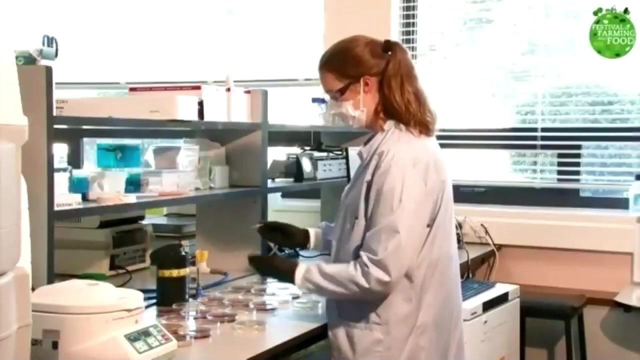 Paola Roja is our technician. What are you working on, Paola? I'm working on how the soil microbial community can divert the agricultural greenhouse gas emissions coming from the soil. You may ask me: how can you tell how many microorganisms? 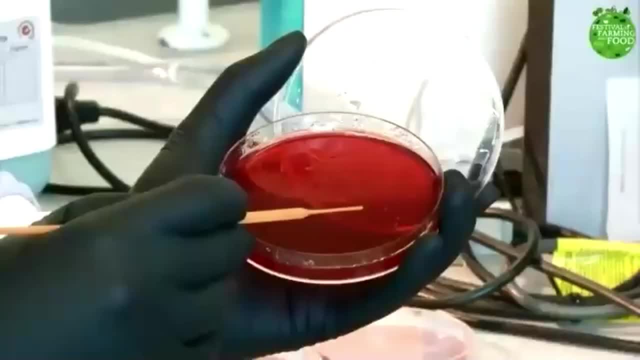 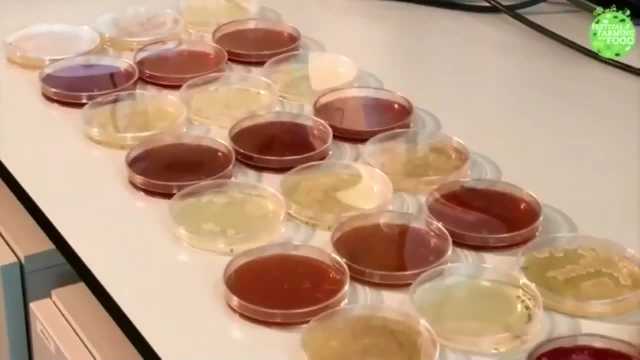 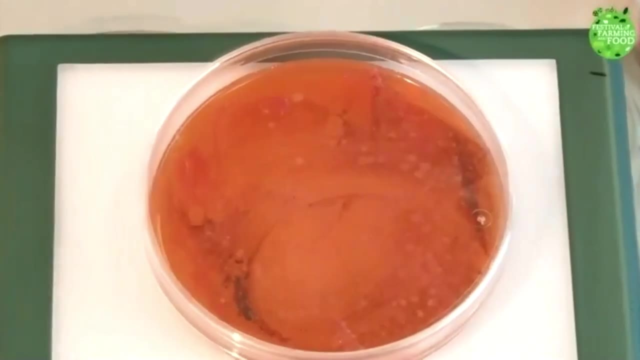 are in the soil. Well, not too long ago, I was working on a project with a group of scientists and discovering what they did was to grow them on lab media. Media is a combination of different elements, like carbon and nitrogen, which the microbes require in order to grow. 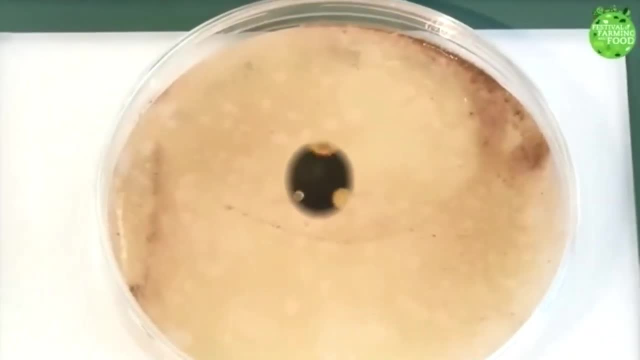 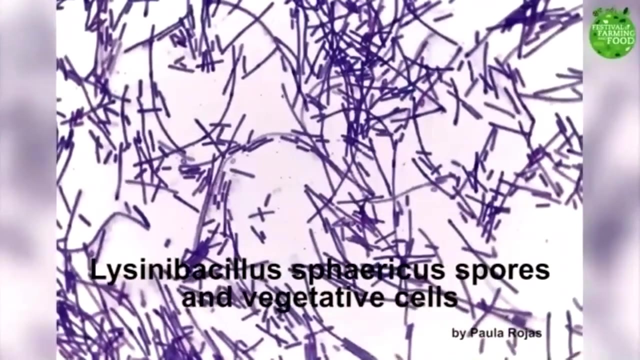 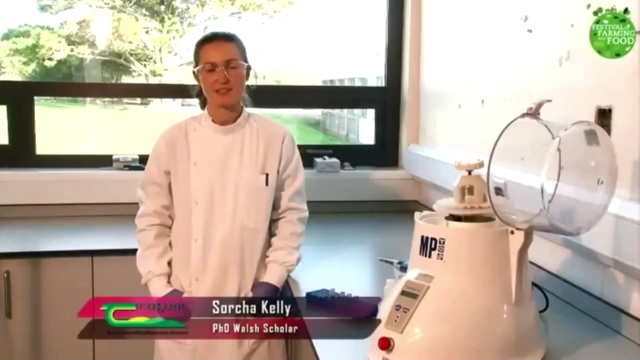 The problem with this method was all microbes may not eat the exact same food or elements, and so the scientists discovered they were only growing about 1% of the microbes present in the soil. Microbiologists started to find a way to do this. Hi, my name is Sirka Kelly. 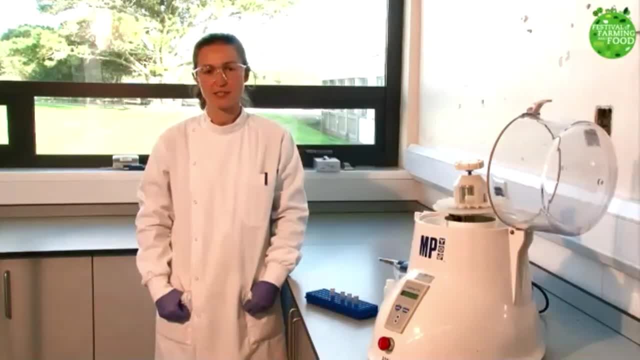 I'm a PhD student here in Chagas, Johnstone Castle. My project looks at how soil microorganisms make nutrients available from soil organic matter in order to help plants to grow. Today, I'm going to show you how we extract microbial DNA from soil. 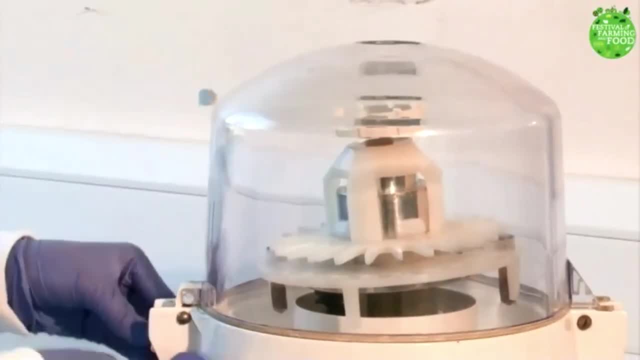 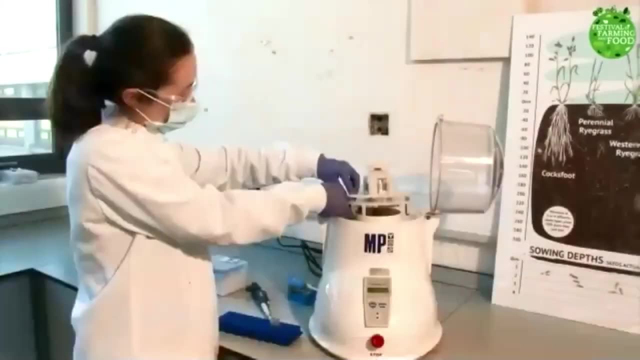 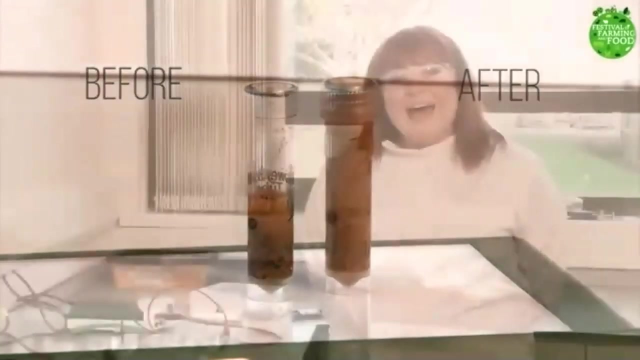 Sirka Kelly is demonstrating a DNA extraction Here. she uses a fast prep machine to vortex or shake the beads in the tube and chemically and mechanically extract the DNA. Hi, my name is Kerry Ryan. I am a PhD student and I study microbes in the soil. 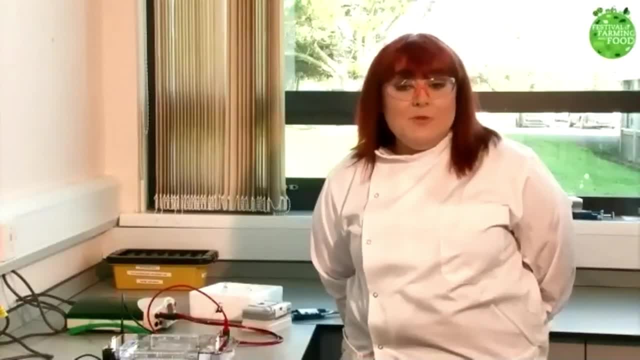 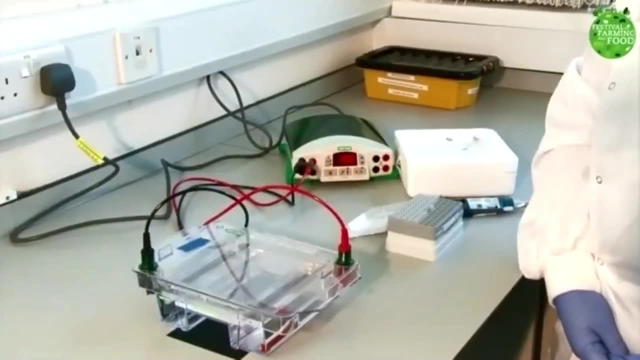 I'm particularly interested in how mixed species grasslands affect, what kind of microbes we find in the soil, how they work and how they are affected by drought. Today we're going to look at how DNA can be separated through gel electrophoresis. 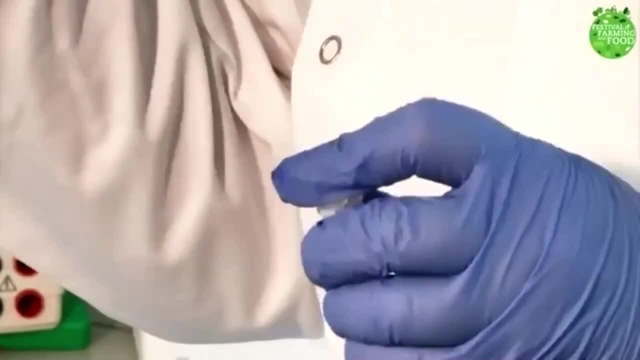 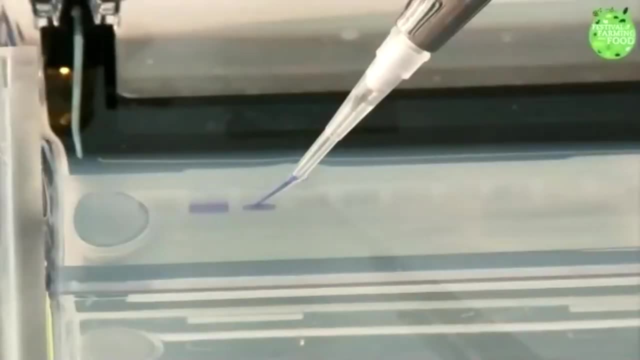 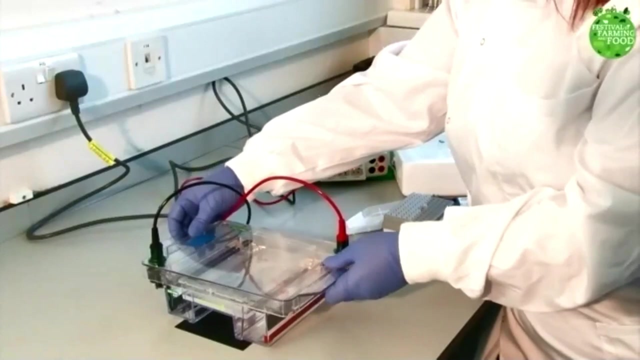 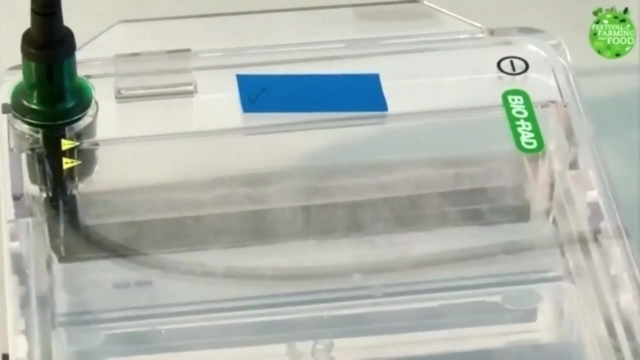 So that we can visualise the DNA. Finally, with a combination of different techniques and sequencing technology, we were able to read their genetic code, which told us all of the genetic information of each species of microbe. So this is just a taster of the world of microbiology. 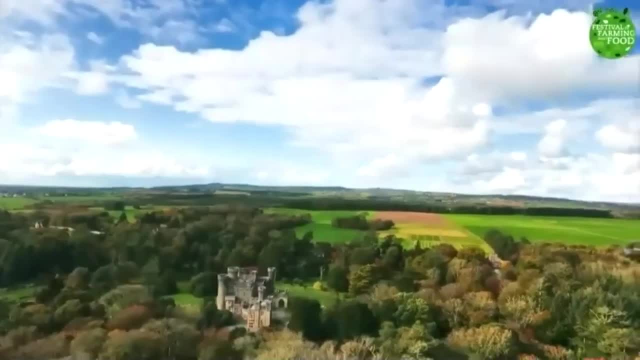 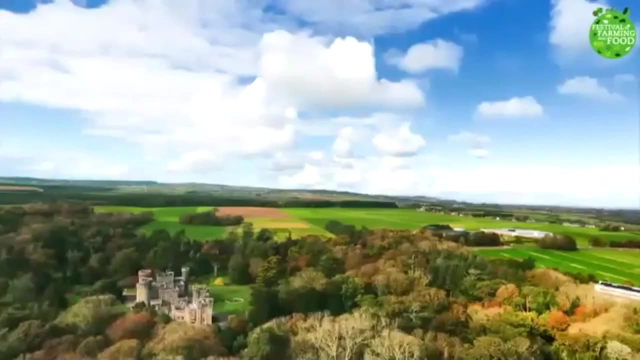 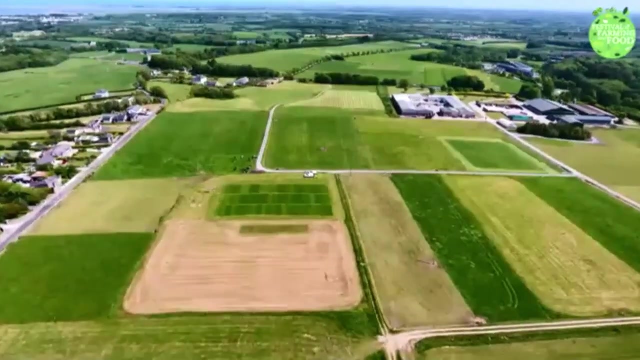 and soil biodiversity in Cagasc. We hope that our projects will help farmers employ the best management techniques possible to keep the soil biodiversity balanced. This, in turn, will keep the soils healthy in order to carry out vital functions that will help the farmer and the environment. 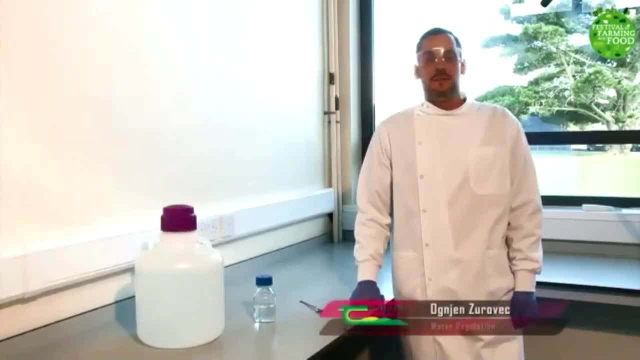 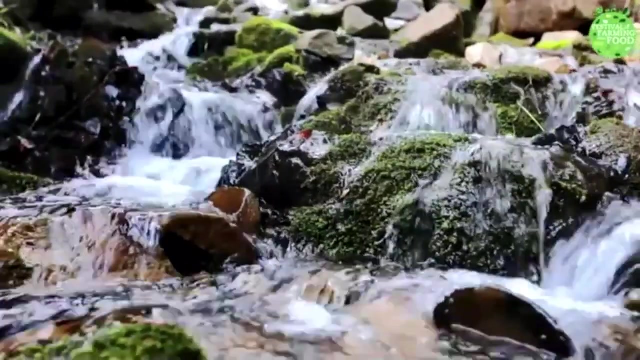 Hi, my name is and I'm a soil scientist in the agriculture, and I'm going to talk about the soil management program. So, as you have heard by now, soil has many different functions. One of them is the provision and supply of clean water. 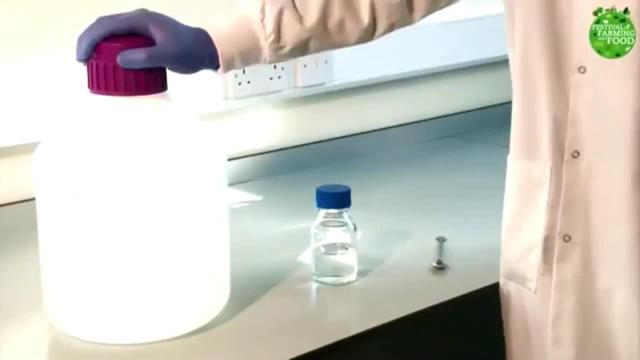 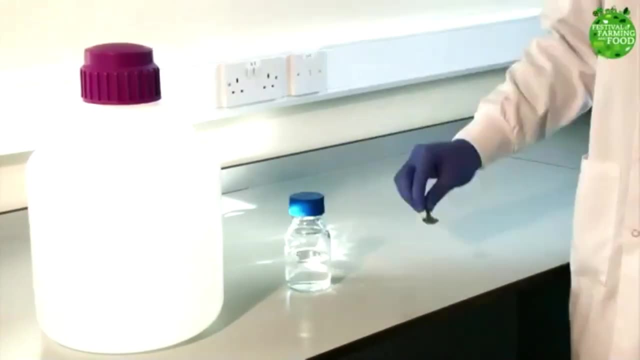 Only 3% of earth's water is fresh water And we can only access and use a tiny fraction of that fresh water. Imagine that this tank contains all the water on earth And this little bottle would be all the fresh water on earth. 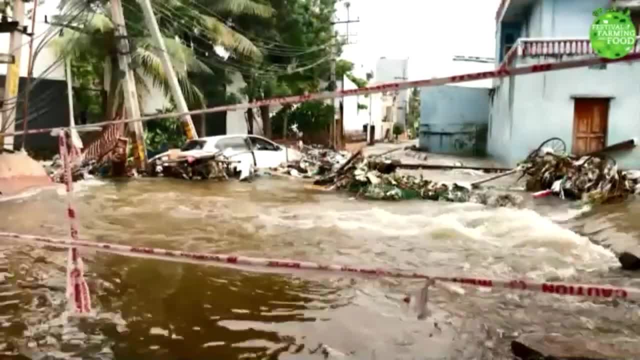 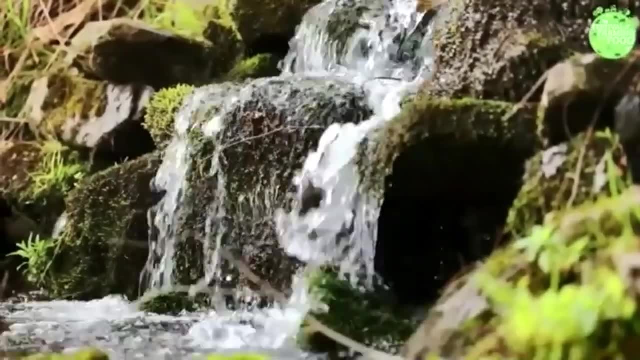 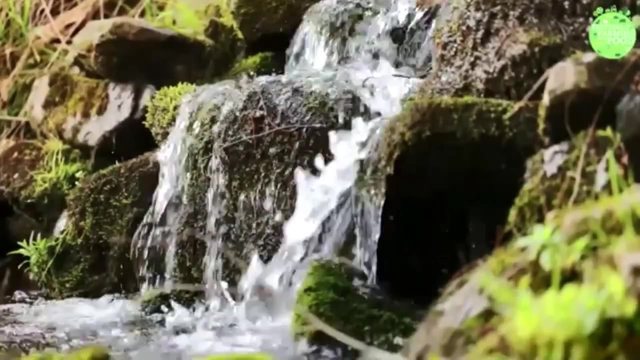 And then this tiny little teaspoon of fresh water is shrinking every day as a consequence of things like climate change and water pollution. Fresh water supply is continually collected, purified and distributed in the natural water cycle with the help of soils. Soils are earth's largest natural filter. 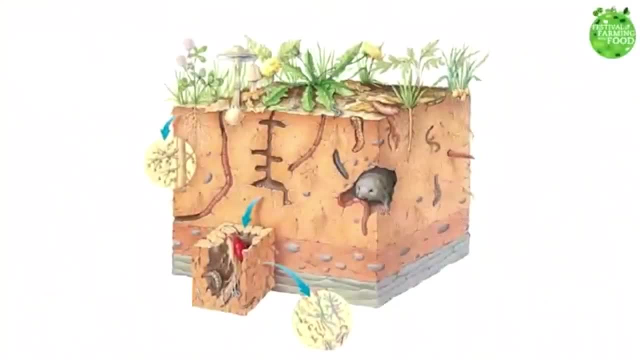 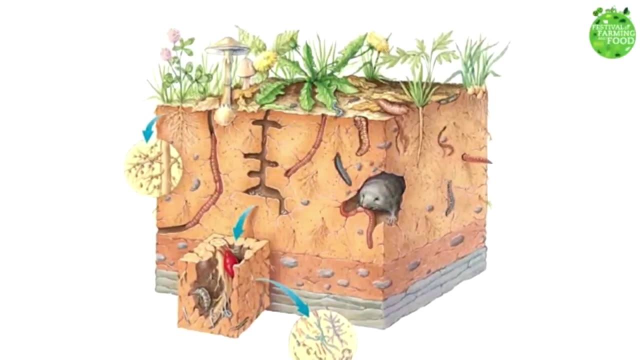 and capturing water is one of the most important roles that soils play in our ecosystem. Soils capture water through their pores. Pores can be any size, from small microscopic holes to large worm-like holes and mice tunnels. Soils capture water through their pores. 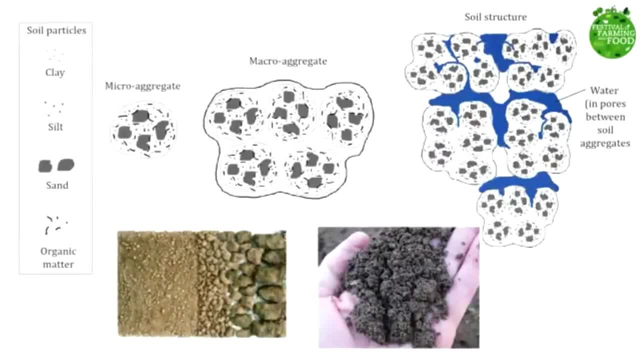 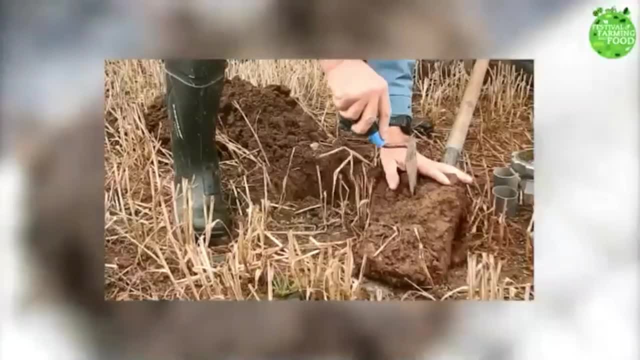 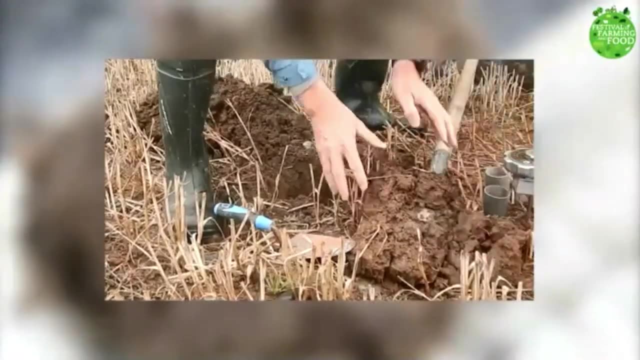 with the help of soil structure, which is a ratio of different soil particles, such as sand, silt and clay. These particles stick together with the help of biological life and organic matter, which provide the glues to form tiny crumbs called aggregates. Aggregates are the building blocks. 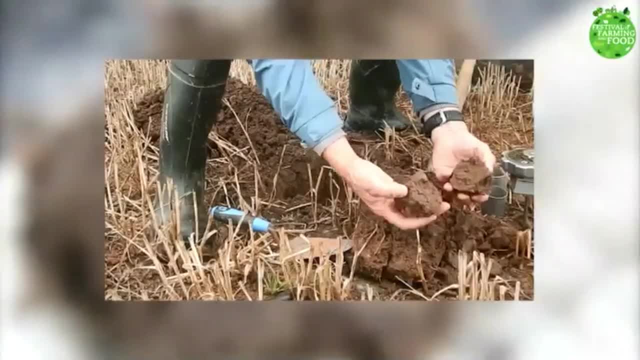 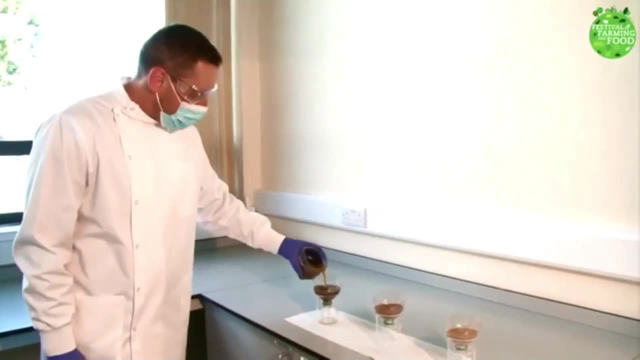 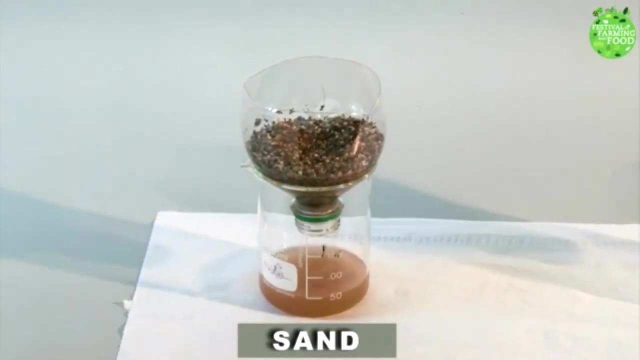 of every soil and they contain lots of pores and cracks. Aggregates form soil structure, which increases the ability of soil to capture and hold water. Sandy soils have many large pores. While they are good at capturing water, water moves quickly through them. This does not allow soil enough time. 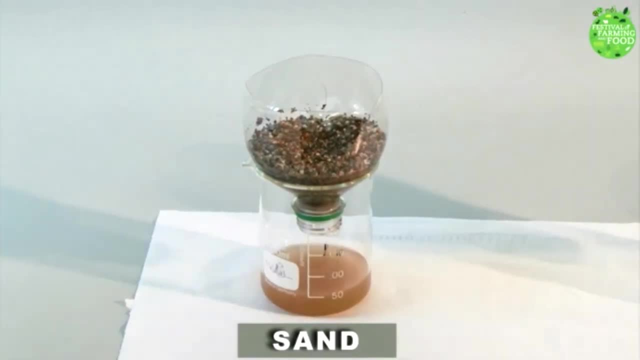 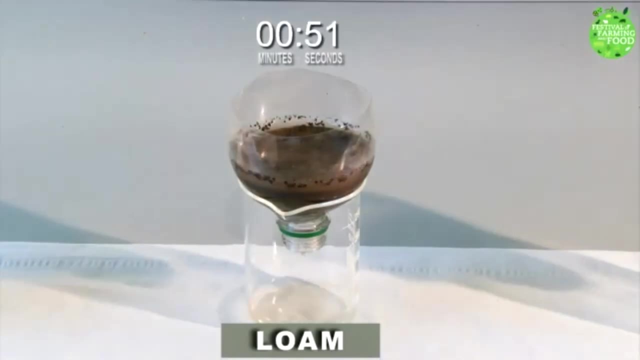 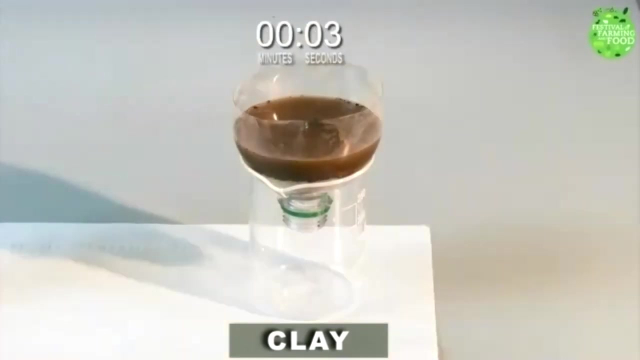 to fully purify on its way downwards to groundwater. Loamy soils have both large and small pores. While water moves through them quickly, some of that water is also filtered. Clay soils are sticky and have lots of small pores. They are very good at purifying. 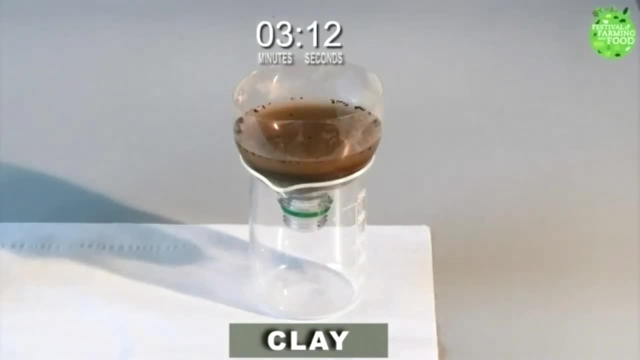 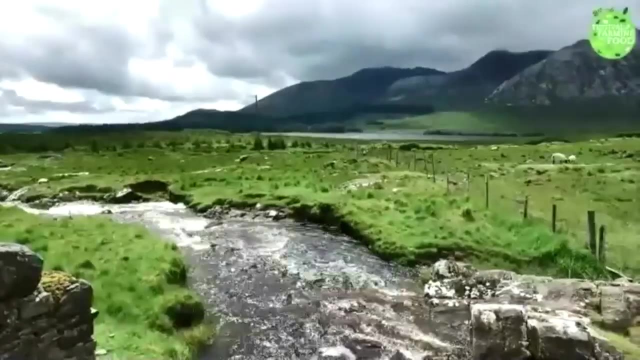 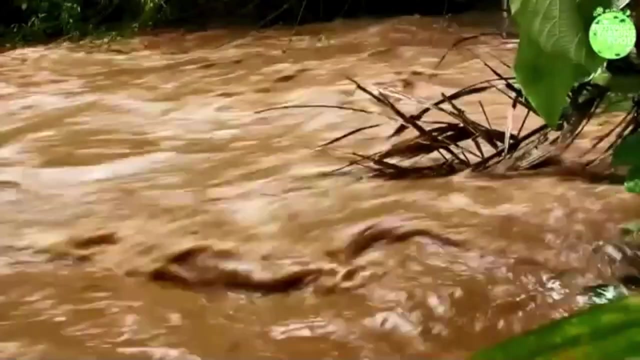 and holding water, but they are slow to capture water. Water that is not captured by soil runs off the soil surface until it reaches a nearby source of surface water, such as stream, river or lake. This water can also cause floods during heavy rainfall events. 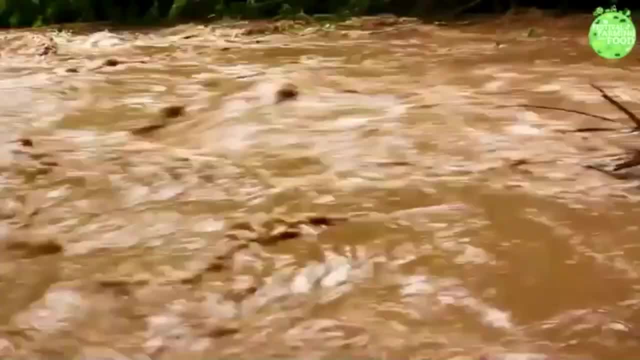 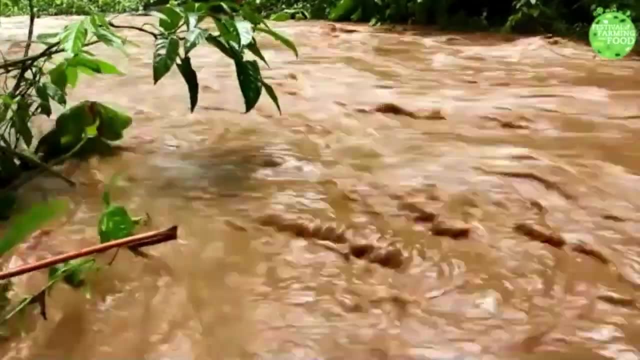 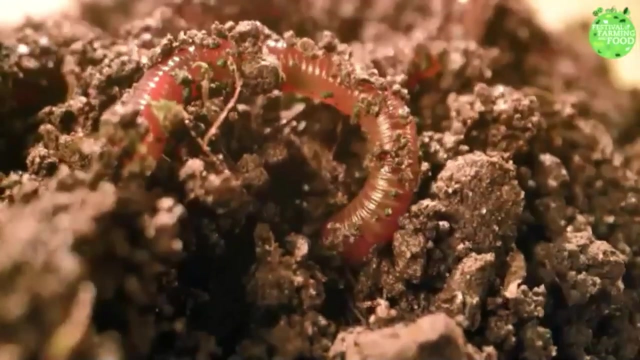 The run of water also picks up soil particles with all the nutrients and chemicals attached to them, transporting and depositing them into receiving waters. This has a very harmful effect on aquatic plants and animals. Healthy soils are full of life and organic matter content. Because of that, they have lots of 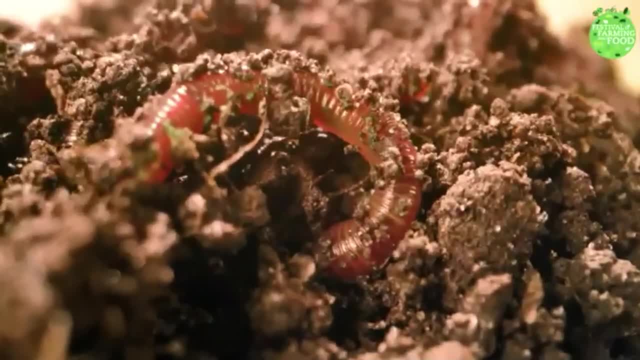 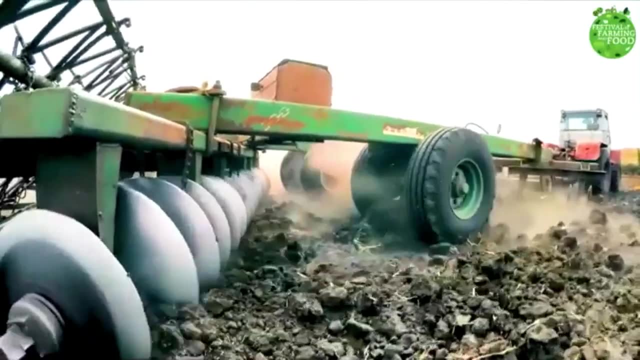 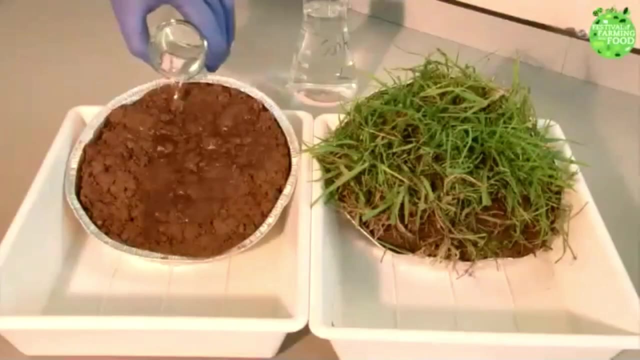 big and small pores. Therefore, it is important to minimize the disturbance of soils. Frequent tillage or compaction by heavy machinery destroys soil structure. These soils will only have small pores. Land surface cover is also important. Healthy soils covered by plants are most efficient at capturing water. 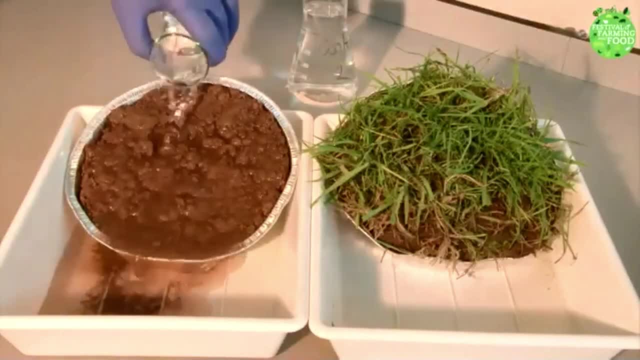 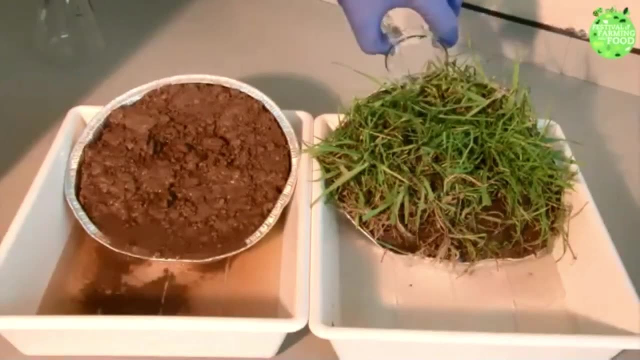 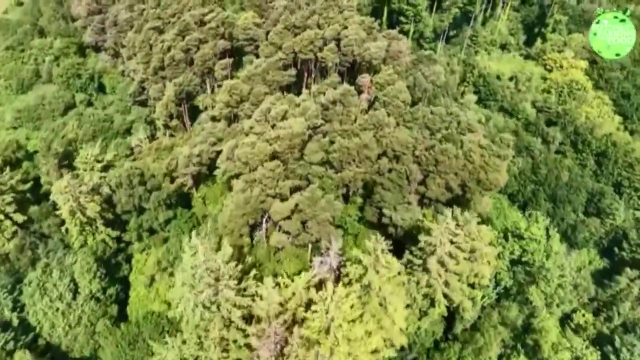 Plant roots keep the soil together. Dead roots provide soil organic matter and together they make the soil resistant to erosion. The above ground biomass, like trees and plants, reduces the devastating impact of rain and slows down the flow of runoff water. It is also important not to fertilize. 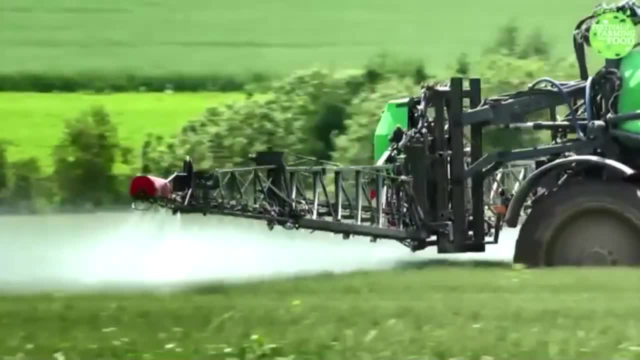 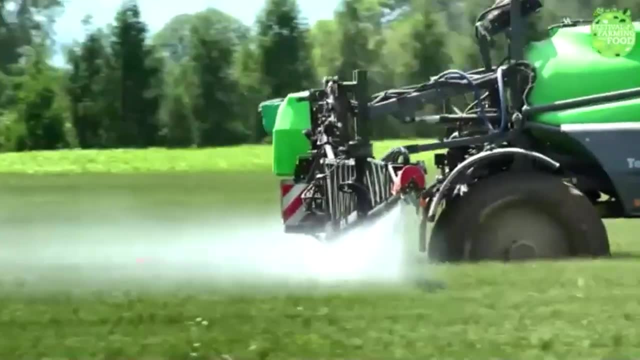 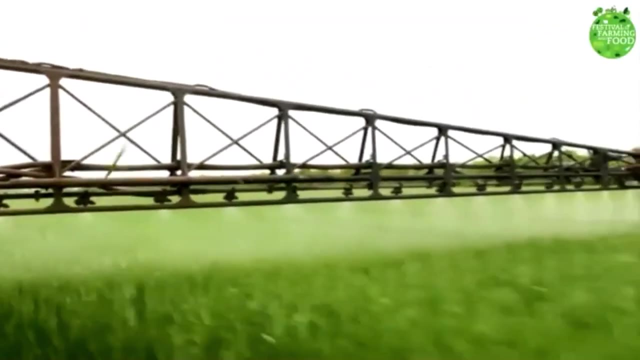 soils more than is needed by plants, especially with nitrogen and phosphorus fertilizers, or to spray them too much with chemicals such as pesticides and herbicides. This is because excess fertilizer and chemicals can enter and contaminate the groundwater or can be washed off the surface. 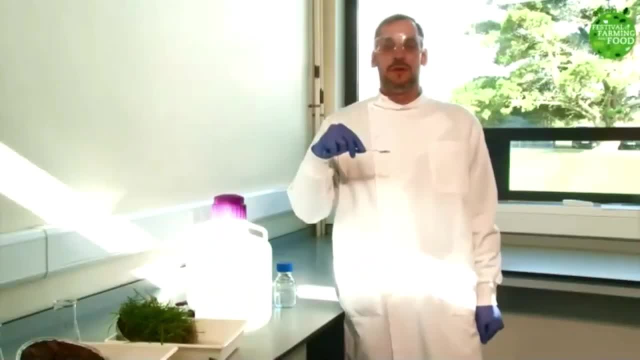 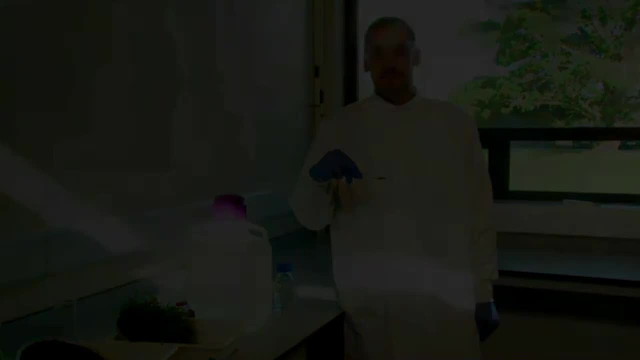 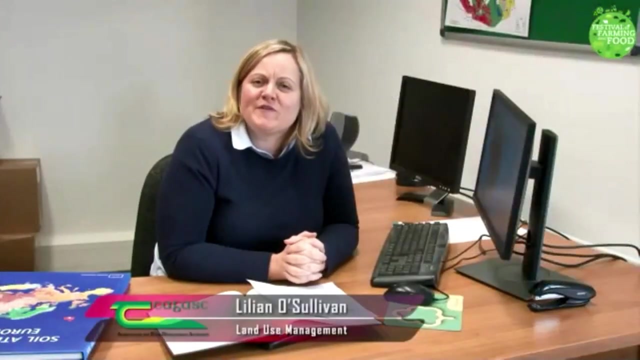 of rivers, lakes and seas. Remember this teaspoon of water. So how do we prevent it from shrinking in the future? One of the answers is to keep our soils healthy. Hello, my name is Lillian O'Sullivan. I'm a research officer. 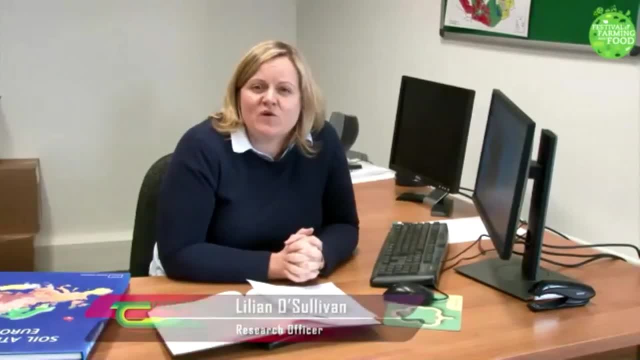 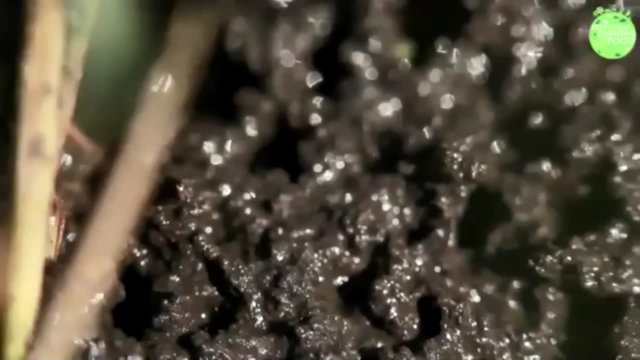 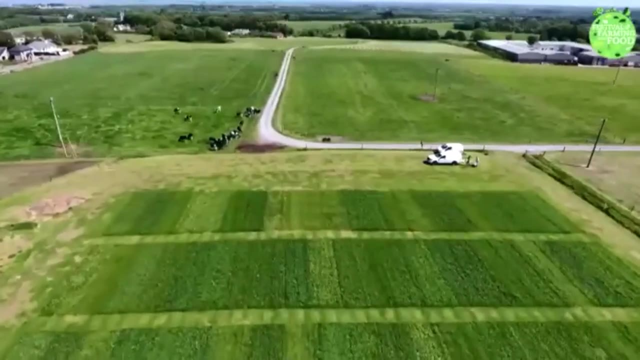 here in Chagask, where my work focuses on sustainable soils and land use. So now you have seen an overview of the different soil functions. we know that soil functions are critical to sustain life on earth, and my work focuses more specifically on how these soil functions work together. 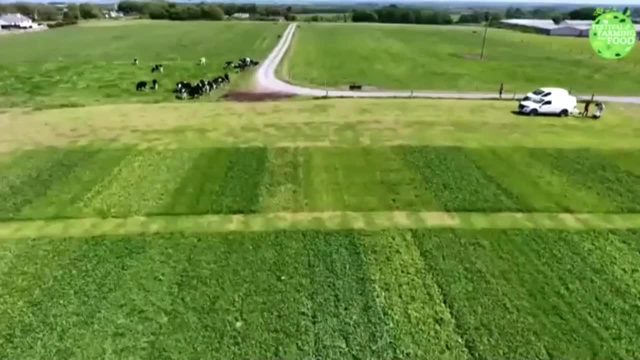 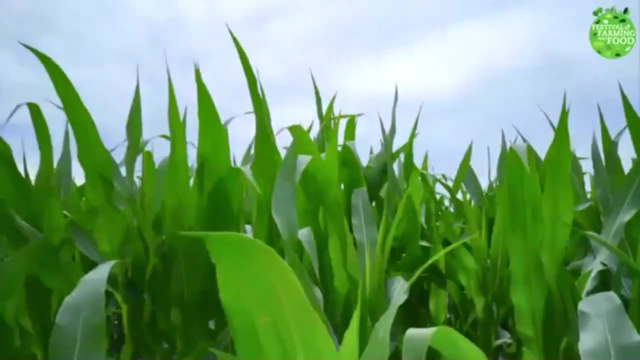 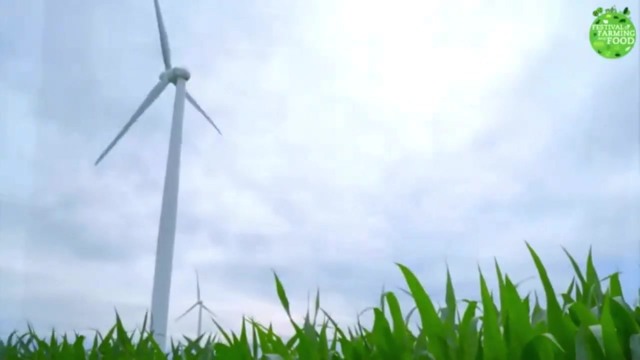 at larger scales. It is important that we manage the system sustainably to maintain soil health, to guarantee the delivery of these critical soil functions into the future. So how can we support this? through our research Process, knowledge can explain how each soil function works and each soil function is. 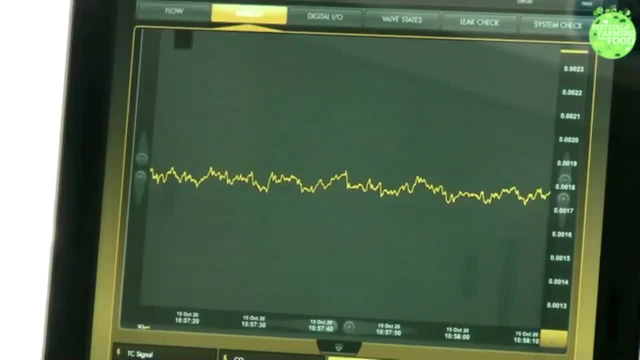 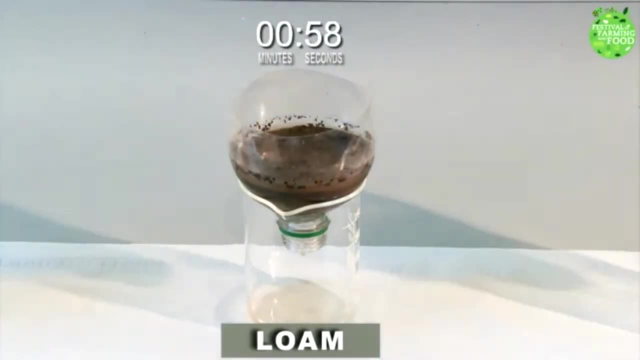 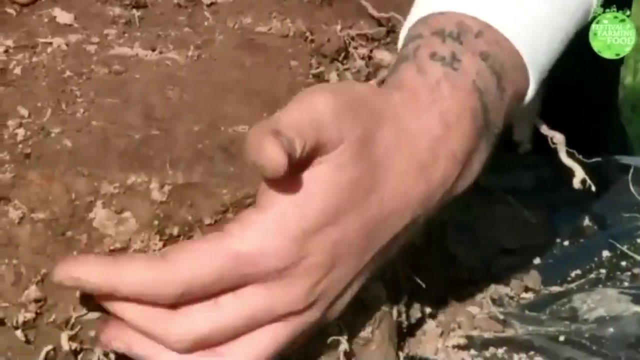 a very complex process in its own right, For example, the process of cleaning and purifying water as it moves through the soil matrix, as Auggie showed you earlier, or how the soil accumulates and stores organic matter, which is really important for climate regulation. 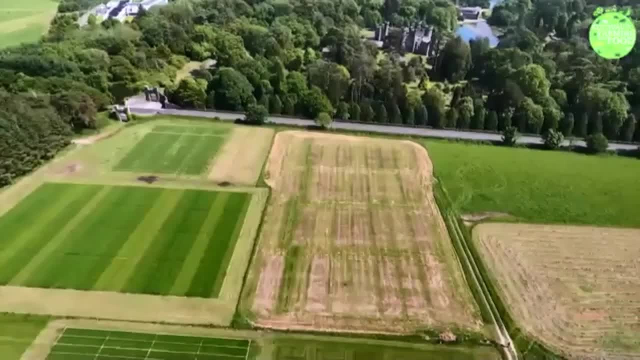 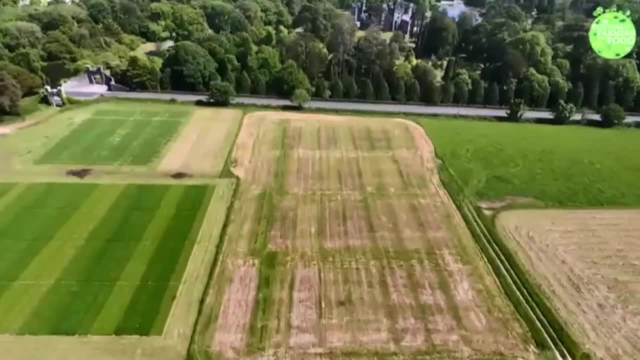 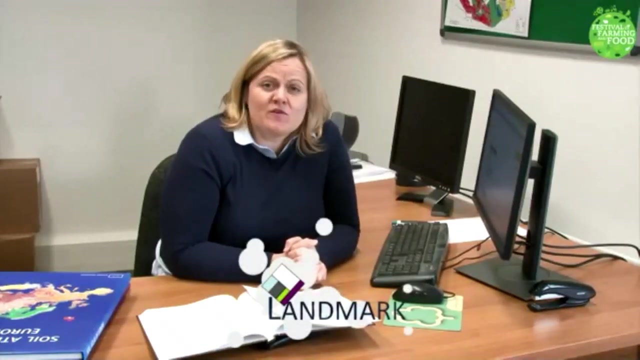 as shown by James. Understanding these processes helps us understand how much a particular soil, in its environment, interacting with management, can deliver a soil function. Recently, as part of an EU funded project, landmark, we developed the Soil Navigator, which is a decision support tool that can help farmers and advisors. 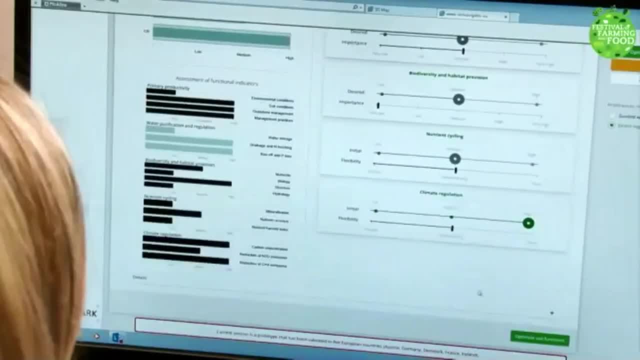 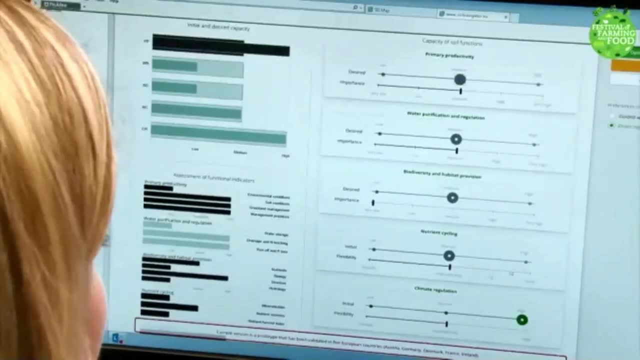 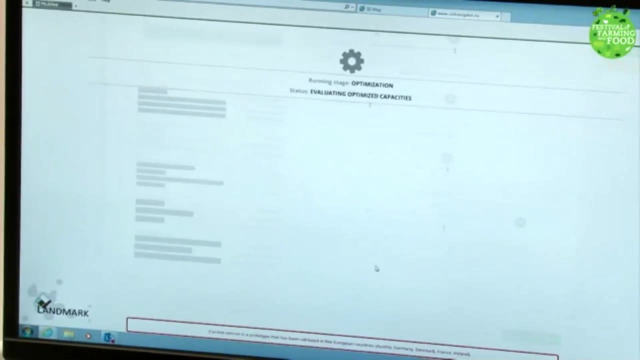 optimise their soil functions together. So, essentially, you input some data and you ask it to assess your soil functions and it allows you to optimise based upon your requirements. So if I have an issue with water quality, I will ask the Soil Navigator to optimise in favour. 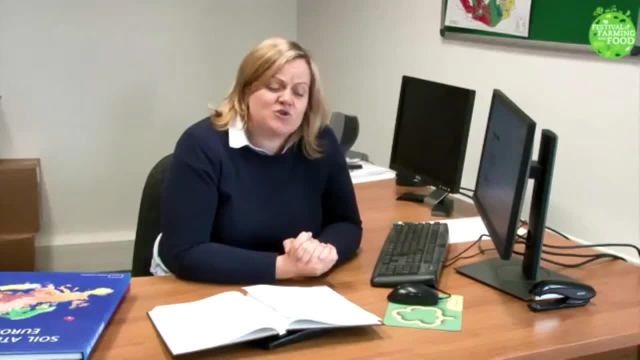 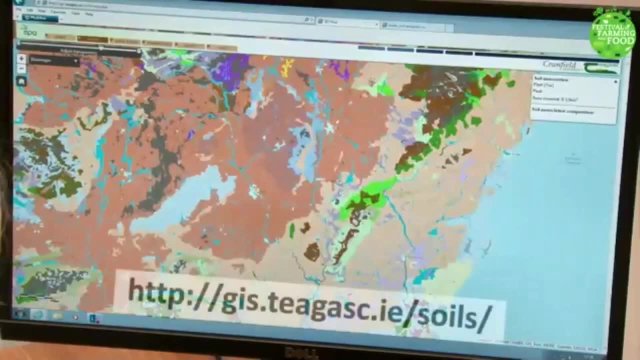 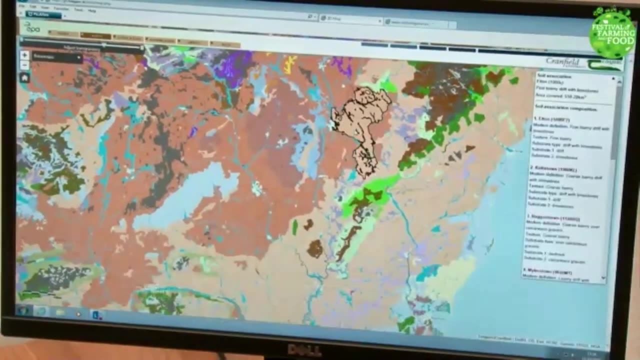 of that soil function. One resource I often use is our Irish Soil Information System. It's a fully interactive map. anybody can go online and learn more about the extent and distribution of the different soil types that we have, or in your own area Here in Johnstown Castle. 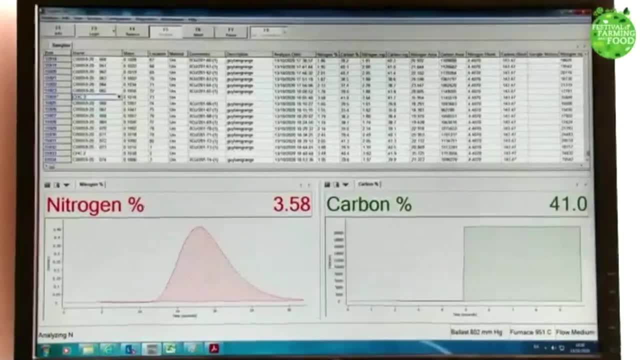 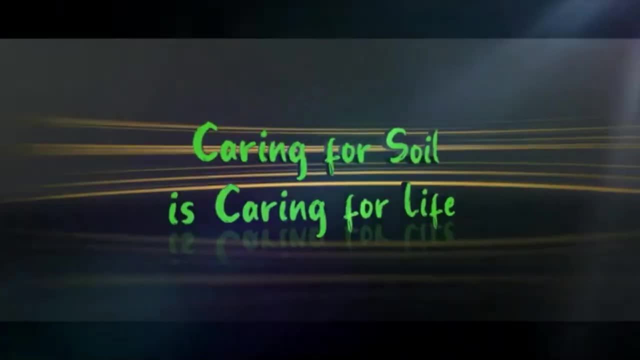 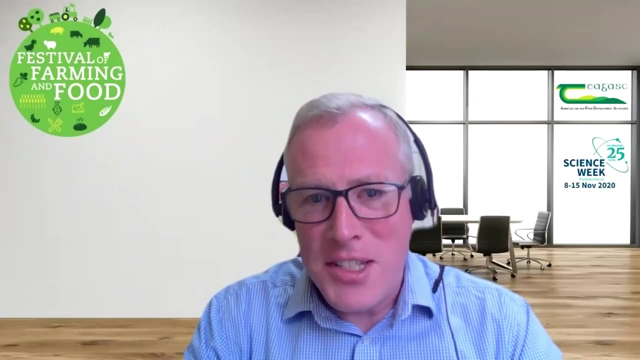 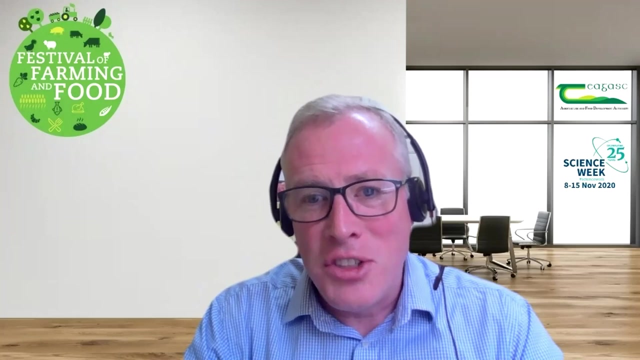 we aim to generate science that can support sustainable land management And remember caring for soils is caring for life. Well, that was really a fascinating take on what's going on there in Johnstown, and thanks to all the staff there for their courtesy in showing us what is going on there. 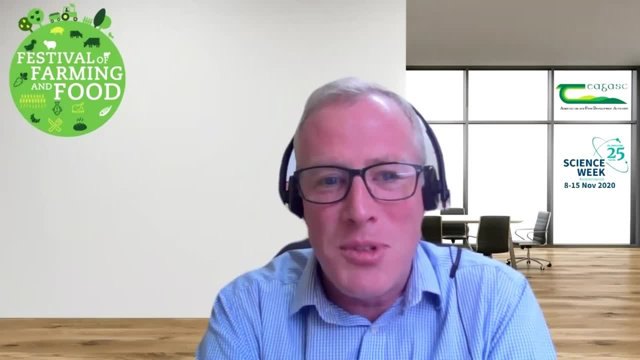 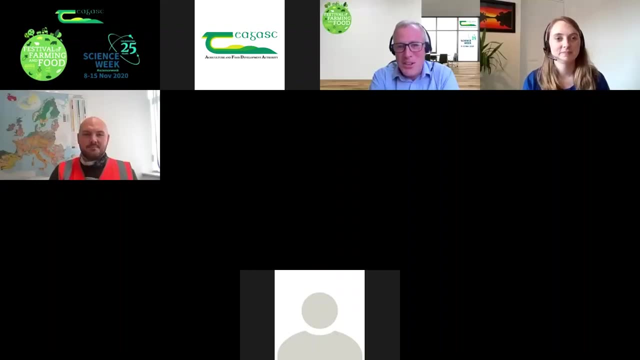 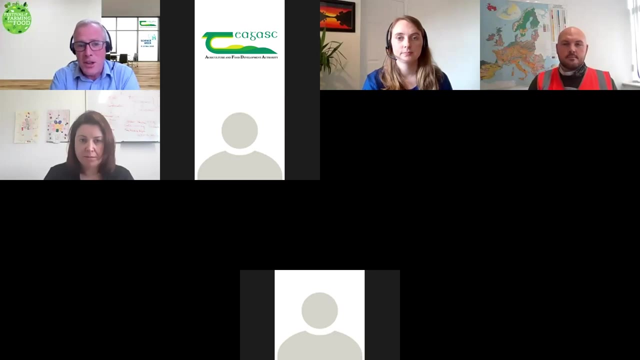 and what's happening in the area. So thank you very much for joining us. I'm sure you all are now joining us, so you can switch on your cams, guys, now that you have the make-up on and all of that, Good morning to you all. 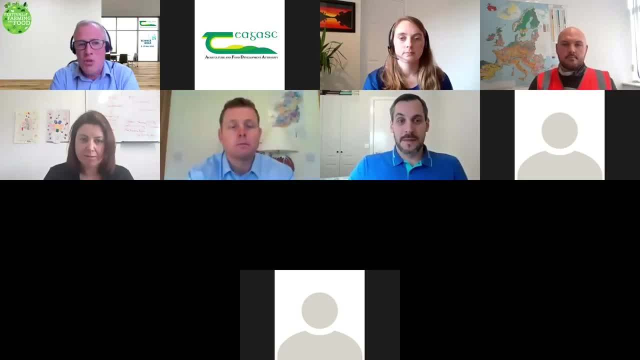 and we're going to chat to you now and remember for the participants, many of you that are out there all over the country and indeed across the world. we do know that we have some international observers at our webinar today, So we're going to do our best. 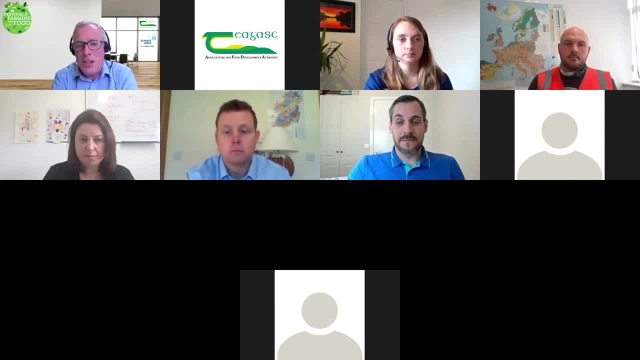 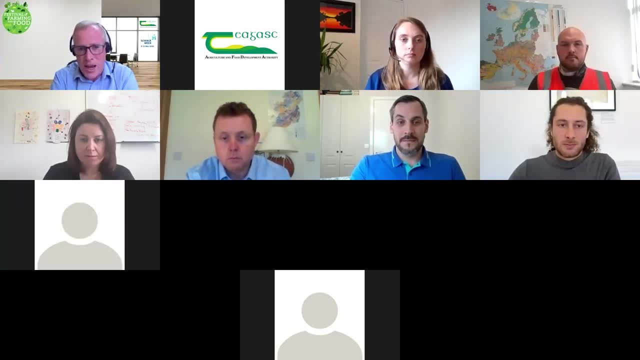 to try and respond to you individually or indeed in the actual chat. So we're going to have a little chat now, as I said, with some of the people involved there, some of the students and staff there at Johnstown, And we have with us Aoife Duff, who is a soils technologist. 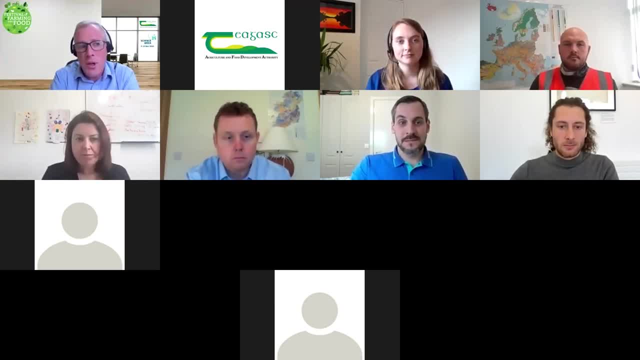 who works in soil microbiology- and you saw Aoife on the video there. We also have Luis Lopez-Sangil, who is a soils research technologist, who is also there. We also have a Chagas-Gouache scholar and a PhD student. 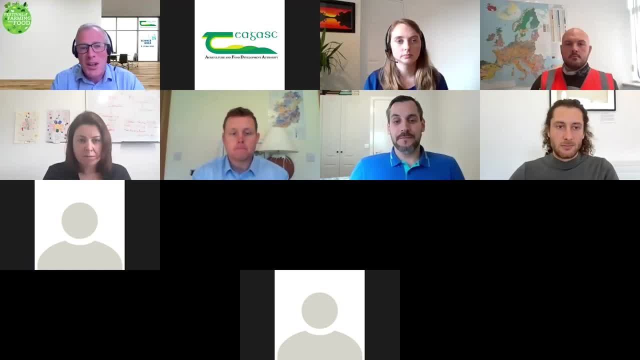 We have Oggy Zurovich, who is a soils scientist, and James Rambeau, who is a soil carbon sequestration technician. It's really like, with all those names, it's like a meeting at the UN there, guys, this morning, But it's great to have you all. 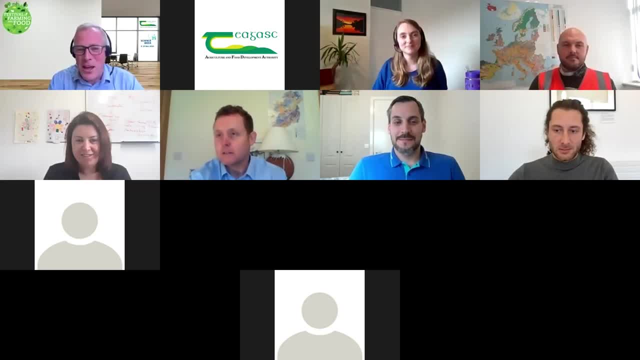 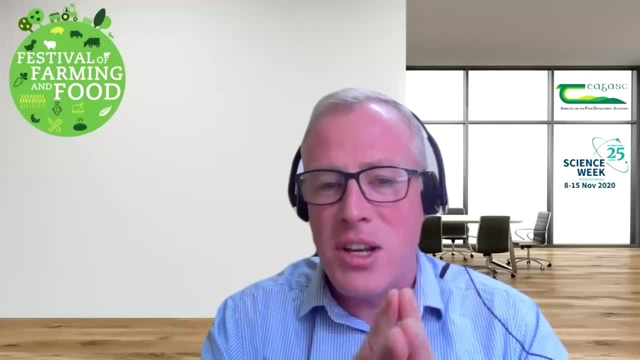 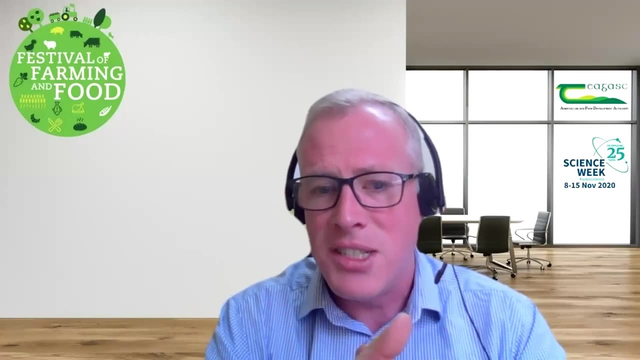 Aoife, can I begin with you? How are you? Good thanks, How are you? I'm really interested. Some amazing facts outlined and it's really wonderful work, and very important work in this time of climate chaos, that you're doing down there. 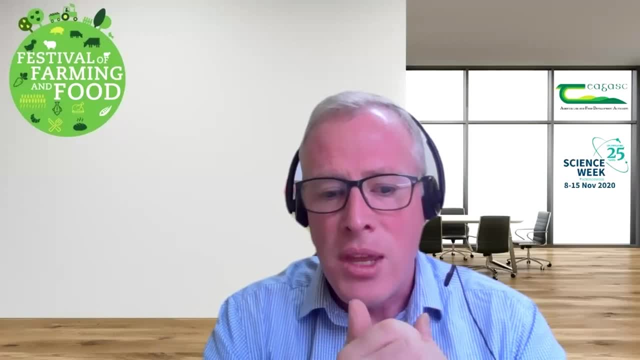 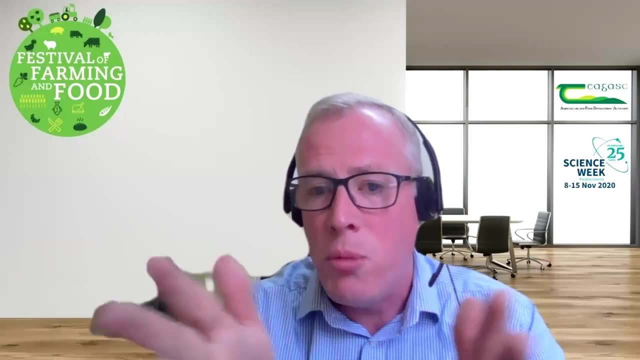 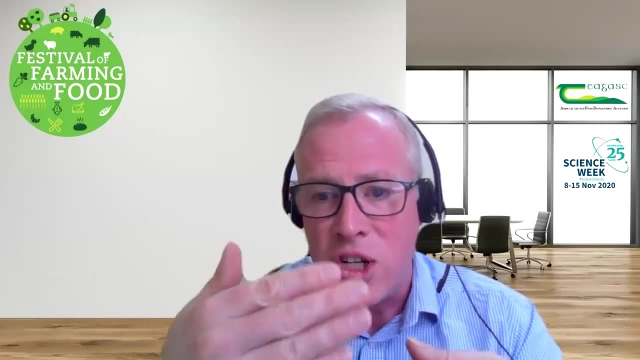 in Johnstown, But I'm just looking at the role of scientists and farmers in working towards a more healthy soil microbiome. How can we ensure that we can maybe do a bit more sequestration and have a more healthy soil microbiome? Yeah, so. 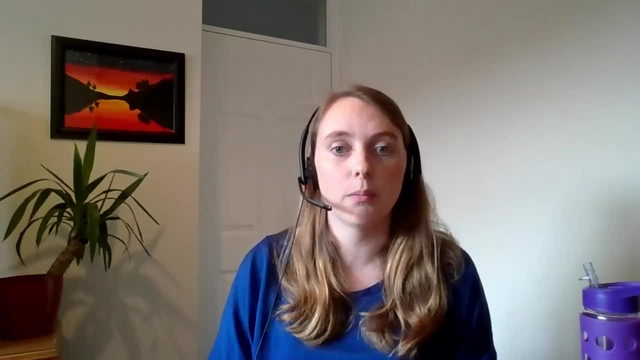 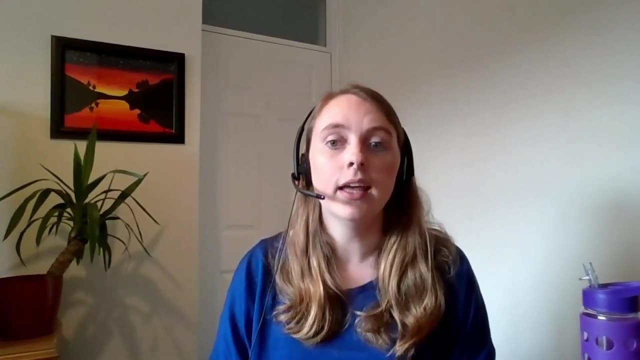 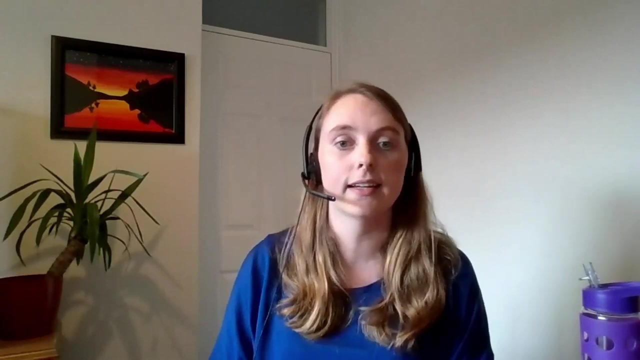 essentially that's what we were trying to find out in Chagas. We want to investigate microbes under different environmental factors and see how they respond, But so far we've found that compaction, erosion of the soil, unbalanced fertilization and avoiding over-fertilizing the land. all decreases the diversity of the below ground community or the soil microbiome. So things like adding organic matter and keeping plants and living roots in the soil will all help prevent the erosion of the soil and it will allow the diversity to increase. And also, if you have, 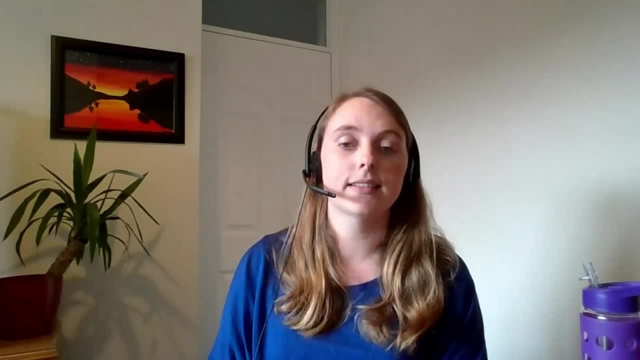 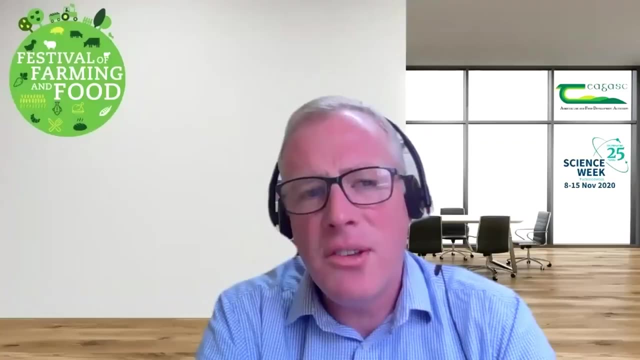 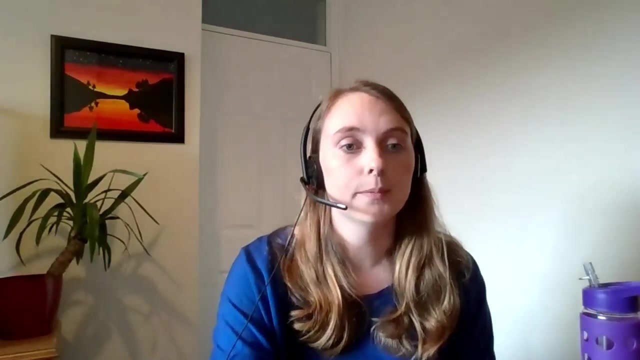 high diversity of plants, as Ghilan has shown, that this will also hopefully increase the microbial diversity as well. Are there such things as good and bad microorganisms found in the soil, Aoife. So you can have bad microorganisms, which are called pathogens, that cause plants and human. or animal diseases, but there's also the majority of the microbes you find in the soil are beneficial. So the main message again is: high diversity will more likely keep those pathogens numbers low, but also plants. most plant species have a natural resistance to the pathogenic infection. 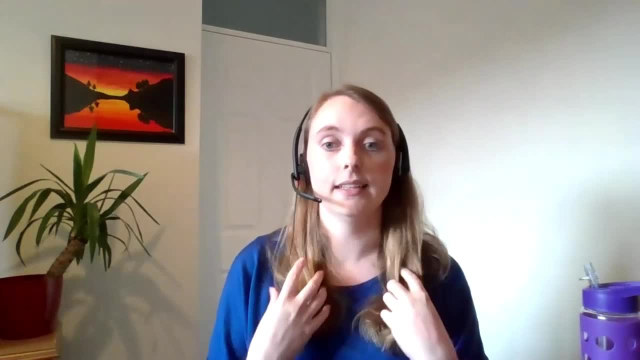 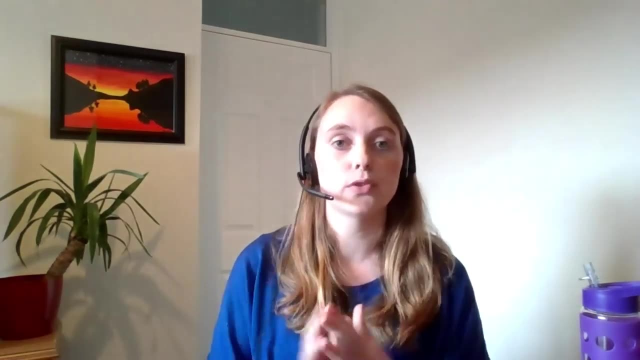 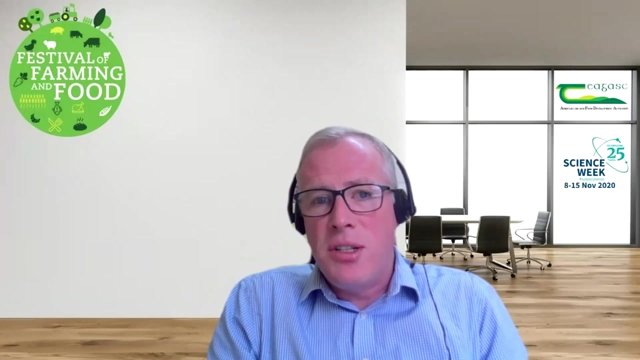 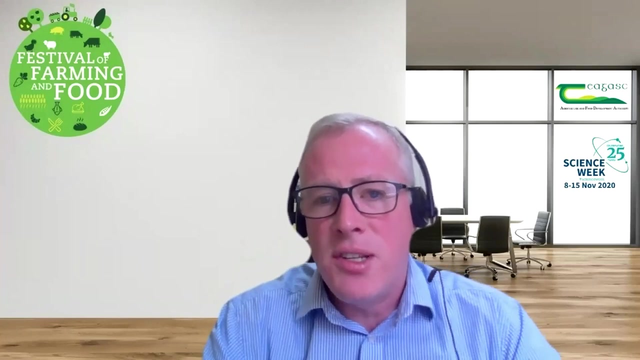 so disease outbreaks can be controlled by, like say, pesticides and that. but hopefully we'll start moving towards more bio controls. Yeah, and I think certainly the EU Farm to Fork Green Deal project over the next 10 years, which aims to reduce the amount of fertilizer used and pesticide use, will. 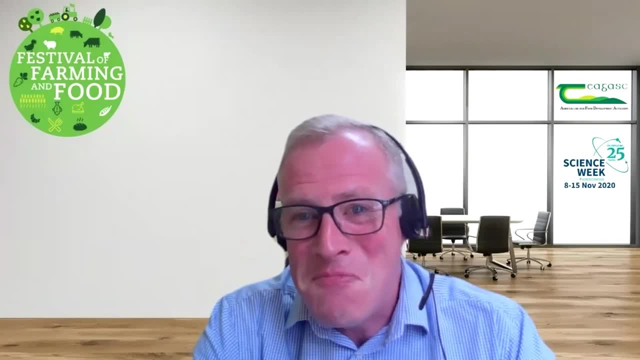 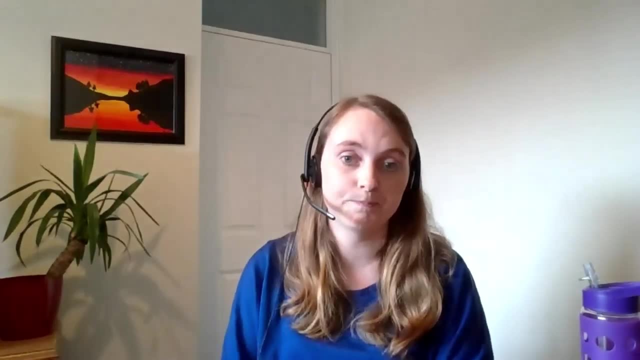 probably will be good for the soil Aoife. yeah, Definitely, definitely. yeah, It'll all contribute to the diversity of the microbes and the health of the soil Right. just one other question to you. going back to my first question: How invested are farmers in all of this? 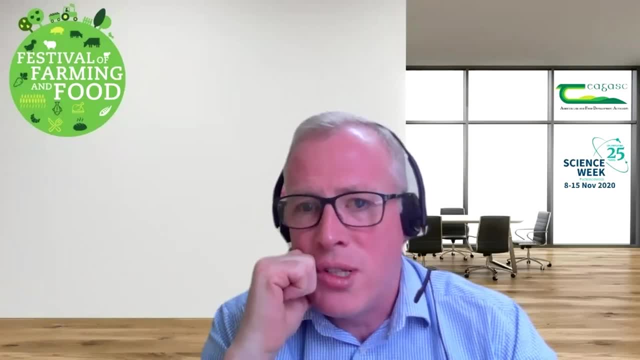 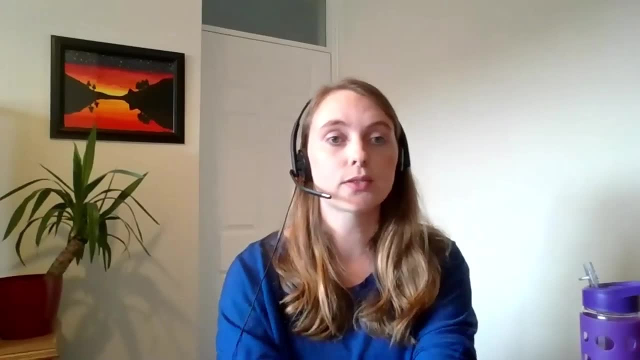 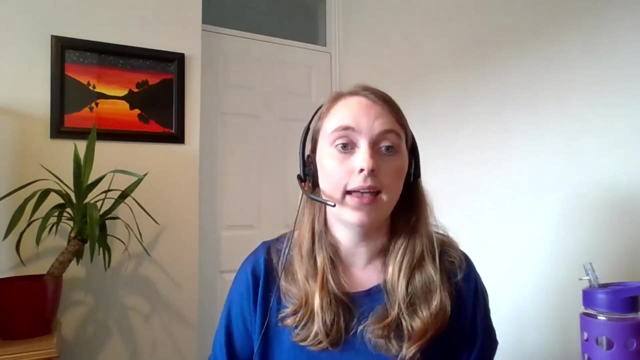 in, you know, quality soil, multi-species, swords and all of that. is this something that's becoming more of a priority, do you find from your interaction with them? So in Chagas, that's what we're definitely trying to investigate and hopefully promote. so farmers, I think, are taking it on board. 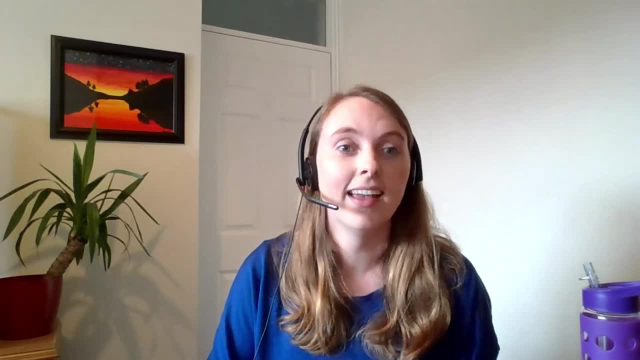 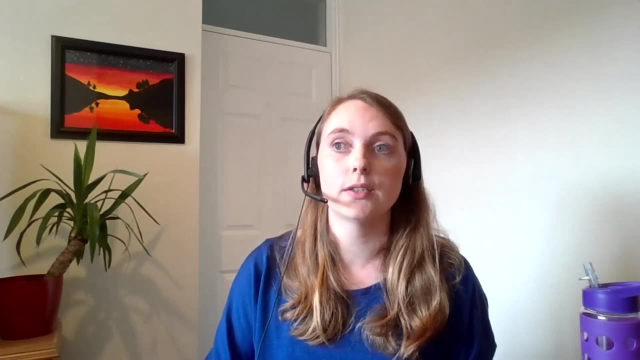 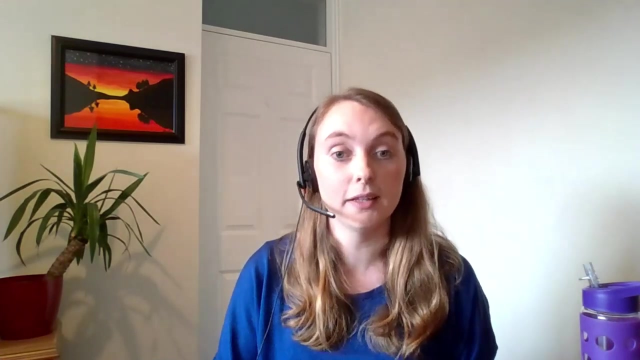 but they do need convincing. so obviously they want to make money. so we want to prove to them that this can be done, and can be done sustainably, and it can make a profit for the farmers. Yeah, yeah, Well, that's the title of our 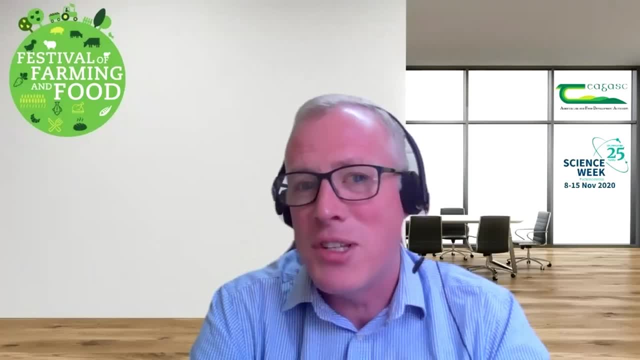 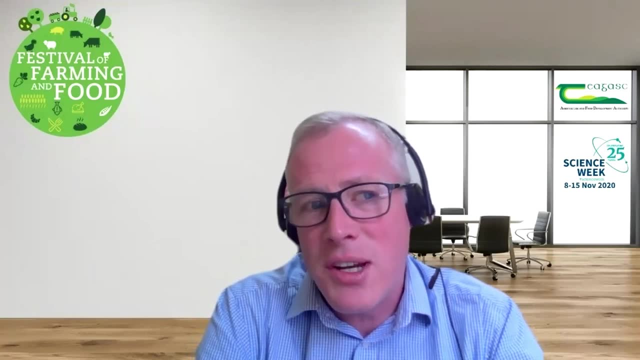 discussion this morning. soil health is our wealth, and if farmers can get that into their minds, certainly it'll be good for us all. I just want to stay with us there, Aoife. I'm going to move on now to Luis Lopez, Sanji Luis. 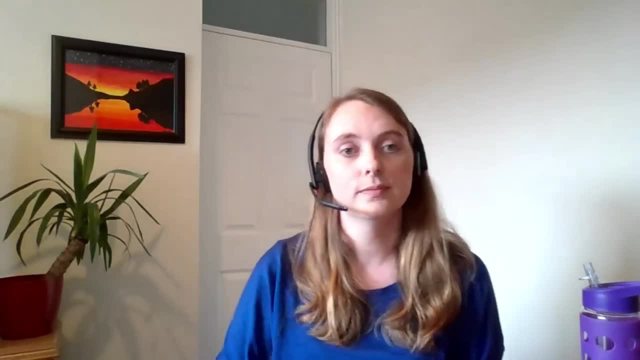 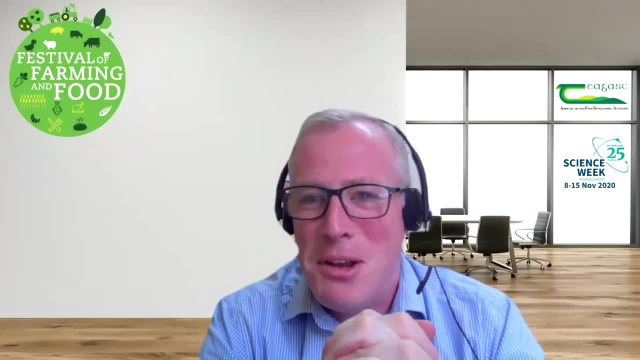 good morning to you. Hello, good morning. I think I have a problem with my video. sorry for that. That's such a pity. we'd love to see your pretty face, but we can listen to your voice. Luis, with a name like that, I suppose the first. 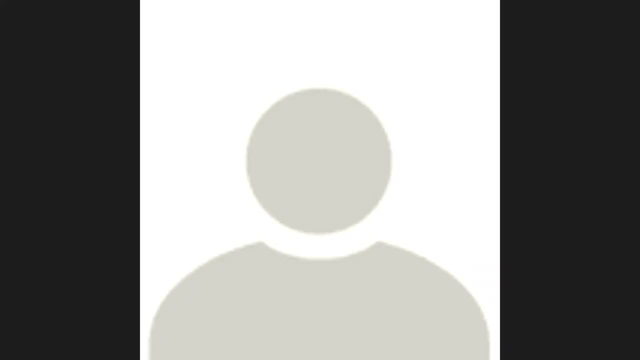 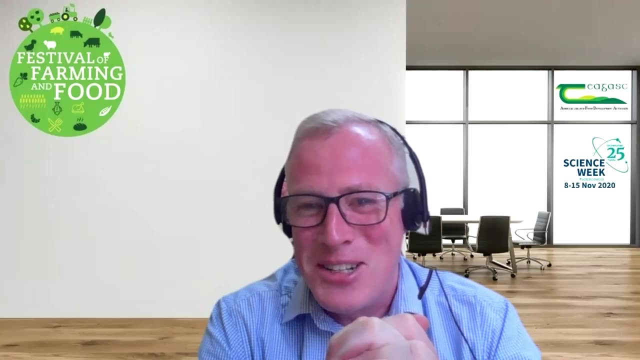 question I have to get out of the way. where are you from? Spain, as you can notice from my accent. Yeah, yeah, we remember Manuel in Fawlty Towers. alright, there's a bit of a similarity there. You're too young to remember that, but anyway. 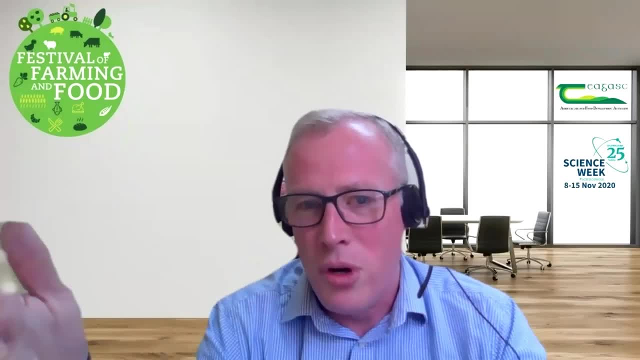 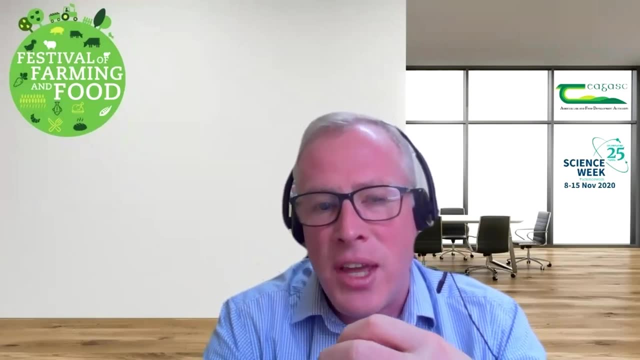 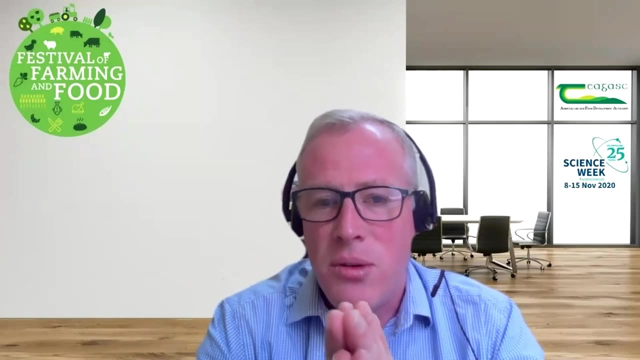 listen. it was really, as I said to Aoife, their fascinating video and wonderful work that's going on down there in the sunny southeast. Can you tell me about any soil disaster that has affected or is still affecting humans in more recent times? you know, because I really was and I'm using 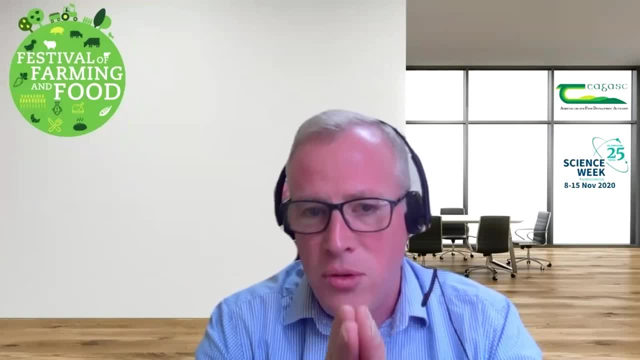 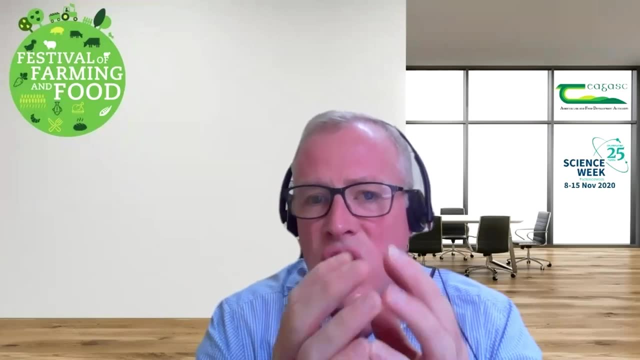 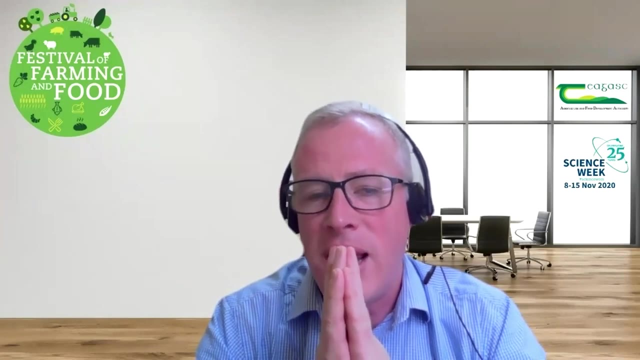 that word again fascinated to discover- I think it might have been you that was saying it, Luis- like in a handful of soil, the millions and millions of living things that are actually there and the story behind a handful of soil. so it is really important to us. but have there been any? 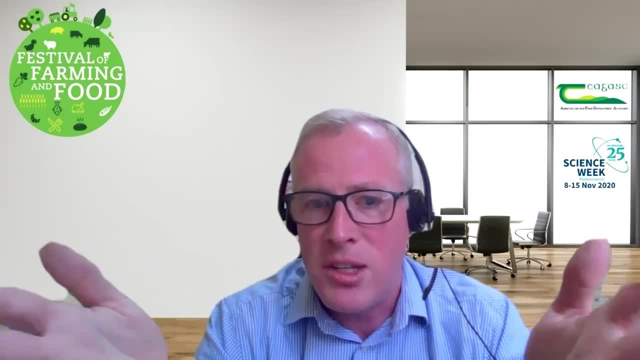 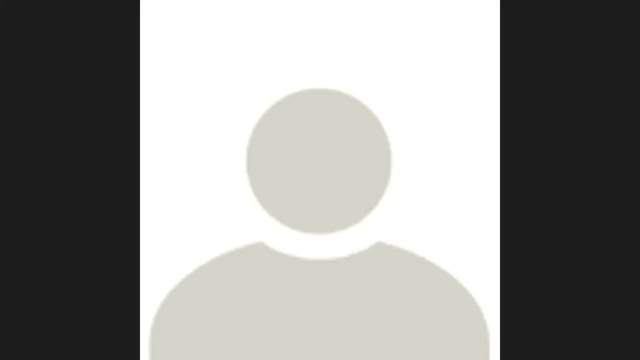 disasters. you know, going back that we saw them going back in history there, but what about in more recent times? So globally, I would probably pick like soil erosion. erosion is at the moment the silent killer of soils. I would say globally because it's a bit difficult to. 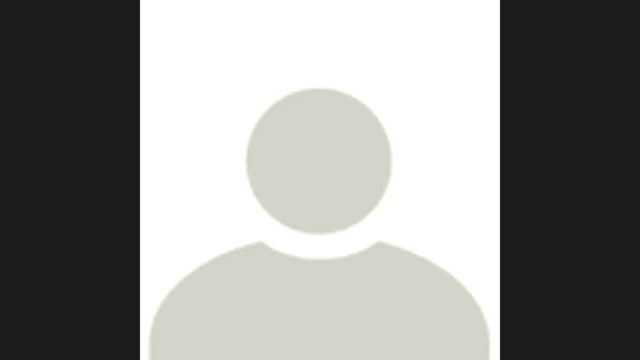 pick up this with the naked eye for normal people, right? so you think that at the moment, we are losing globally like 24 billion of fertile topsoil into our rivers and seas? that's a lot of soil that is being washed away, so it's fertile soils and nutrients as well. 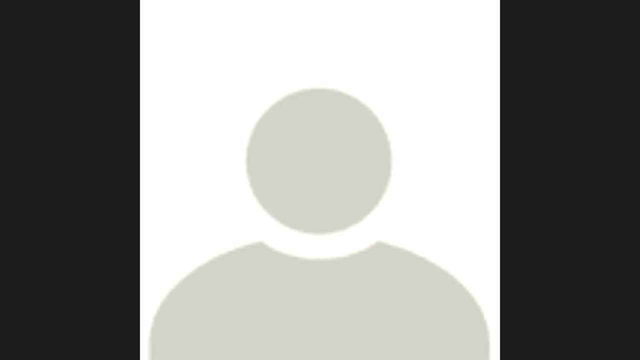 right, so this is very bad. this is something that could be say like catastrophic if you think it takes like 500 years to form only one inch of topsoil in normal average agricultural conditions. right, so it takes a lot of time to form. I've been 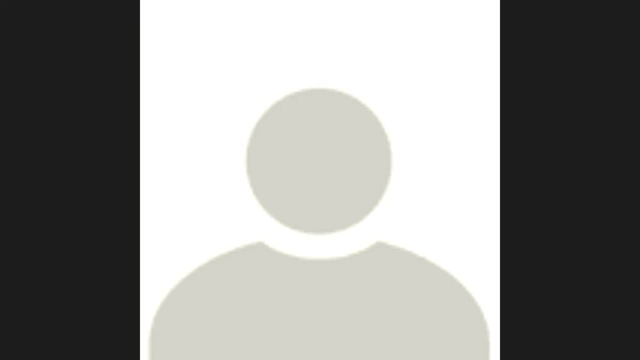 in places, in croplands in the mediterranean and also here in sloppy areas that you can see more, even more than an inch of soil. it's been literally washed away during heavy rainfall, heavy rainfalls after only a few years, really. so you can see. 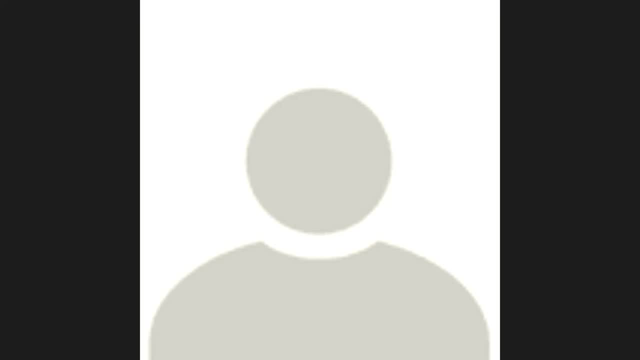 like when you see all those, all those brown rivers and streams with this brown color of soil being washed away with not only soil but the nutrients. it's something that it's very bad. it really hurts my my soul really. so it looks like for me. in many areas we are repeating. 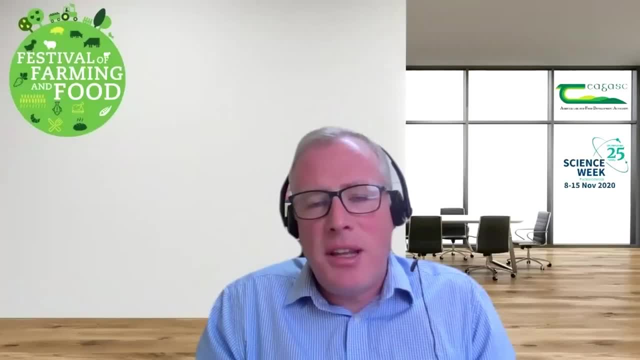 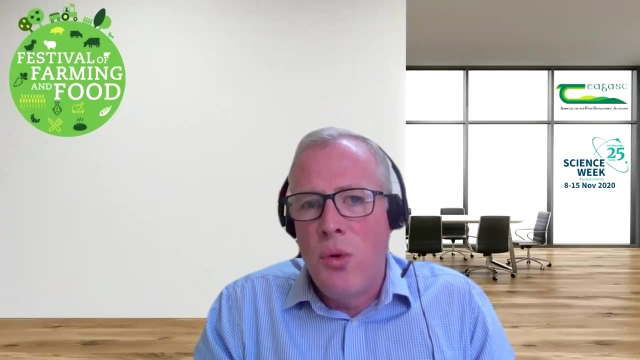 the same history of Greeks. really, yeah, that that is very interesting. you know, something that takes 500 years to mature in five minutes can disappear. so, Luis, obviously you're saying heavy rainfall, it's climate that is having that impact. so how can we kind of rest or redress the situation? 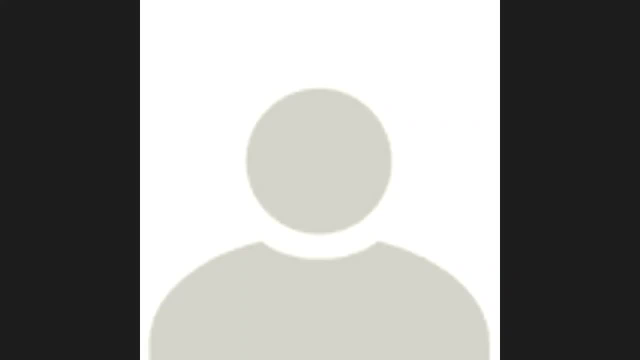 probably best thing, or one of the first solutions, would be to not to leave soils naked without the plant cover. it's a main issue that we are having at the moment in many areas in which, after crop lands, especially in crop lands, we leave the soils naked and then 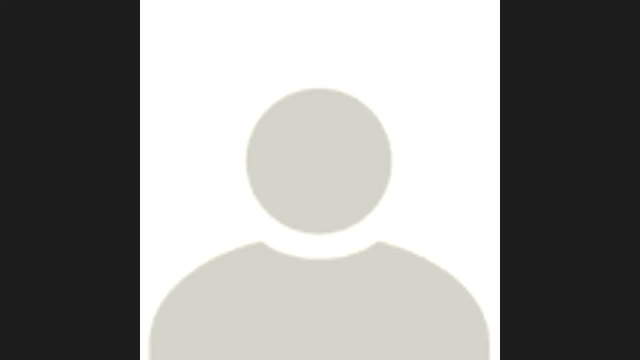 a heavy rainfall comes and it literally washes away the soil. so there are no roots in there that can hold on to those soil particles, and then it's been. if you do that years after years after years, you are literally losing inches of soil away. so there are in some 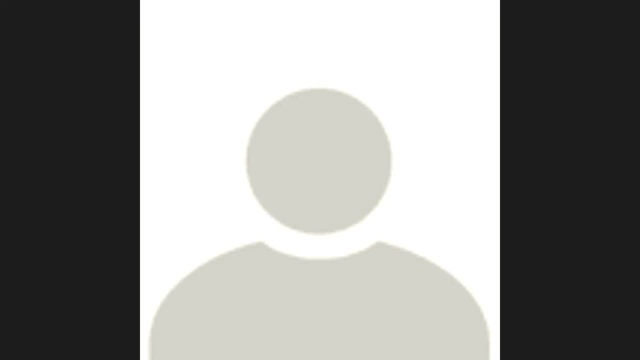 areas actually in which there have been studies calculating the rate of soil loss and it has been like calculated that we are only having like 50, 100, less than 100 actually years of crops if we are not keeping that soil, so definitely not leaving the soils. 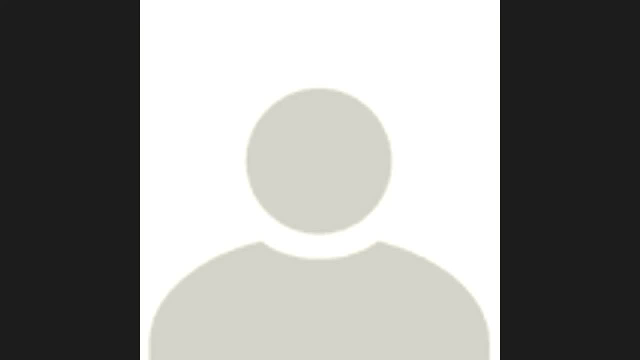 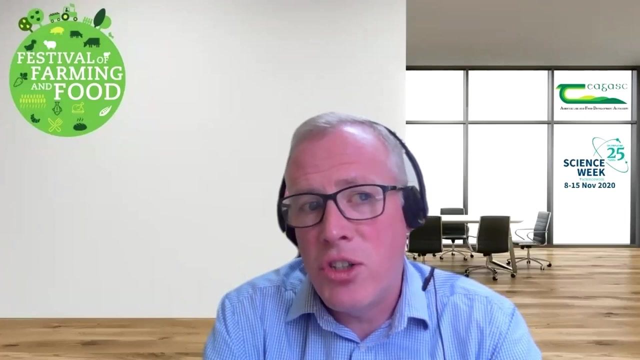 naked, having cover crops catch up, crops that can hold on the soils, that would be a good point, especially in places here in Ireland where there is a lot of rain. yeah, okay, and that brings me nicely on to Gillian Grange, in terms of Ireland specifically, when you talk: 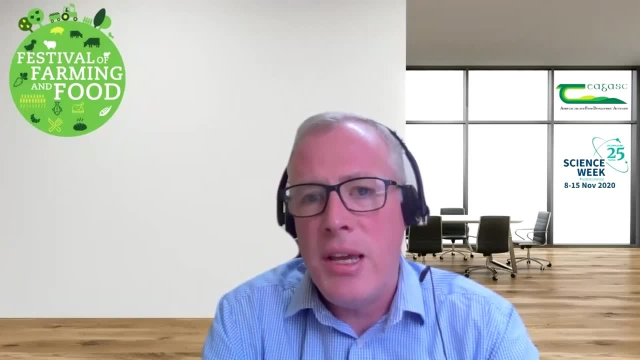 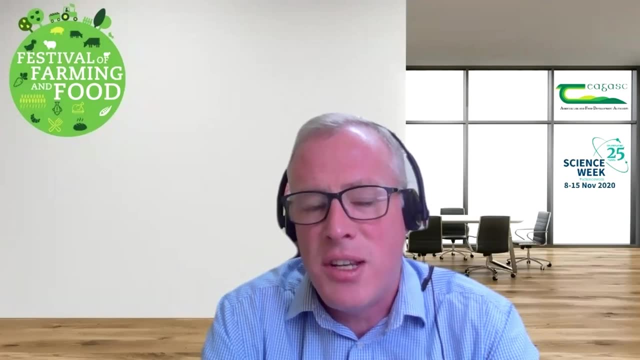 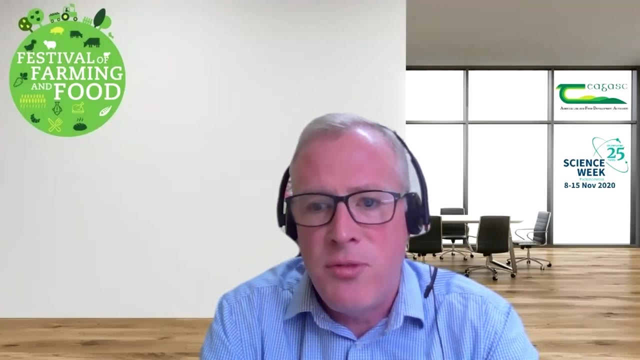 there, Luis, about not leaving the soil naked and about cover crops. of course, the most prominent cover crop- you could call it- that we have in this country is grassland, is pasture all over the country. so, Gillian, when it comes to grass production, which was featured a lot in that video, 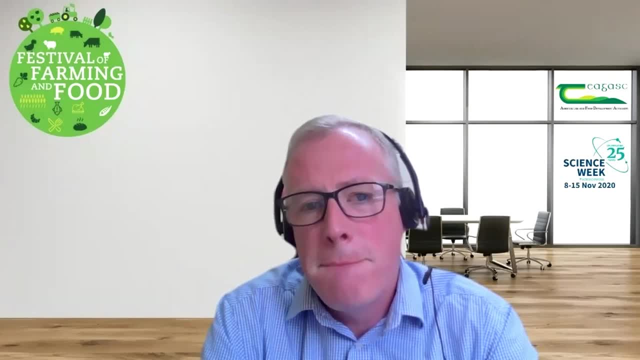 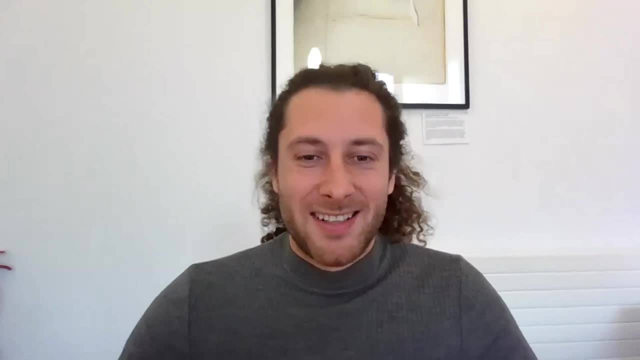 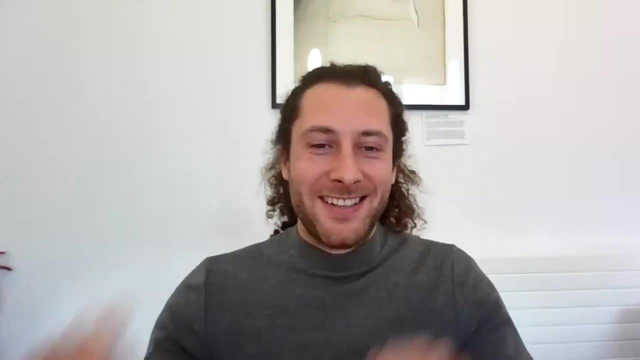 what else can we get from the soil? calling Gillian, maybe unmute. hi, how are you, I'm sorry. hello France. so we are moving from Spain to France, am I right? completing the UN panel? but yeah, no, just talking there about the importance of grassland pasture in Ireland. 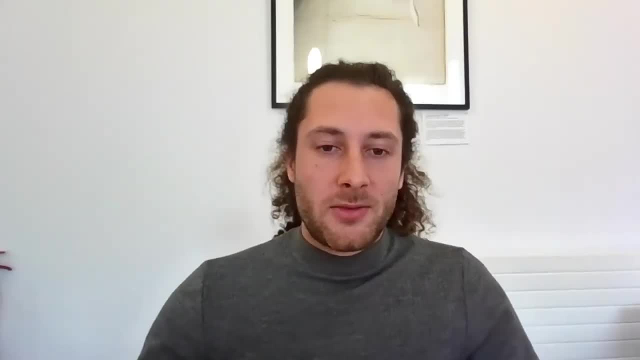 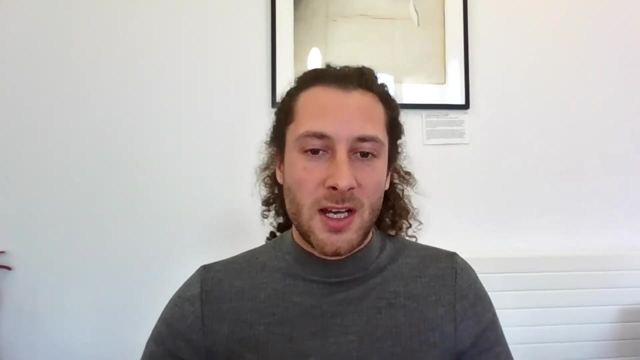 good for the soil? yes, so of course, like as a French, I can say that we are all jealous of Irish grasslands because they are so green and they look so great and it's actually a very good way to protect the soil health, because it's always covered. 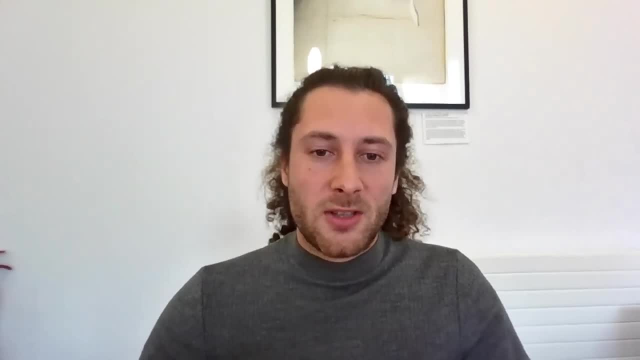 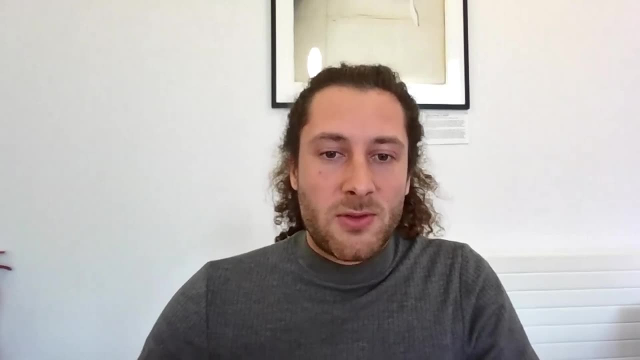 so the raindrops cannot harm the soil- the bare soil- and the sunlight don't reach the the soil neither. so it's good to keep good soil health. but of course you cannot produce all what human needs from grasslands, and so that's why we have also crops. but 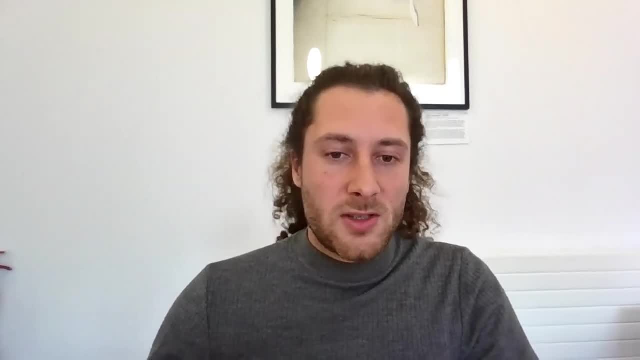 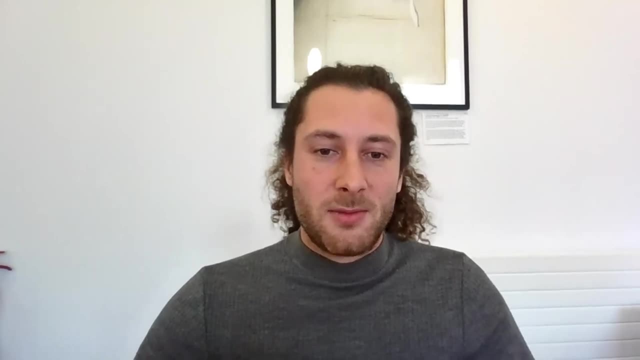 soil is actually at the origin of much more than just our foods, because also the fiber that's- for example, I'm wearing a wool jumper today and maybe you have a cotton shirt- and that's all derived from soil, because everything grows on the soil and also the forest. 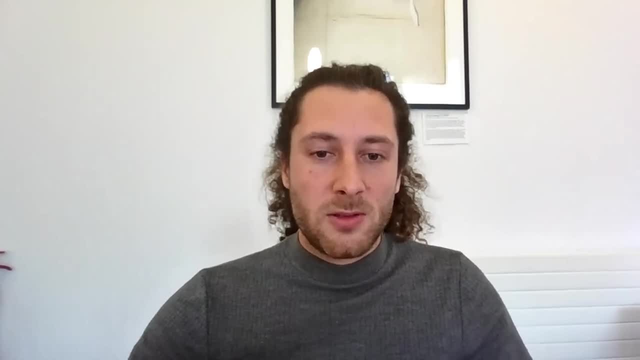 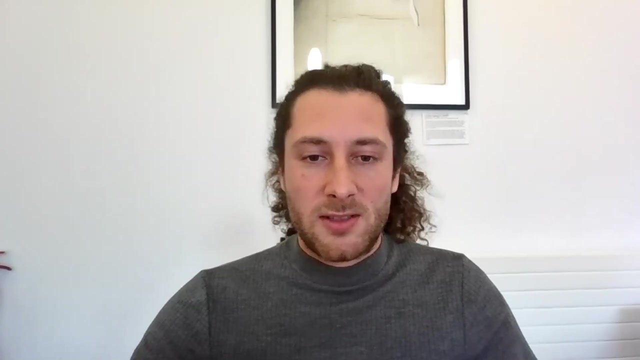 grows on the soil. so this production function of the soil is also at the origin of the paper we write on. the newspaper we read is derived from soil, and even the fuel that we burn from having warm houses, like the turf, is soil derived. the oil is soil derived and very ancient. but 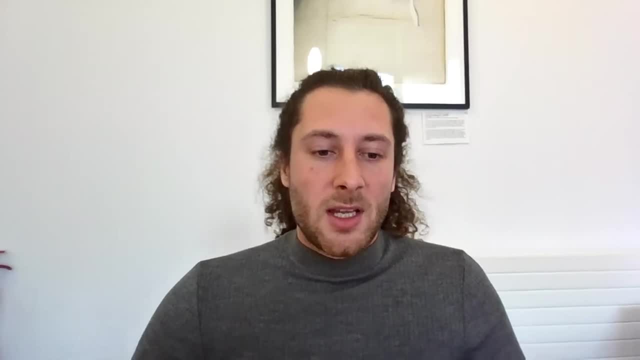 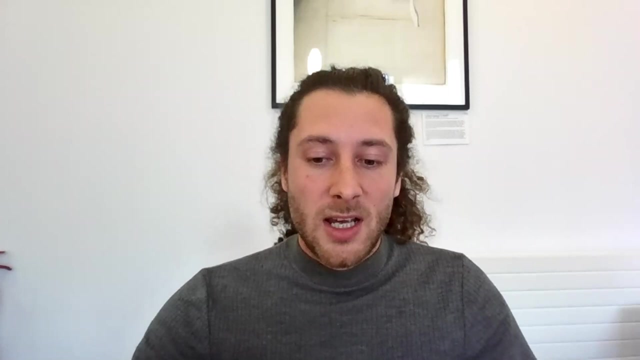 of course it's. it was plants growing from the soil, and so that's even the most renewable energy. the timber is soil derived. so soil is at the origin of almost everything in our daily life. even the plastic is derived from the petrol that is derived from the ancient plants growth. so 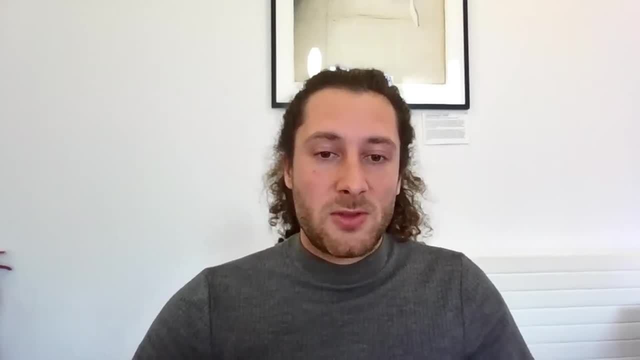 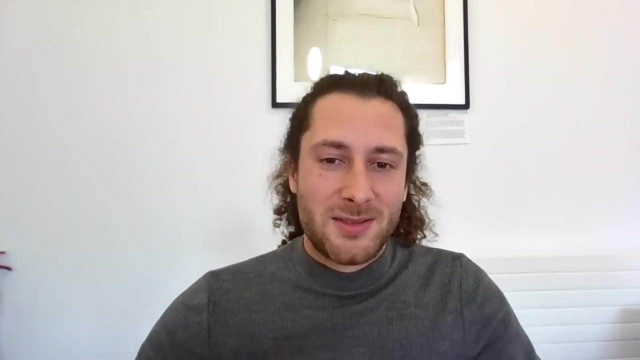 we have to make sure to take very good care of our soils and, as citizens, the things- easy things- that we can do is eating sustainable foods and making sure that we use renewable energies- all this kind of stuff. that's a good way to keep our soil healthy, yeah, and 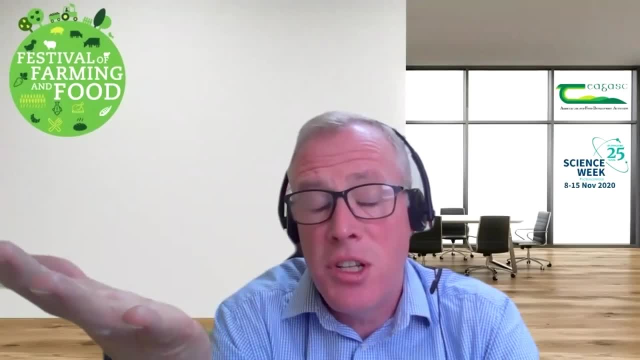 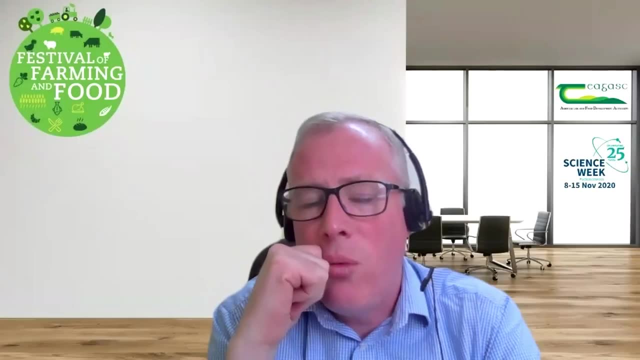 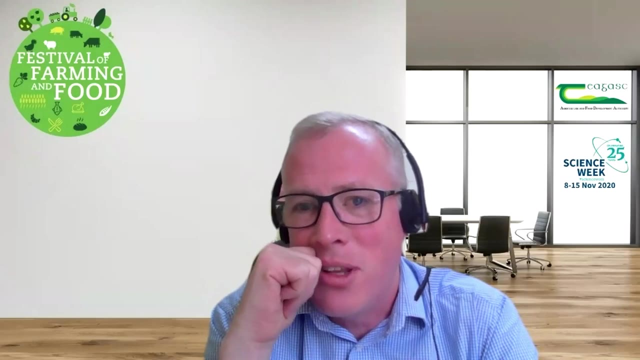 I'm just wondering if we go back to farming again, and you know the predominant, the dominant form of farming in this country, as you know, Gilane, is obviously livestock. what about you know? organic manure? obviously cattle pooing on the grass where they're out nine months of the year and then 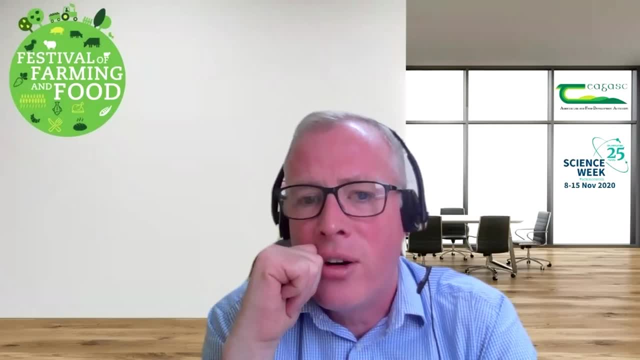 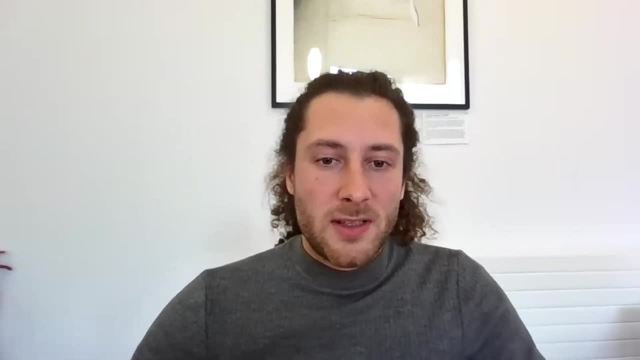 we spread slurry as well, is that? what sort of an impact is that having on our soil? so the best renewable farming is the one that is self sufficient, so, as in developed, then we can recycle nutrients and so we can produce food from grasslands and then the animals redeposit. 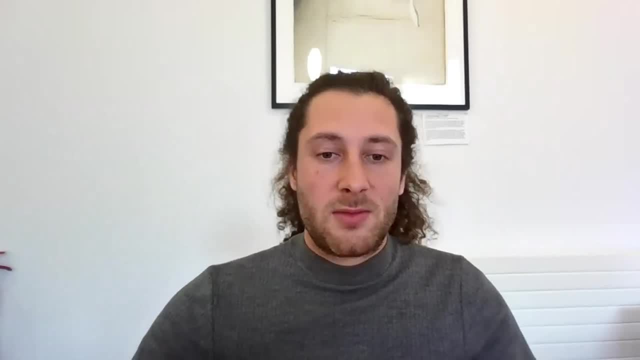 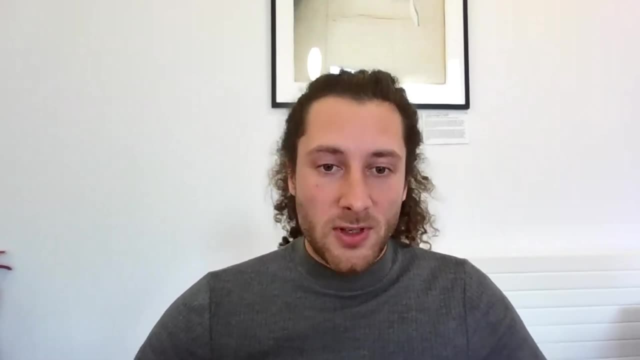 the manure or everything that is brought back to the soil and then bring nutrients back to the ground, and so that's a very good way to recycle nutrients and produce food on a very sustainable way. so in this way, the grasslands are very good and the most organic. 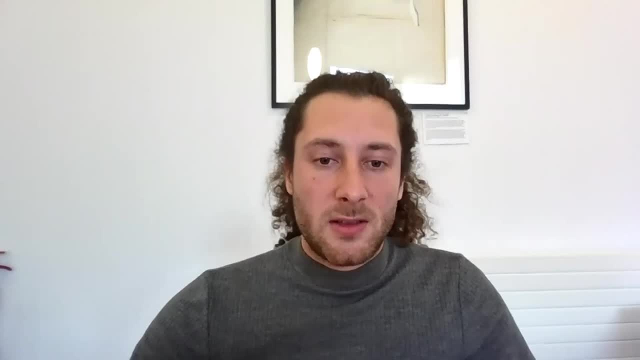 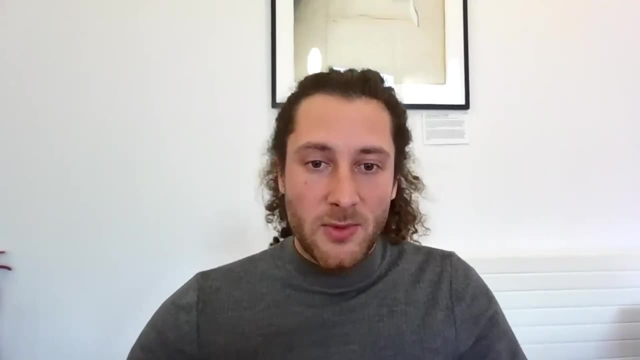 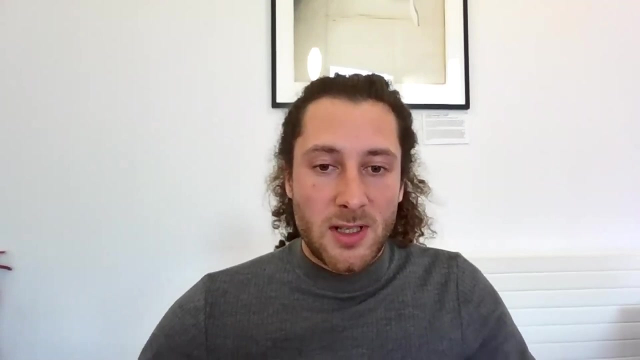 manure you use, then the most sustainable it is. and the only point is, because we produce much food from the soil, then we have to bring some nutrients to this. so that's why sometimes fertilizer is used, and the problem is that fertilizer can lead to greenhouse gases emissions. 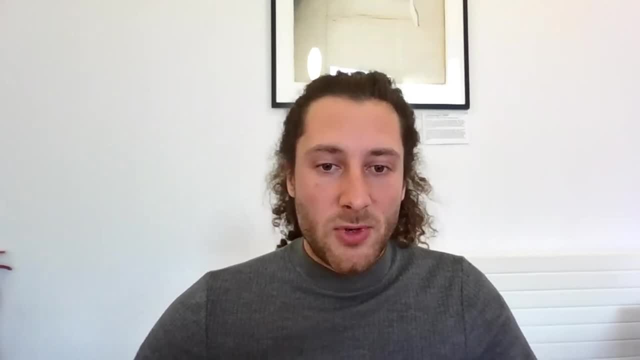 so that's why we promote the use of clover, for example. that can bring the fertility to the soil by fixing some nutrients that they actually derive from the atmosphere. so it's for free and it's sustainable. so that's why we promote clover here in Johnstone. 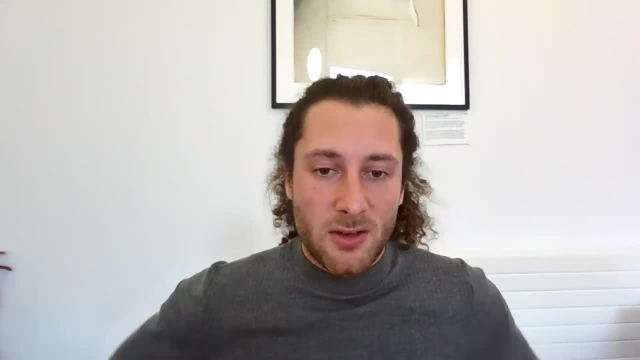 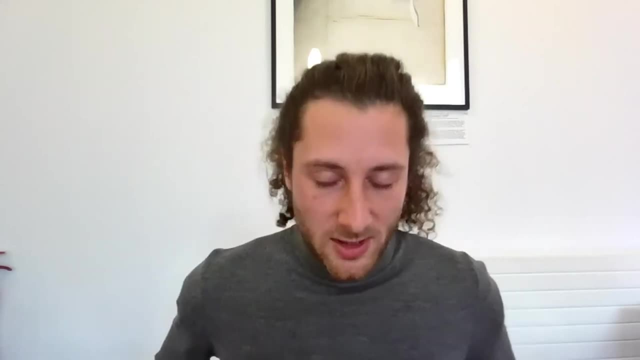 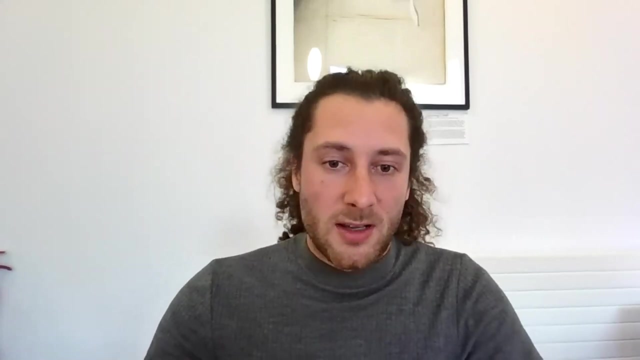 Castle and the use of other species as well that have many other benefits, like, for example, they promote pollinators coming to the fields, and so on. so plant diversity in grasslands plays a very good role in soil health, but also in the whole ecosystem health. All right, and just finally to yourself. 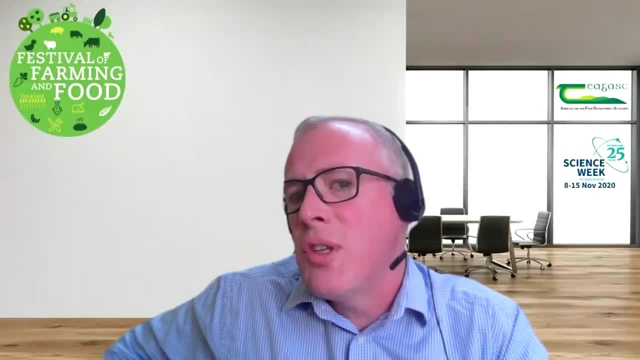 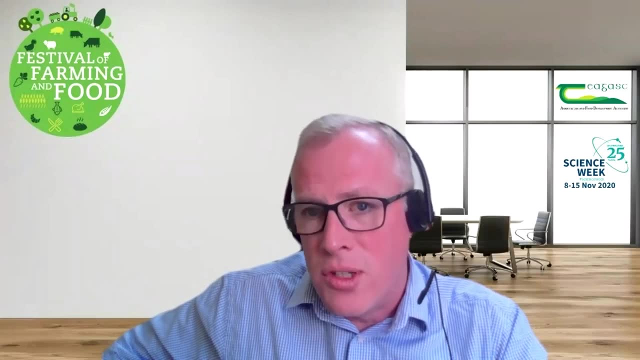 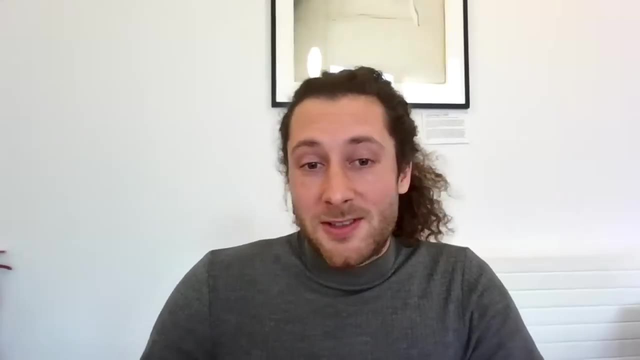 Ghilan, because the question I put to Aoife earlier on: what is your assessment of farmers interest in the soil now and them realizing the importance of soil health for their good wealth? Actually, farmers are citizens as well, and as everybody. everybody is getting aware that climate is changing. 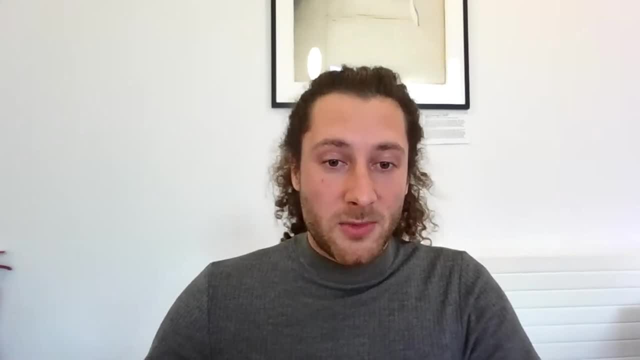 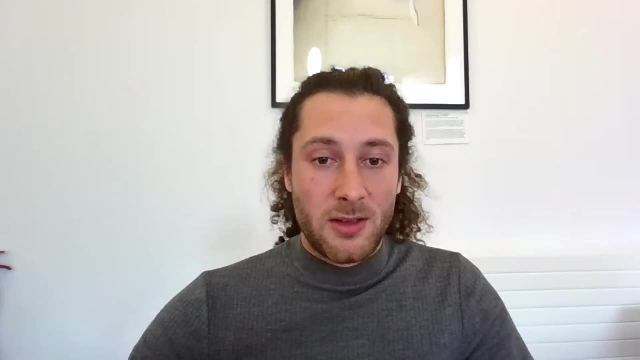 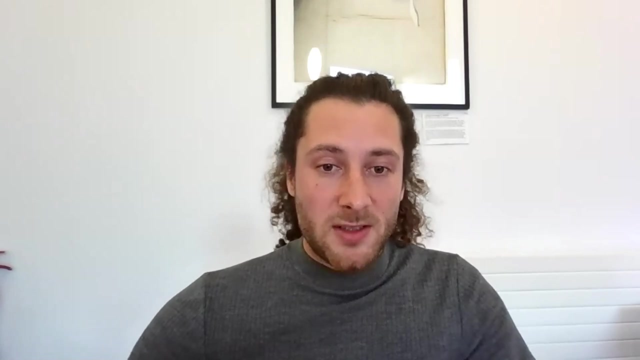 and actually farmers are at the front line when the climate is changing, because when you farm then you rely on regular rainfalls, you rely on first fertilizer price or this kind of stuff. that's all. the climate change can bring much viability in it, so they are the first victims. 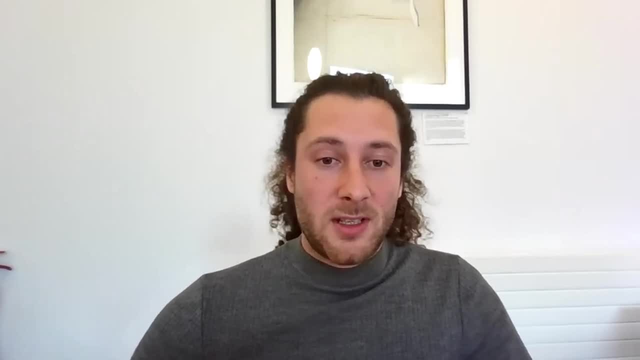 and so they feel very concerned about this climate change, and so there is much interest in getting more sustainable production, and also there is ask from the consumers that ask constantly for more sustainable production. so, like both on the markets ways and their own point of view, there is much. 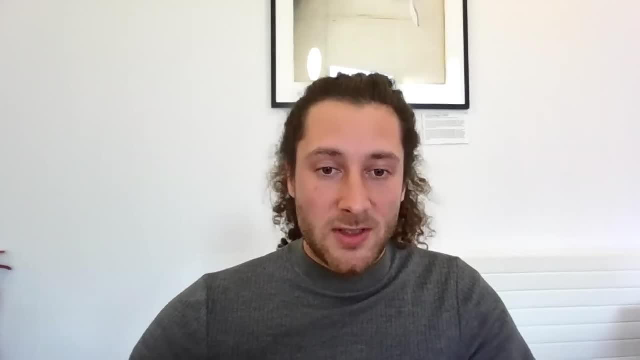 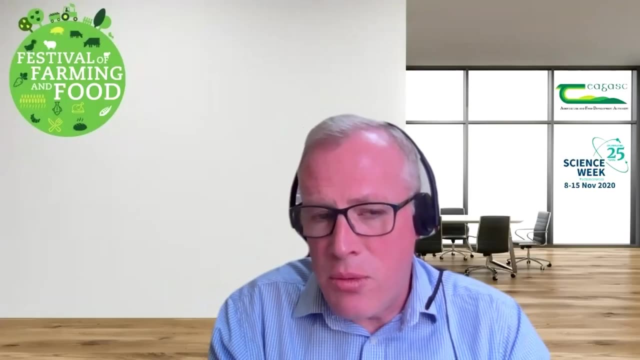 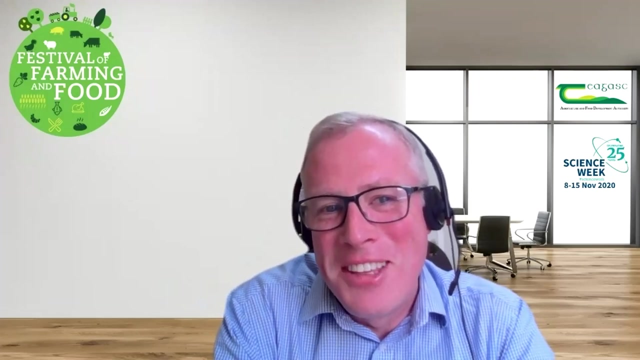 bigger growing interest from farmers about sustainability, and biodiversity is one part of the sustainability. Okay, I'm going to move on. do stay with us there, Ghilan. very interesting there. we are moving on now to Auggie Auggie. good morning to you. Good morning Nathan. how are you? 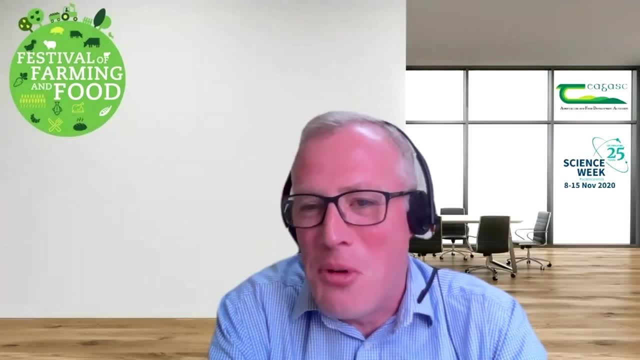 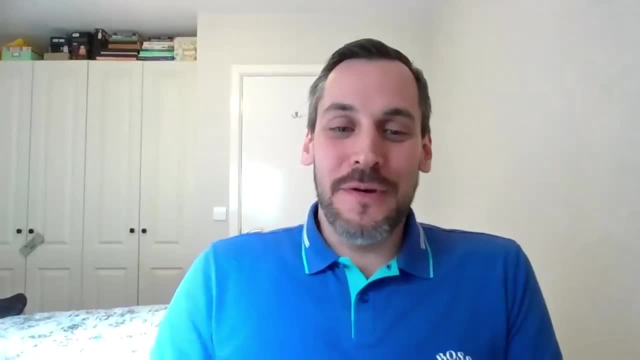 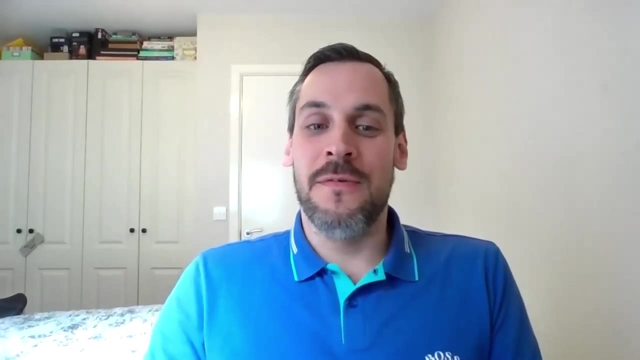 I'm continuing with my UN line of questioning. so what has brought, where have you come from to arrive in the wonderful country of Wexford? well, I was born and bred in Bosnia and Herzegovina, and one exciting thing about science is that you never know where your scientific 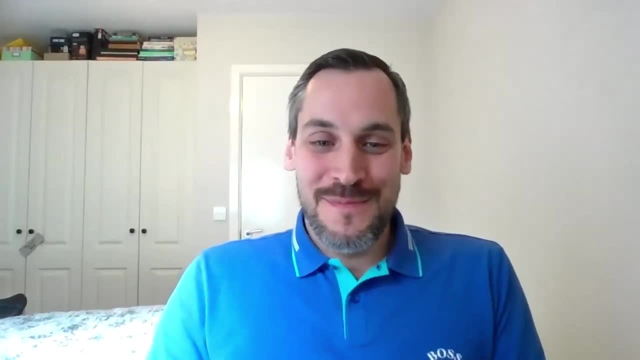 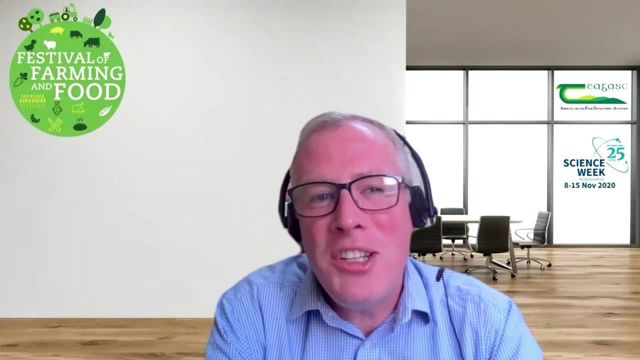 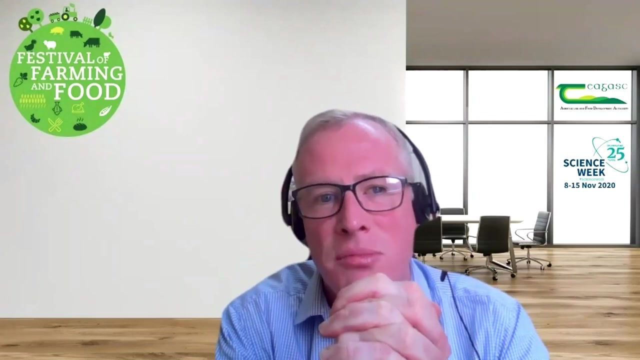 pursuits will take you, and they took me to Ireland. alright, no regrets? no, not at all. yeah, you could be in worse places than down there in in in Johnstown. you mentioned that you're a scientist in the agricultural catchments program. tell us a little bit more. what, what is? 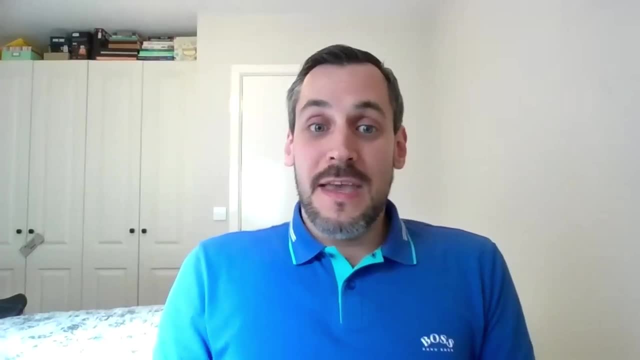 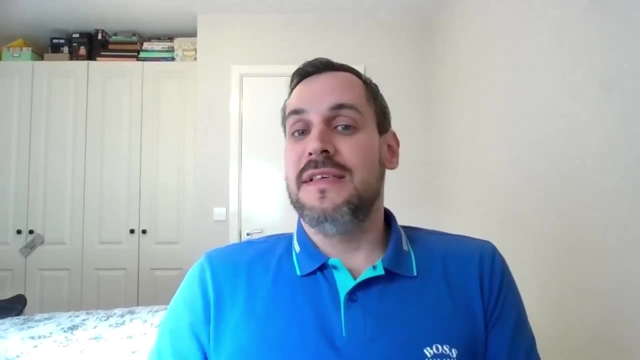 what's that all about? okay, well, first thing for the viewers and who don't actually know what the catchments is. so the simple definition is that the catchment is an area in which water is collected by the natural landscape into a nearby body of body of. 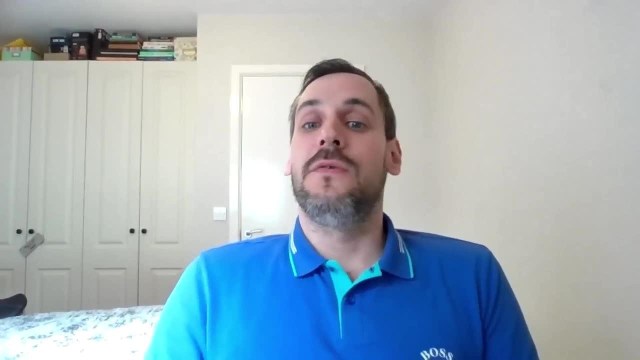 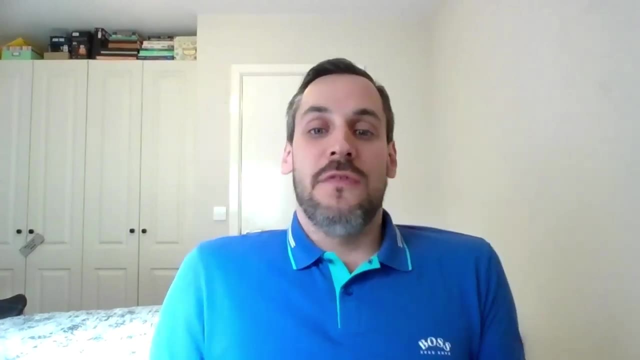 water, such as river, lake or ocean. so, for example, imagine the valley surrounded by hills from each side, so this area acts like a natural funnel and it captures water in that area. and imagine that hills are the edges of that catchment and then all the rain falling on the surface of that catchment. 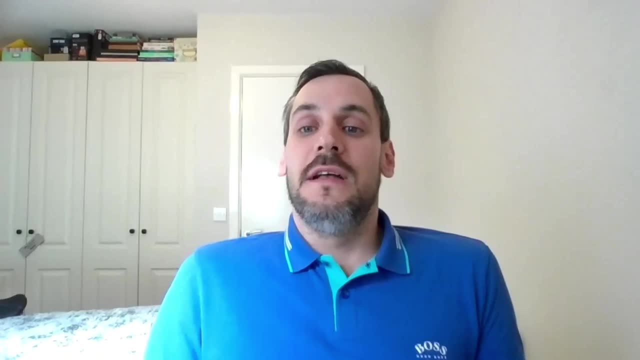 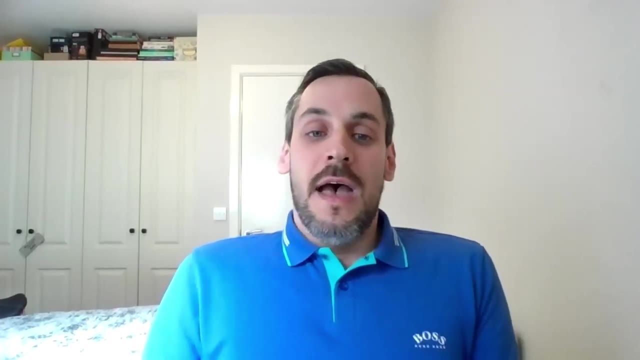 and then all the rain falling on the this area runs down the hill from higher points to be naturally collected by some larger body of water in the lower point of this area, and then the rain outside the edge of this catchment is falling on a different catchment and will flow into. 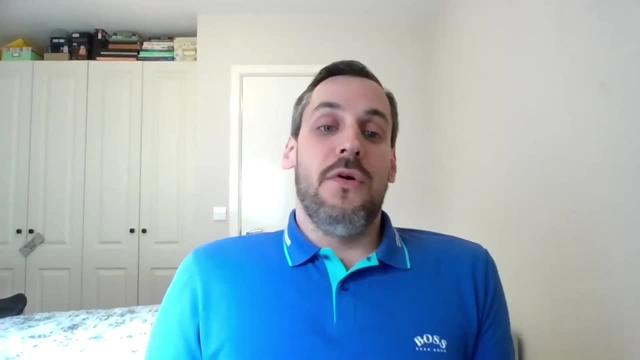 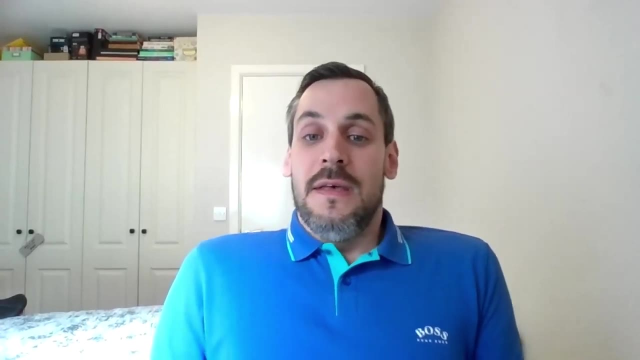 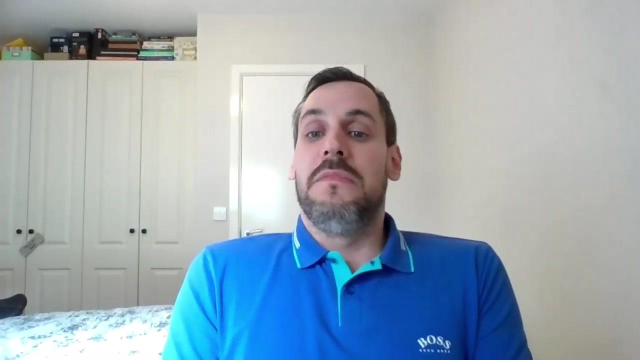 a different river early, so almost every inch of land is part of some catchment and we all live in our local catchment, and a healthy catchment provides high quality drinking water and supports our activities such as agriculture and fishing and, for example, water sports. and then healthy catchments also. 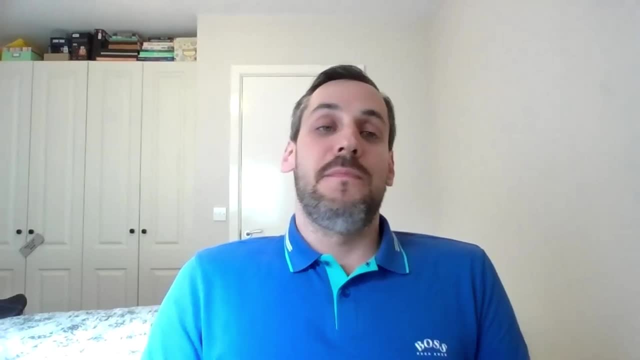 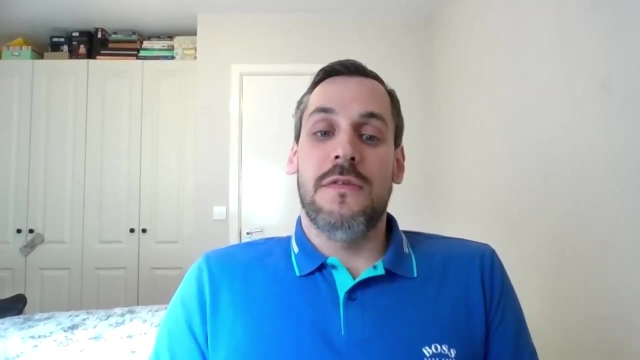 supports local ecosystems, so plants, animals, fish and insects that depend on having healthy water, tribe and flourishing such catchments. so what is our role? what's the Chagas role in in Chagas catchment research? so basically, Chagas agricultural catchment program is a research group of more than 20. 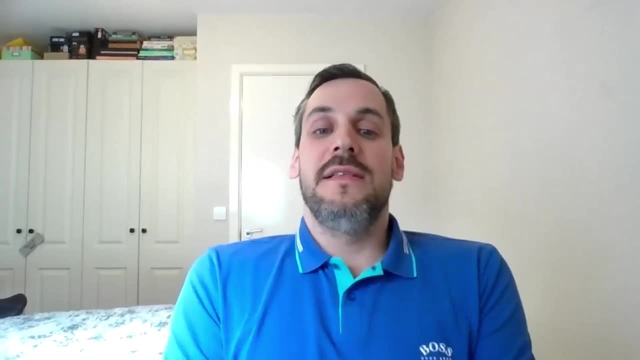 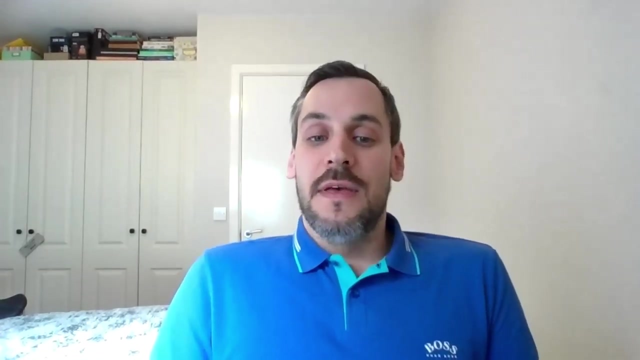 scientists, technical staff and advisors working in the Chagas agricultural catchment program. we are working in six different catchments located in different places across Ireland, and by agricultural catchments we mean that the main land use in these catchments is agriculture. so our main objective, what we do, is to 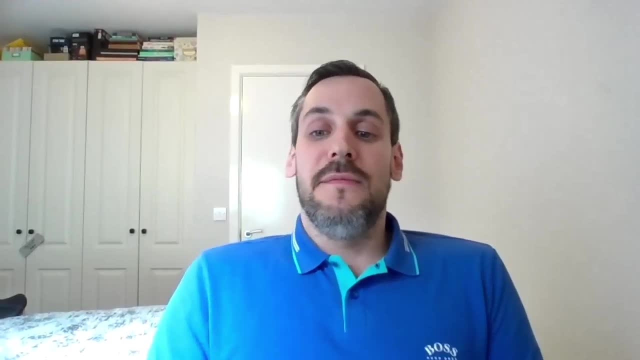 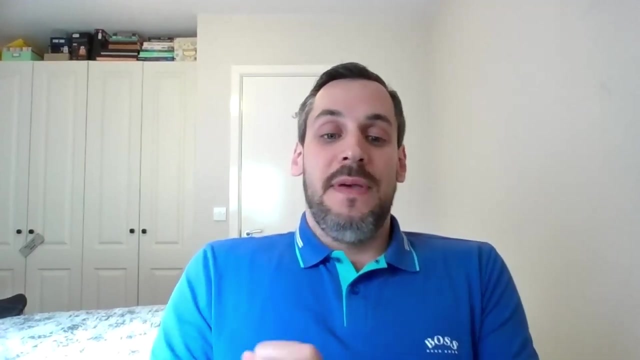 investigate links between intensive farming and water quality in these catchments. so for that we use a variety of instruments and then scientific methods to monitor and impact. they'll monitor the impact of farming on soil and water quality, and we are also very happy and proud to work with 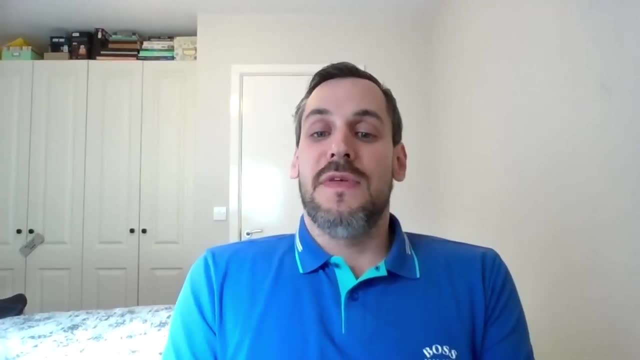 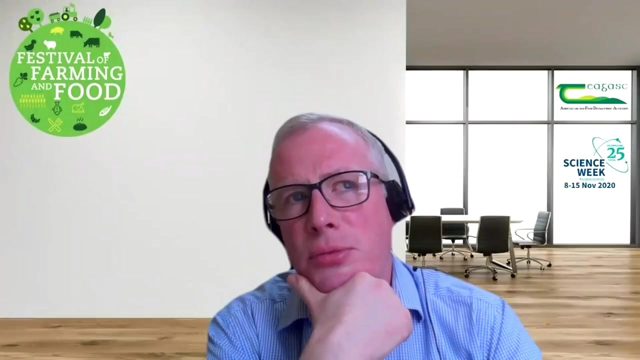 more than 300 farmers covered in these catchments and, based on the results of our research, and we also advise them how to increase their agricultural productivity while also protecting water quality and environment. in terms of water quality and the role of soil as a filter, I was looking at your. 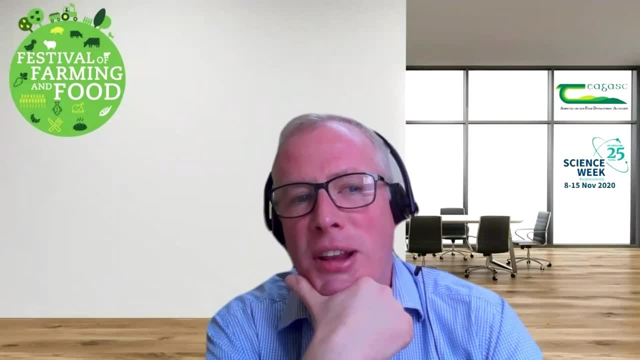 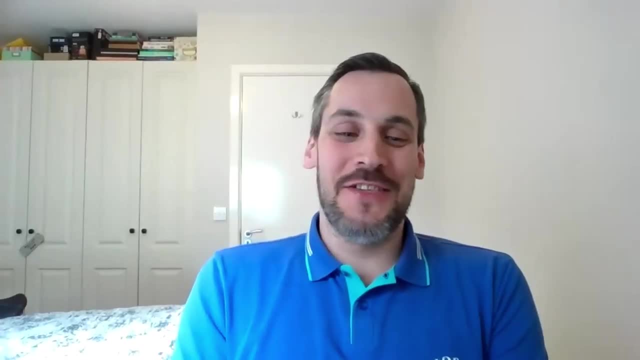 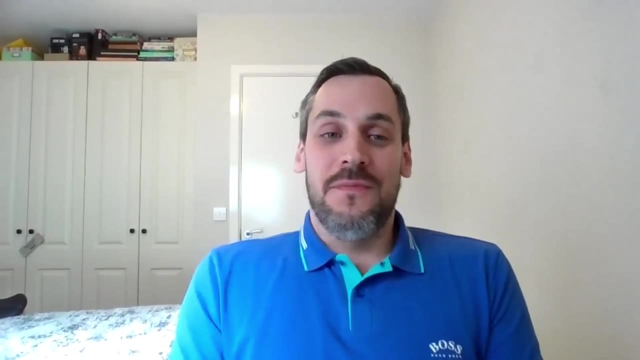 experiment in the video there, where you poured dirty water and it came out cleaner once it passed through some soil. is that water drinkable then? well, that's a good question. I wouldn't drink that water from the glass, and for the reason, as we said, that soil is. 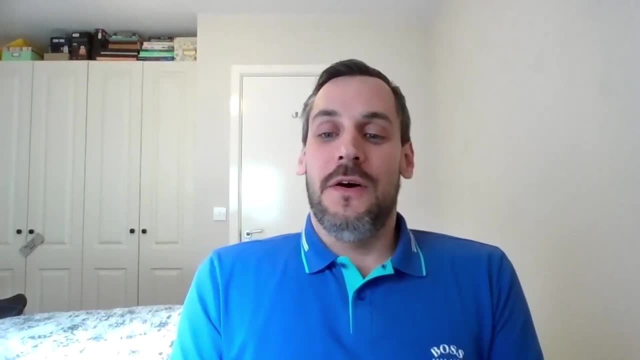 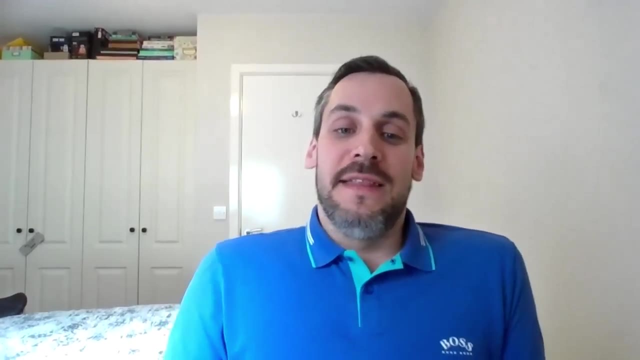 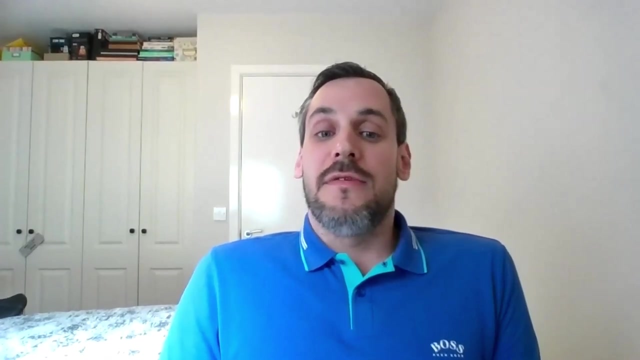 the largest natural filter on this planet. but for that water you've seen in the experiment in the glass, it took only minutes for that water to filter through the soil and end up in the glass. in nature it takes water years, sometimes even decades, depending on the soil. 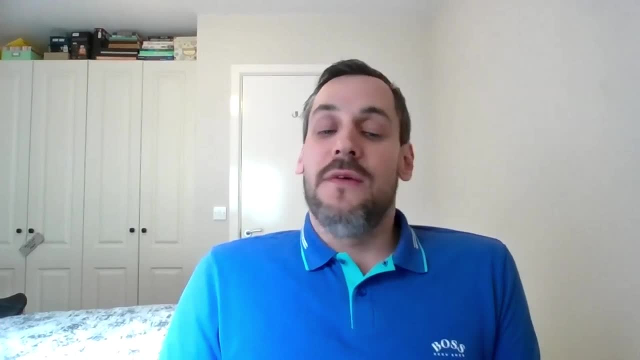 and how deep those soils are for that water to reach groundwater, for example, and so for that reason I wouldn't drink the soil from the glasses. but, yeah, I can explain to you more about how that water is purified on the way down to the soil. so the three main mechanisms: 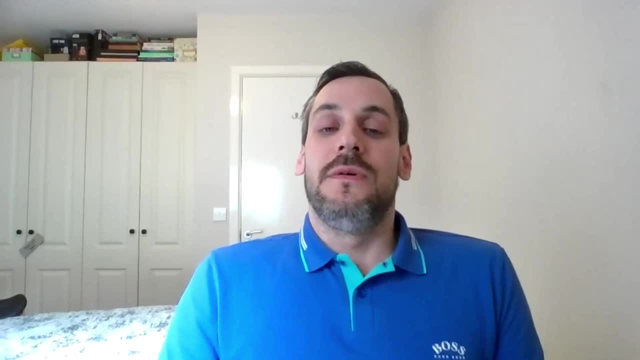 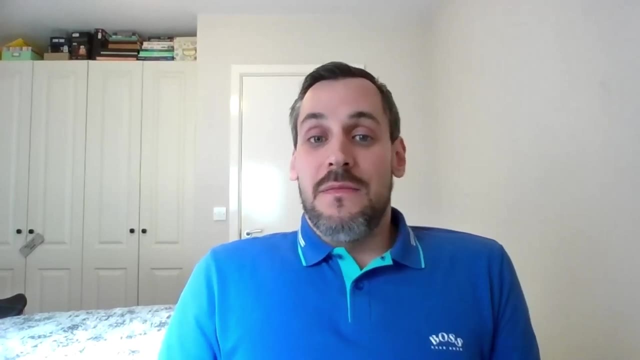 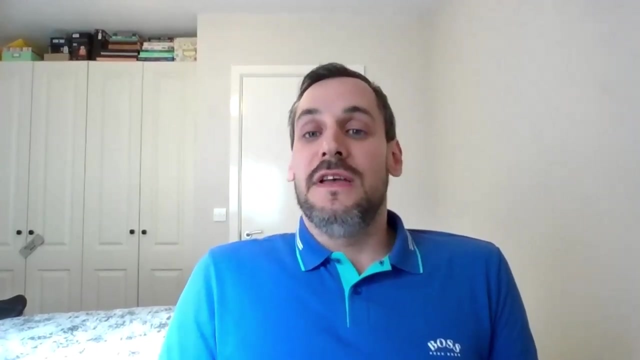 at work. and what cleans water in the soil is physical, chemical and biological. so by physical, imagine that soil is like a big sieve and all the soil pores capture larger particles in the water and they get stuck in the pores and can't move further with the water. and then 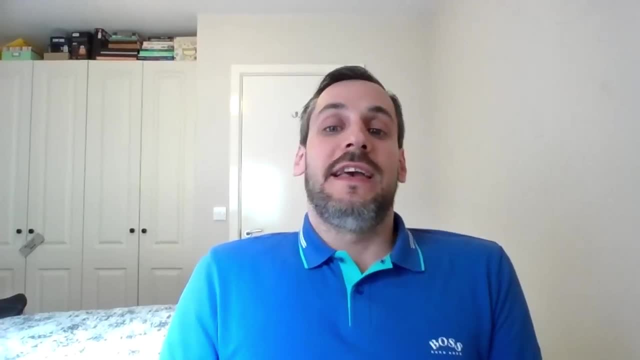 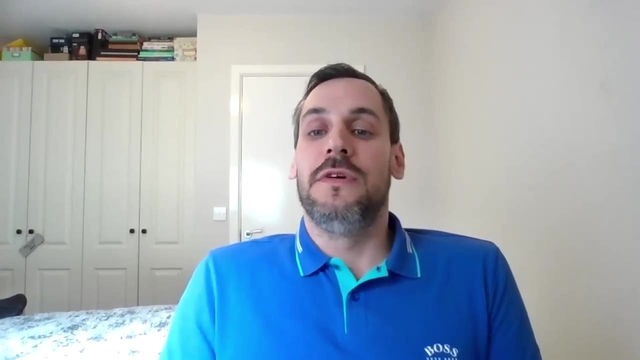 we have a chemical cleaning, so soil particles are electrically charged and they act like millions of little magnets which attract any chemical compounds in the water which have an opposite charge, for example nutrients from fertilizers, heavy metals, pesticides and other chemicals. that's very important and 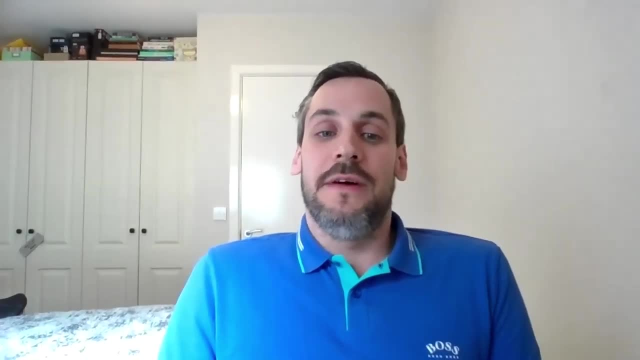 also soils, as IFA and all other participants mentioned. soil is full of life, and particularly a wide variety of microorganisms which have the ability to decompose or transform both organic and inorganic substances which enter the soil. imagine the oil spills on the soil and even 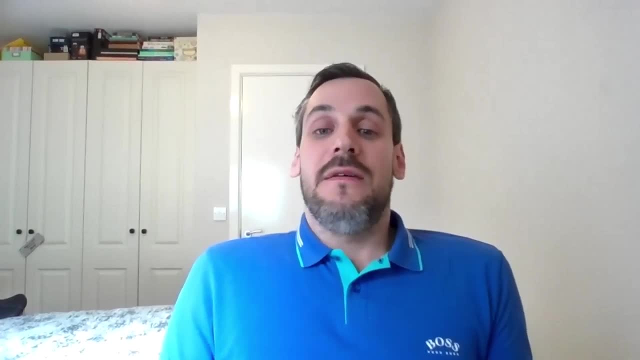 there are even like it's harmful. there are some microorganisms who actually consider well, who can use that oil as a food for their metabolism, and then they transform that oil and decompose them into harmless substances like carbon dioxide and water as the end product. so basically, 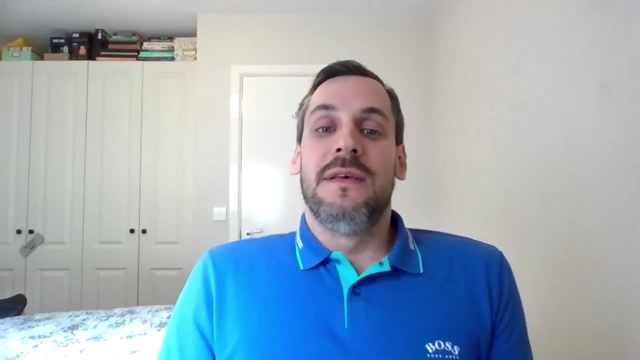 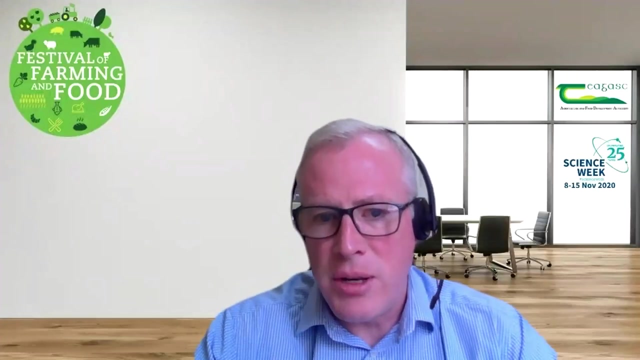 soil. these three functions define how soil, how water, is cleaned through the soil, and this process, as I mentioned, takes years and it's not something which happens quickly. okay, I'm going to move on now to finally to James Rambo. James, good morning to you. morning, David. how are you? 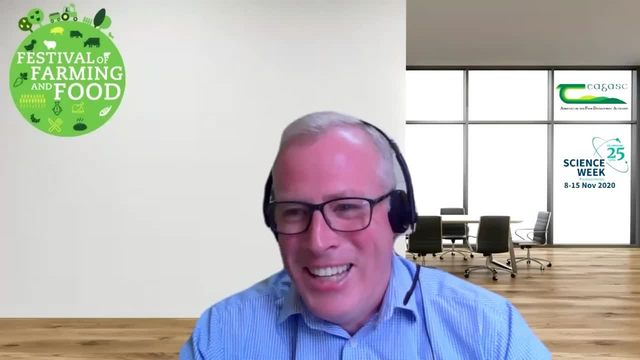 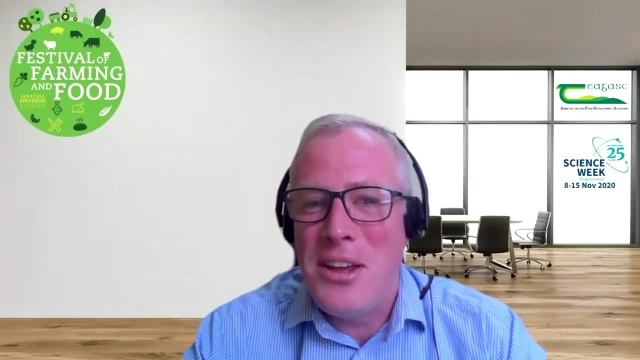 what a great second name when you were growing up trying to impress everybody. Rambo, that was my nickname. yeah, I'm sure it was, and I'm sure you didn't mind it. listen, I really enjoyed your input there into the video and you know. the big question now is we need to reduce. 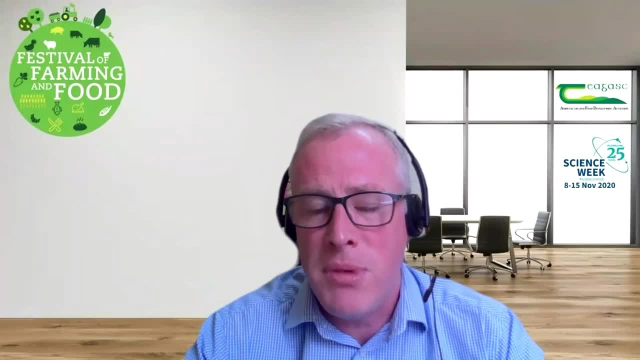 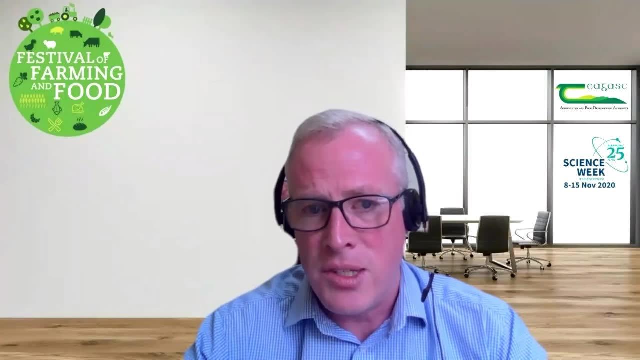 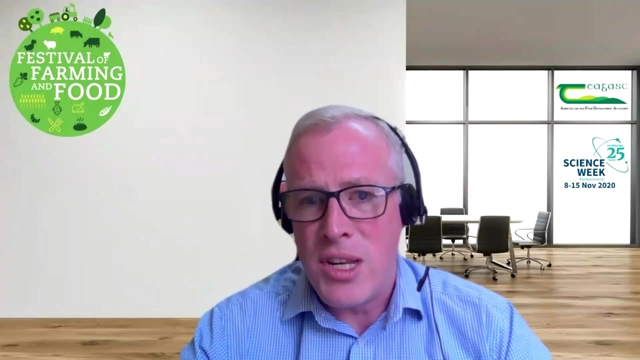 our greenhouse gas emissions. agriculture has to play its part. methane emissions have to be reduced and you know the impact of agriculture on climate is huge in this country in particular. but at the same time, when we talk about sustainability, James farmers say: well, you know economic and social sustainability. 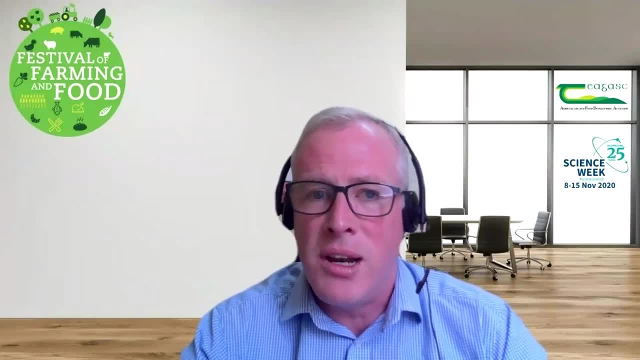 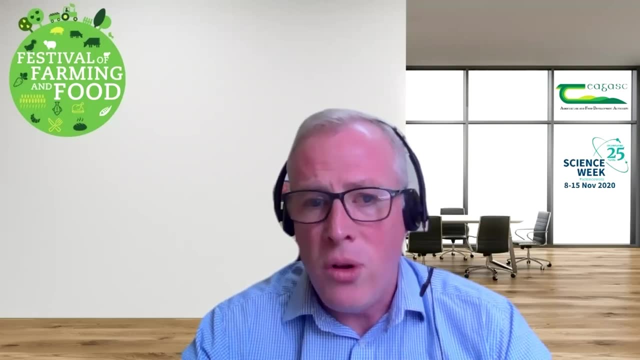 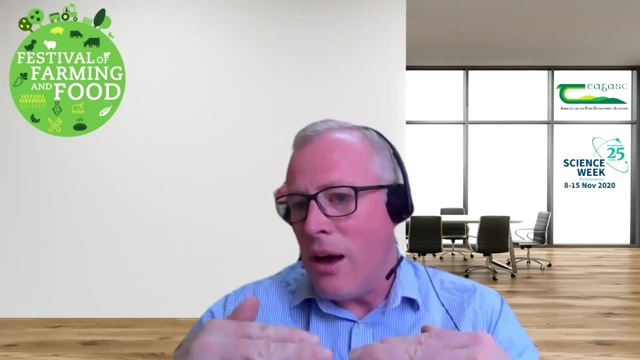 is quite important, as well as environmental sustainability. in other words, farmers are saying, yeah, we want to reduce the impact we're having on climate, but we also want to maintain our livelihoods. so I think you kind of touched on it there. how can we have both meeting? in other words, reduce, 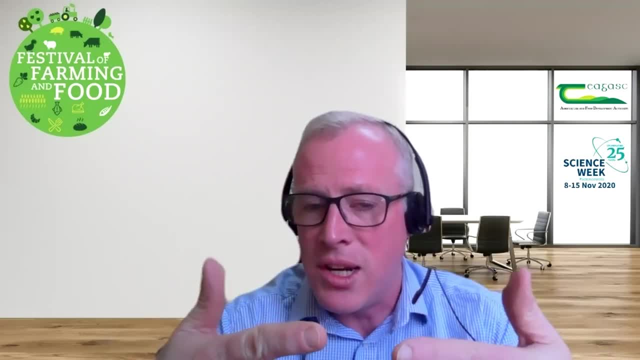 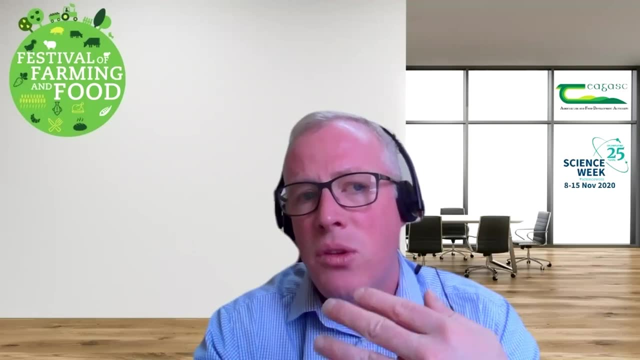 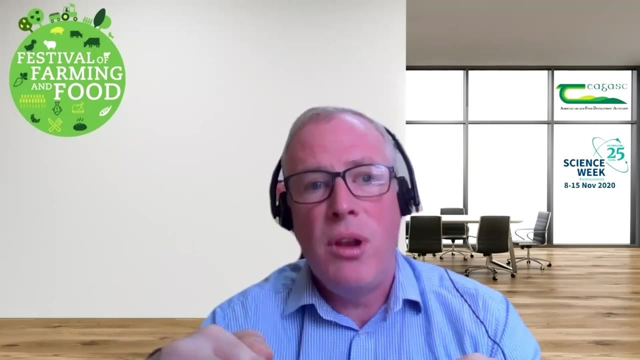 emissions and using soil quality as an example and multi-species, swords and so on and so forth, and better fertility and all of that, but where will soil, I suppose, and pasture? what sort of a role will that play in helping farmers reduce emissions while also maintaining the output that? 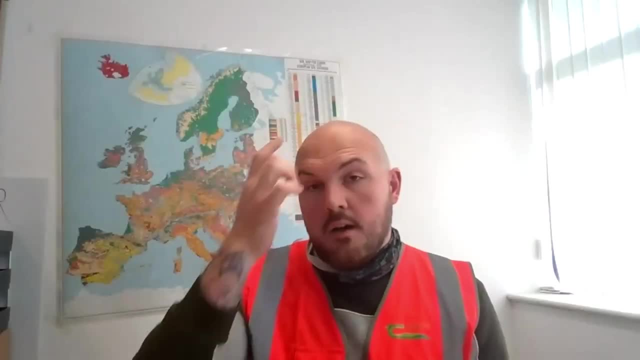 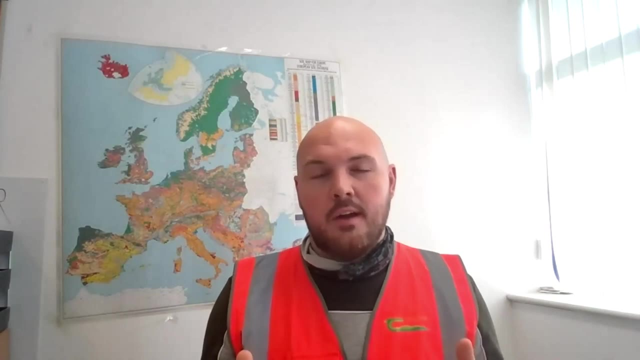 they're currently enjoying. well, I mean, it's all going to depend on your soil quality, like this has been bad. we battered the life out of that word soil quality throughout this video- and if you have a good quality soil, you are going to naturally bring your costs down, which is going to 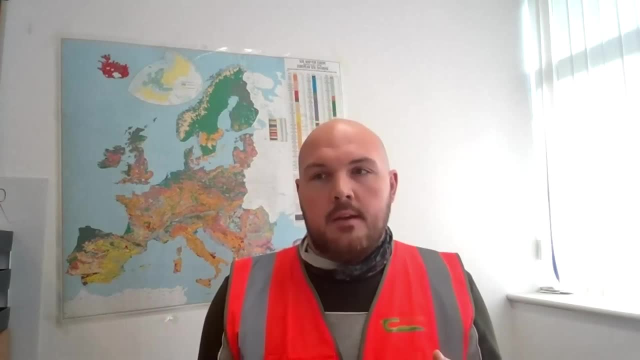 you know help you certainly maintain your livelihood. if you have a poorly managed and you know poorly maintained soil, you're constantly having to fight it by putting inputs in. you know you're having to pay for extra fertilizers, for extra minerals to get the you know to. 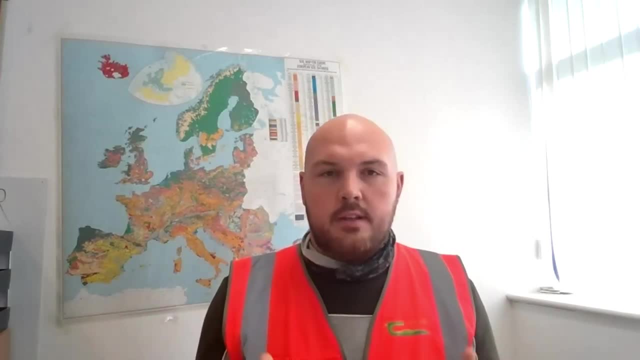 get the grass moving or your crops moving. if you have a soil that has, you know, good soil organic matter, rich in nutrients, pHs are at a good level that soil itself, as it mineralizes, will release, you know, vast amounts of nitrogen that will buffer your inputs in growing. 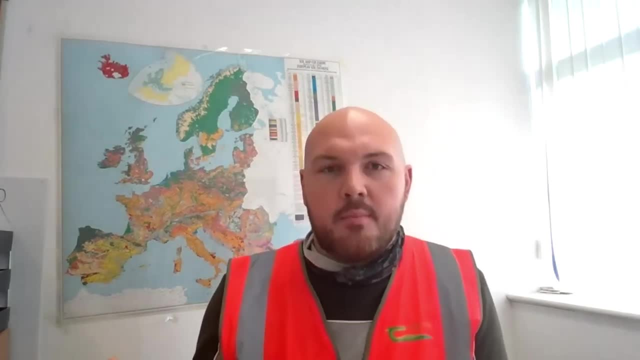 your grass or your crop. you know you're going to end up with higher yields. if you have a crop, and if it's a grassland, higher yields as well, which is going to be able to feed more cows, which is going, you know, feed more people in the long. 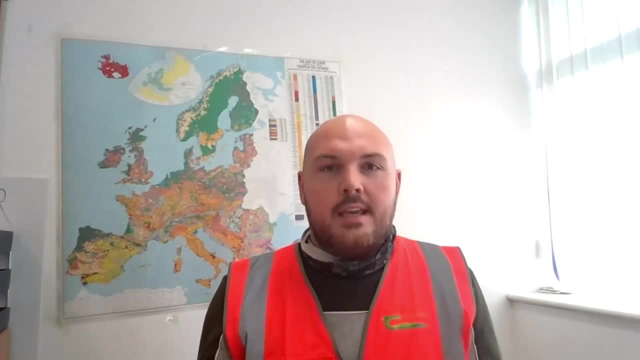 run. so, again, we're just saying if you have high yielding, good quality soils, you're going to be able to save in the long term on your inputs, which is going to benefit your pocket, obviously and, you know, will enable you to sustain your own livelihood as well as the livelihoods of many others. 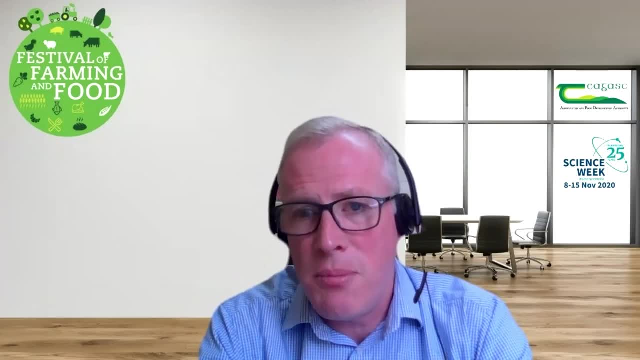 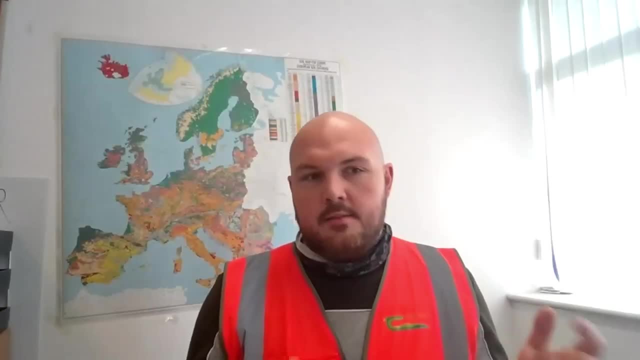 and is this something, James, that farmers are beginning to appreciate more now than they would have maybe a generation ago or even, you know, 20 years ago? yeah, farming has shifted over time. so, you know, farmers back in the day we'll say would have been, you know, great carers. 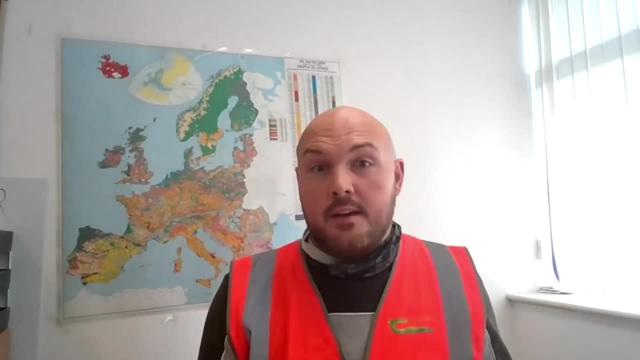 of soil and their land. you know they depended heavily on it. this would have been, say, pre-fertilizer era, where they had to take the excrement, I suppose, from their soils and reapply it to really buffer the quality of their soils. there was a period. 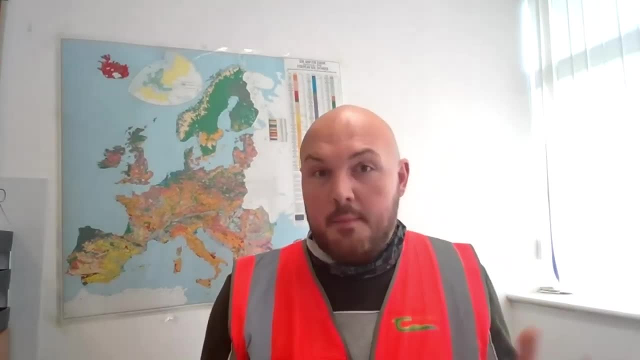 then, where fertilizers became a big thing, everybody was hammering their ground to grow whatever they needed to, but they weren't replenishing the- you know the nutrients that were needed. now there's been the shift back. now people are realizing that it's costing so much- not both environmentally- 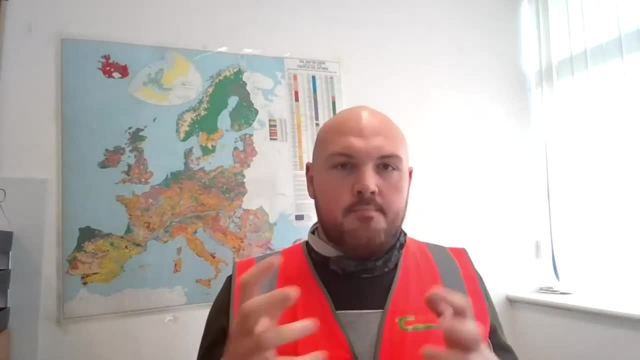 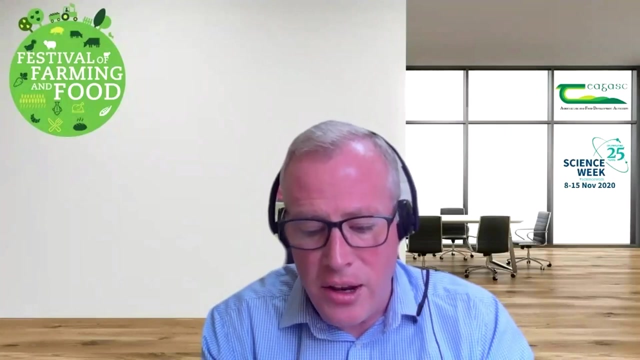 and you know, financially to have to keep trying to get these soils to be productive artificially when you can just build up your soil quality again and that will reduce your costs, right? okay, listen, we have a few minutes left and we've had a lot of questions and, as always, you know. 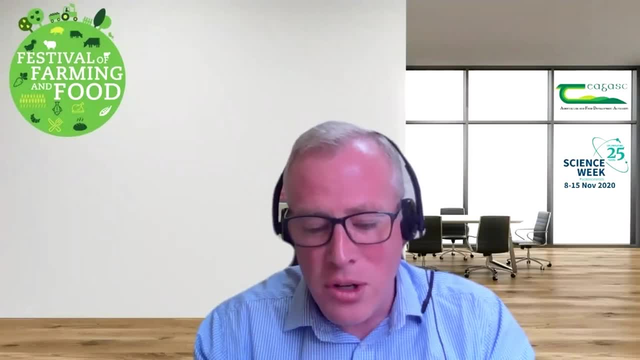 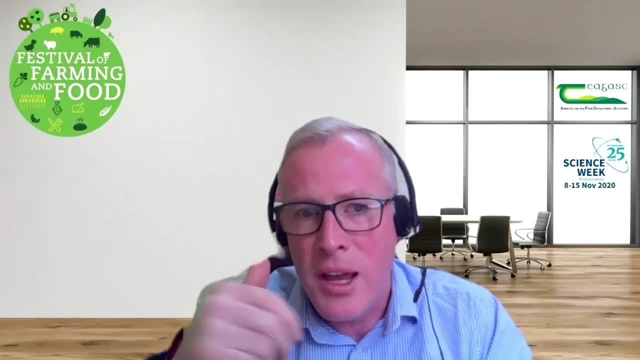 we run out of time. I get carried away, maybe a little bit, but I don't know. I'm going to just throw out a question here from Lisa: how long does it take to improve organic matter in soil? so who wants to jump in and give me an answer on that? 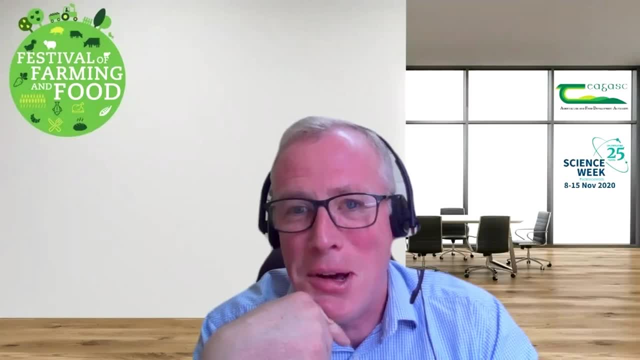 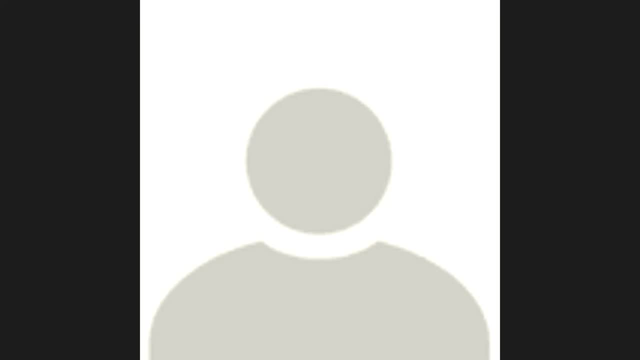 anybody, anybody. yeah, yes, Luis, yeah. so yeah, it may take, is that definitely depending on the soil? there is actually, during the last few years, a push from Europe, and especially from the French government, to just to impulse this program of four per meal. right, and this is actually. 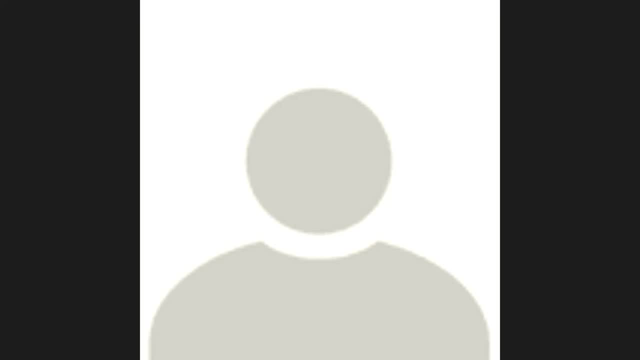 is indicating the rate in which we are encouraging our farmers to increase our soil organic matter. so four percent or 0.4 percent each year, right, so that would be. that would be a kind of a gross approximation of what our farmers could try to achieve with a good management right. 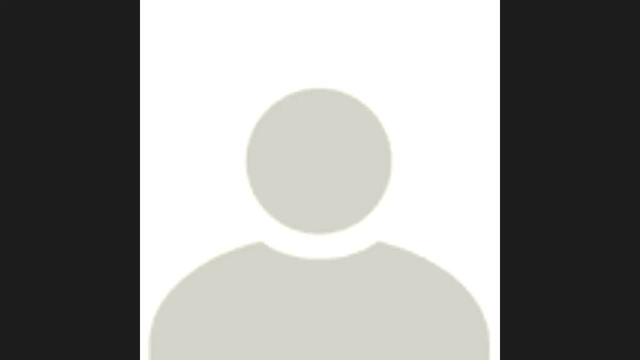 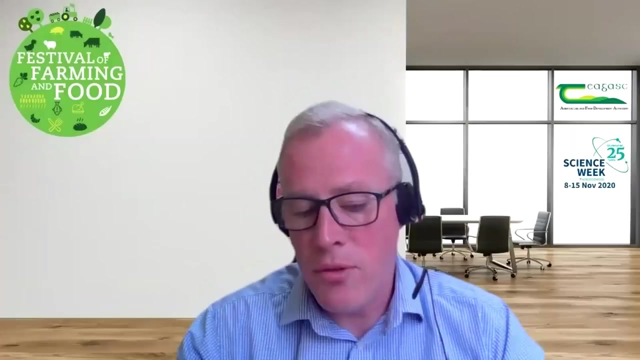 in which you are applying soil. well, you are applying like residues from agriculture, for instance, or like farm yard manure, in which you are increasing the soil organic matter content of your soils more or less at that rate. if you are are lacking, okay. okay, we have a question here from Mark. 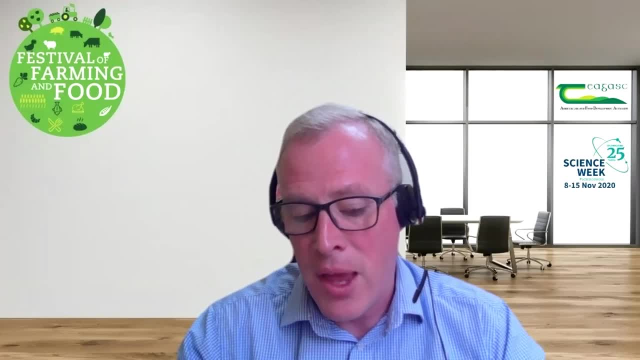 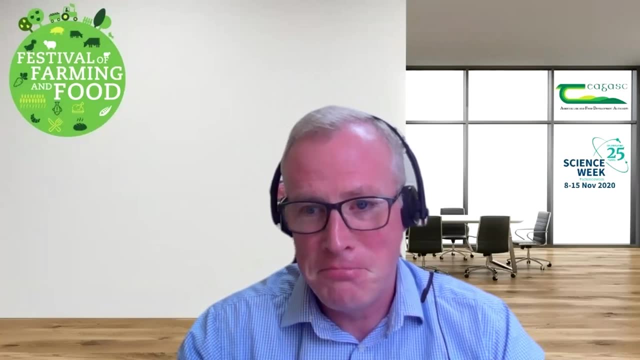 again jump in whoever wants to answer this one: how much better is rotationally grazing sheep than set stocking? I'll take that one if you're rotationally grazing sheep, then, and set stocking, I'm taking that one. a lot of things, Wegerman james, for if you're rotationally. grazing any animal. really, it increases your carbon sequestration potential because you're constantly grazing the ground, but it also gives the ground time to regenerate. So grasslands shed their roots several times in the year, And every time they do, those roots obviously decompose and 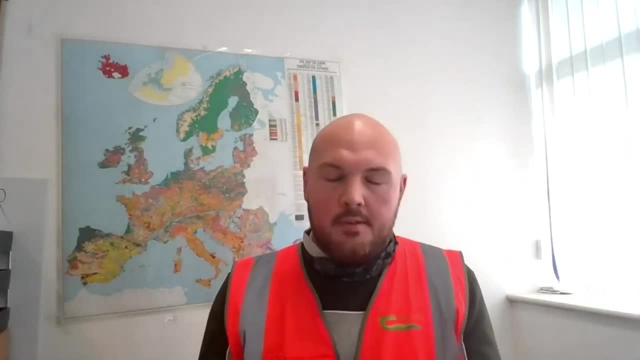 over time end up becoming stable forms of carbon in the soil. So if you're set stocking, the grass never has time to rejuvenate because it's constantly being nipped. It doesn't have that time to rebuild itself between grazings. I mean, if you look at Africa, for example, you look at 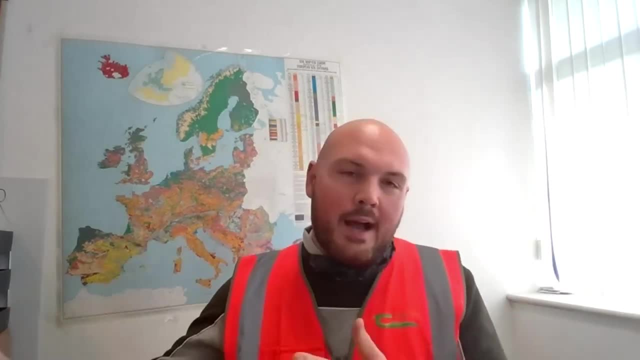 the Serengeti, you have these vast herds which pass by, who are, in a sense, rotationally grazing. They pass by, really scalp the land, but move on, allowing the land to regenerate itself behind. So, yeah, definitely rotational grazing is better from a. 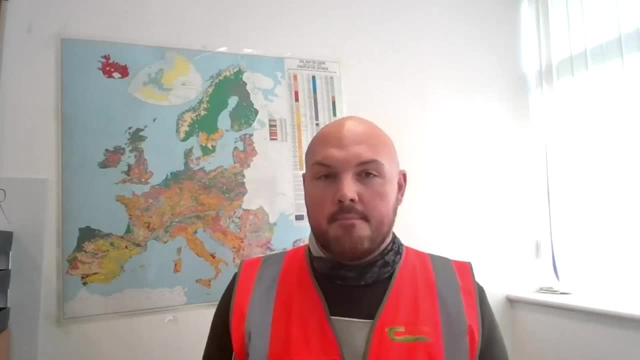 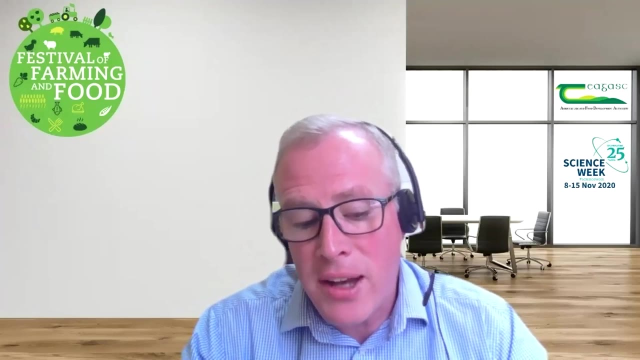 carbon sequestration point of view than set stocking. yeah, All right, James, and I'm going to chance this question for you as well, but if it's not for you, someone else might jump in. It comes in from Donna. What is the impact on earthworms from spreading slurry that has come from wormer-treated? cattle. That's a tough one. I'm not exactly qualified to answer it, but I don't think there are any negative effects because the wormers are targeted at endoparasites which live within cattle. Earthworms aren't of that same group, So look if there's anybody else that can enlighten. 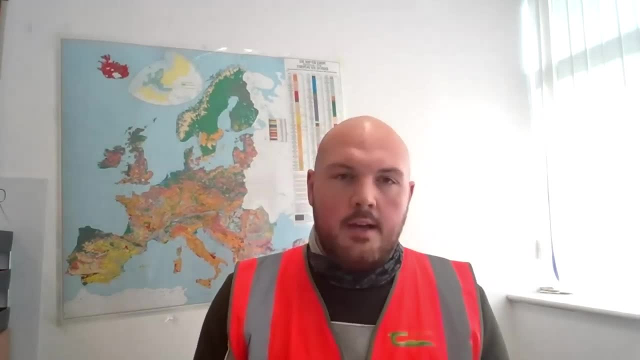 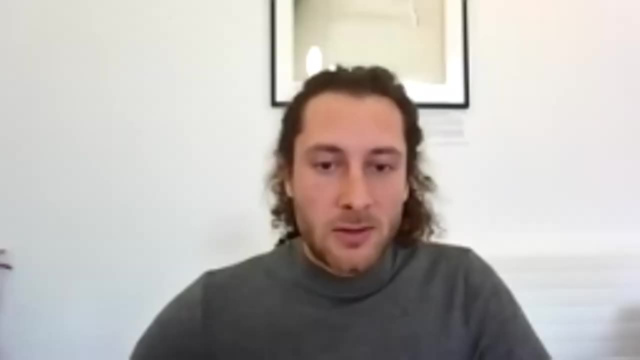 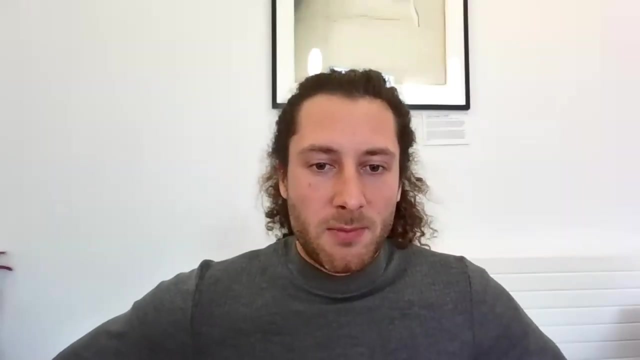 the subject. please jump in, but I don't think it has any negative effect. cattle wormer on earthworm populations- no, All right, anybody else Not to change the sorry, to just go around like in diverse grasslands. you can also insert some. species that have entelmatic effects and so avoid the application of such products, that they are not necessarily harming earthworms, but they are designed to harm some worms. So even if it's targeted, it's not going to harm the earthworms. So if it's targeted, it's not going to. harm the earthworms. So even if it's targeted to the pests of animals, it's still targeting some life and then you can have harm. it can harm some other species down the road. But yeah, just grazing some specific plants like herbs, you can have the same effects without damage on the. 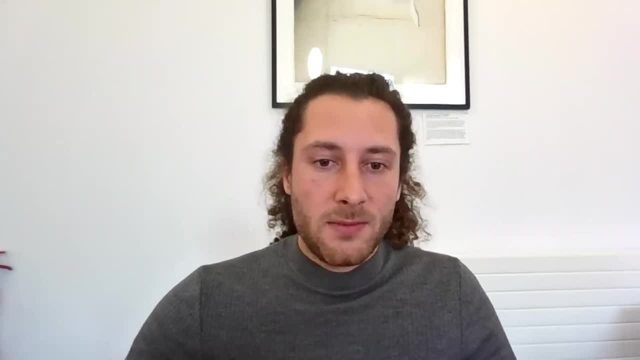 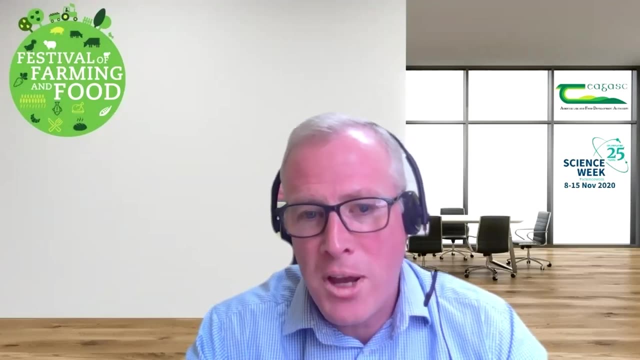 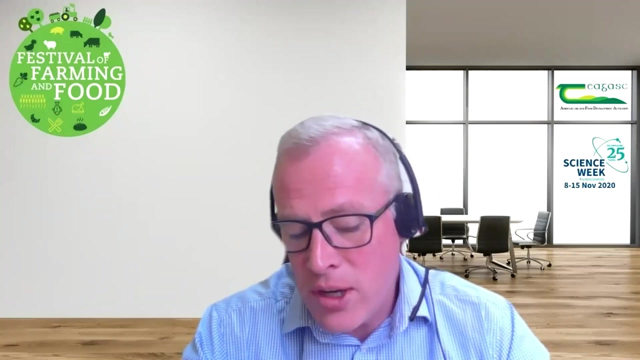 ecosystem. Okay, and anybody else want to come in on that before I go to my final question? Okay. well, it's a final question, Final question I'm going to put to you all, So maybe just in 30 seconds. It's a question from: 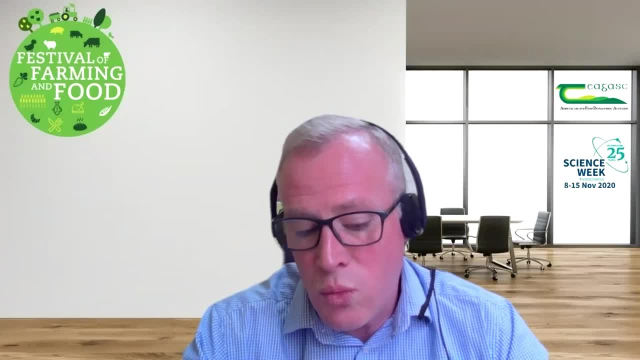 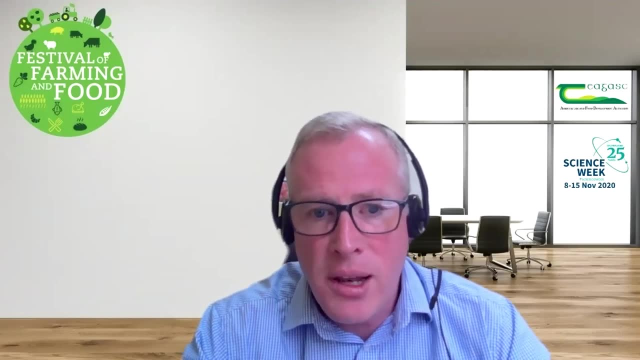 Willie, and I think it's a good one. to finish, He says: if you were to give farmers one single piece of advice that they can implement on their farms to improve soil health, what would it be? So I'll get your thoughts, Aoife. I'll go back to you first on that if you don't mind. So you know. 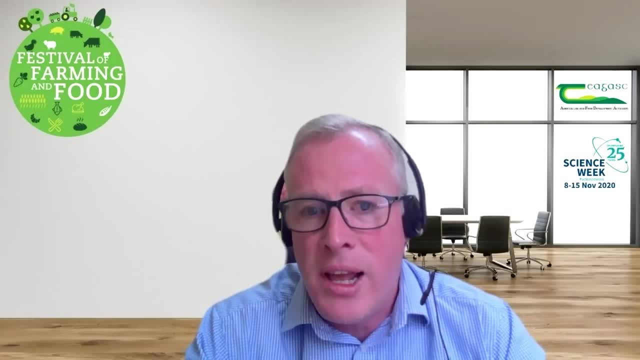 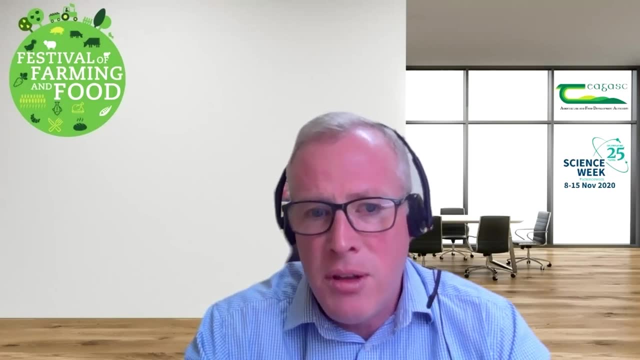 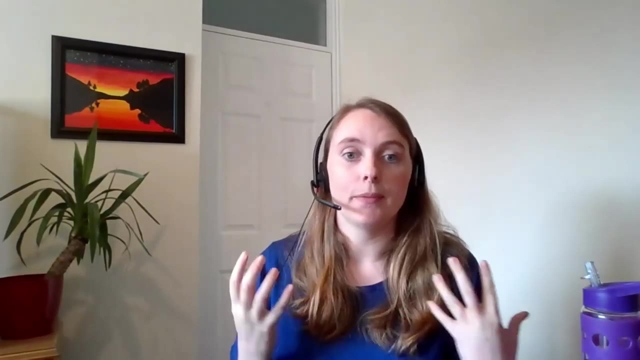 farmers asking you: what can I do? I want to improve soil health, for the environment and, obviously, to give me a better margin. What's the one key piece of advice you'd give them? Aoife Duff. So I'm going to focus on the soil microbiome aspect. Basically, my advice would be to 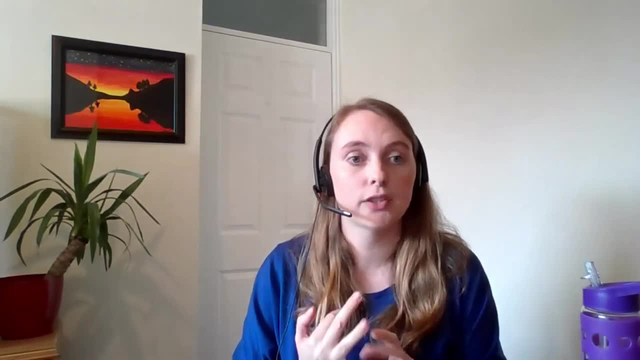 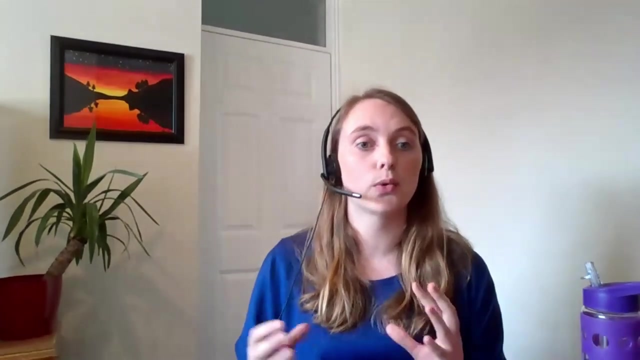 do what I said before and reduce your compaction, reduce soil erosion, reduce over fertilizing. get your soils tested and see what they actually need so that you don't fertilize or you don't over fertilize, you don't give the wrong fertilizer, that you put the right balance in. 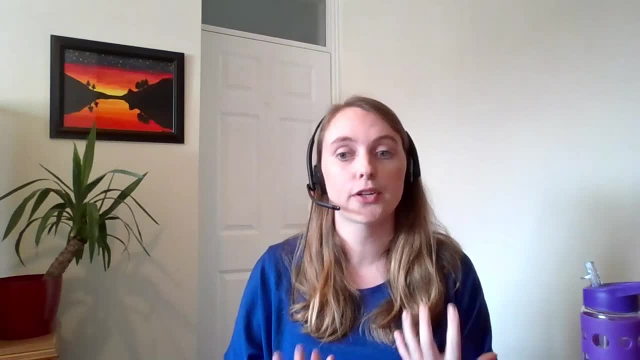 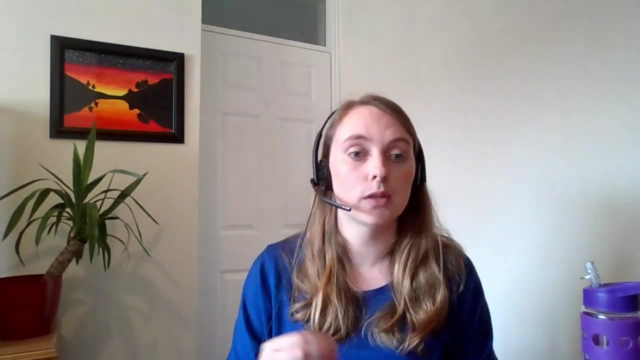 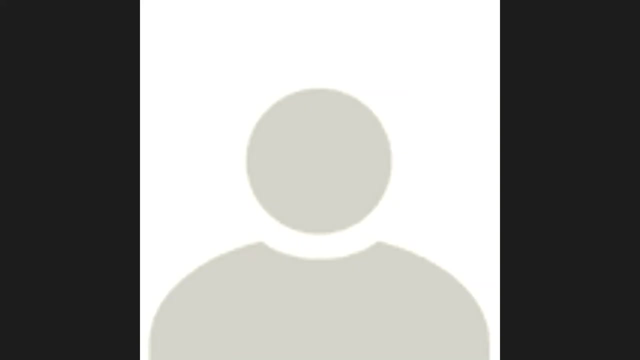 And if you can increase diversity and plant diversity on your farm, because that will also promote soil microbiome diversity. Okay, that's great, And your 30 seconds, Luis. Yeah, so it would be depending on the soil, So I would probably say that. 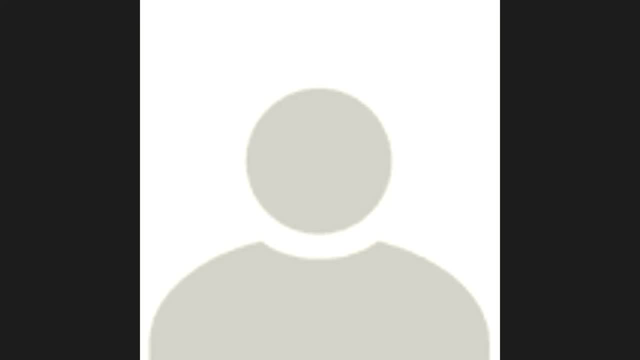 that farmer or that question to just first check what your soil is, which type of soil you have and which type of problems you are experiencing. if so, just to try to decide which is the best strategy to help growing or enhancing your soil health Here in Ireland specifically. 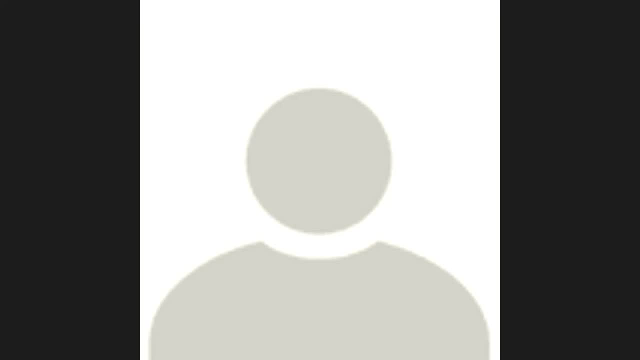 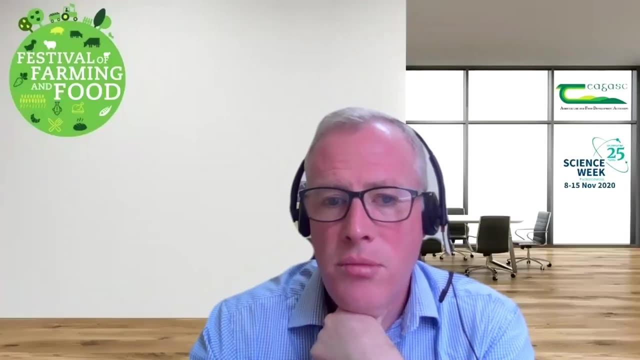 I would probably say: try to reduce as much as possible compaction through going with less trafficking on top of the soils. Okay, If it's crop lands, for instance, I would say like increase as much as possible your soil organic matter content. 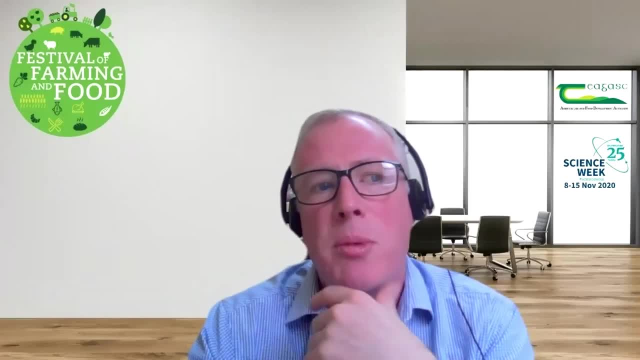 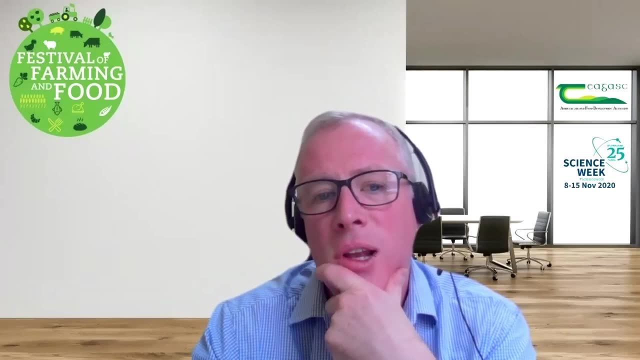 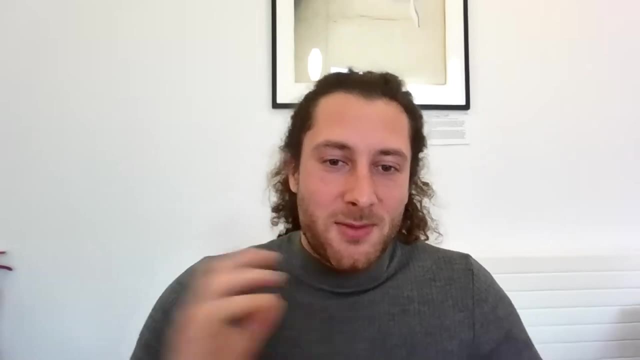 Okay, All right, And, as you said, there's no one size fits all. depends what part of the country you're in the. you know the soil changes, Ghislain. Yeah, sorry, Basically I'll not. I won't fight with the others to say: 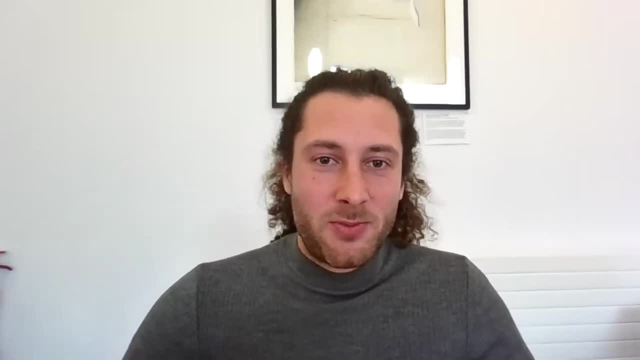 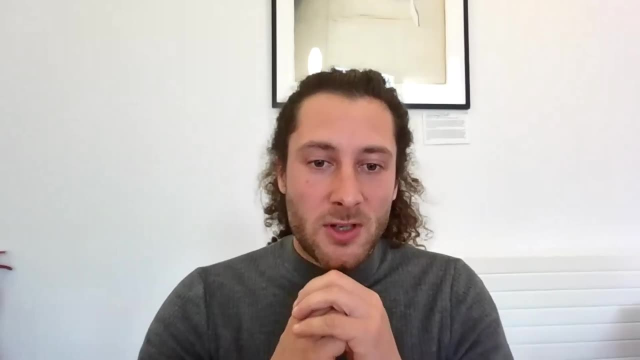 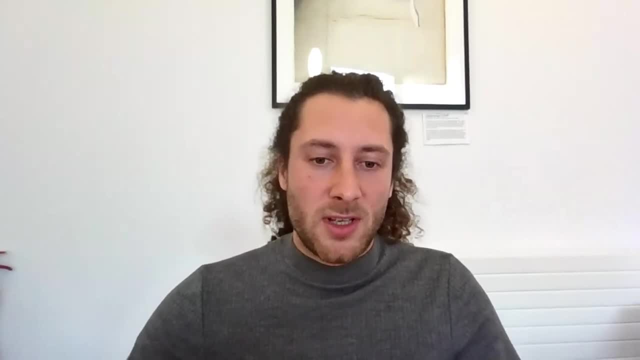 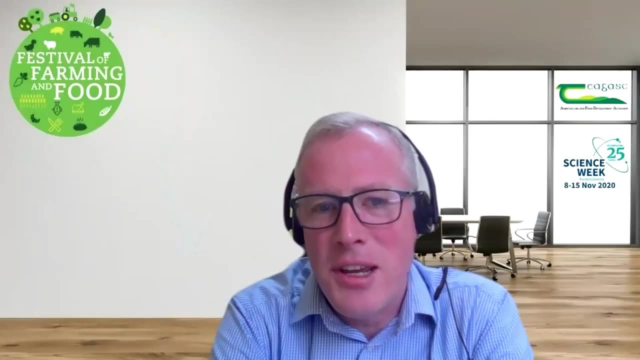 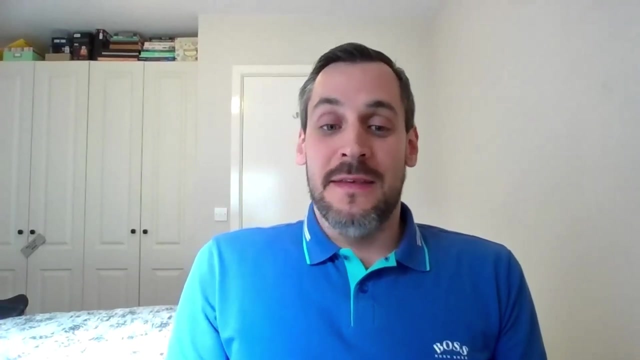 you get a full lot of diverse benefits that you will never get from one single species. So keep your soil covered and keep it covered by diverse species. Diversity is the key there. Aghi, Well, I completely agree with all my colleagues. And what else can I add? like 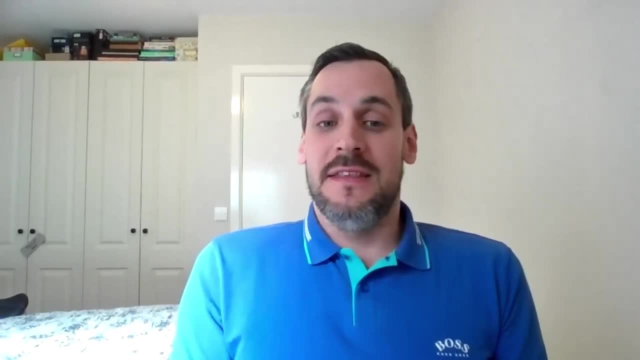 like they covered most of the things. So I would agree that maintaining soil cover would be very important and to minimize the disturbance of soil, which is already mentioned. What I could add is: well, I would suggest that, especially the farmers- 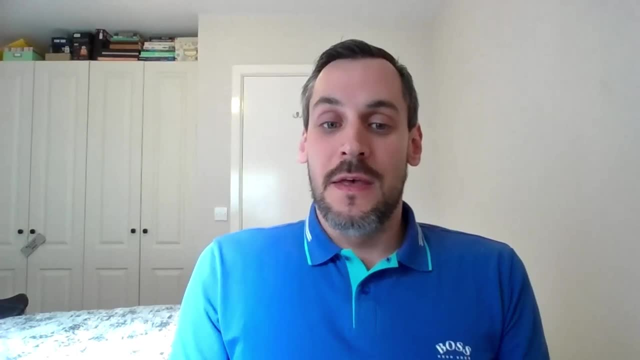 to always know their soils and test them regularly and check the fertility, know how to fertilize and when and how much and according to the needs of the plants. So, like us, like plants have specific requirements at a specific time and if they're not hungry, they won't update that. 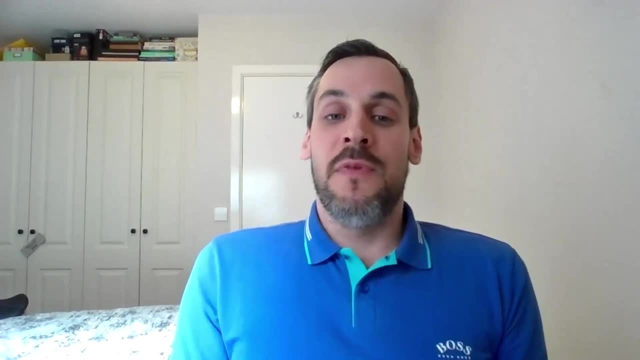 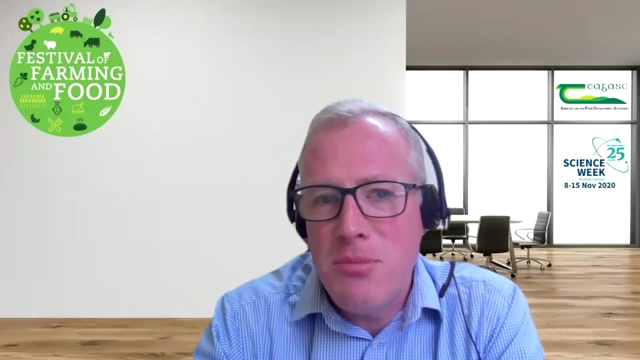 that those nutrients and then that excess nutrients is both the economic loss to the farmer, because it was applied but it wasn't taken up by plants, and that excess fertilizer or or something else can be lost to the environment. Okay, All right, And finally to you, James. 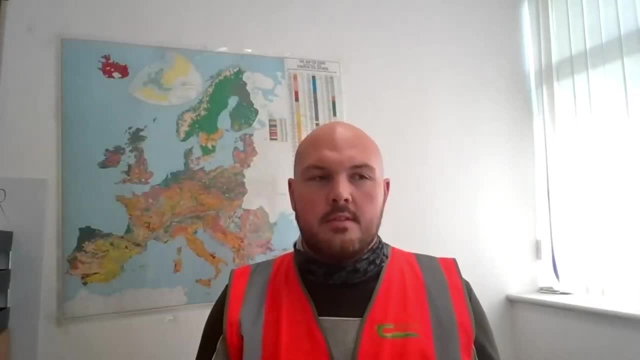 Well, look, I I obviously concur with all my colleagues, but I would have to say that balance is key. You know, if you look at your yourself, if you were to just eat McDonald's all day long, you know you wouldn't do too well on that. So definitely, as Aoife said, as Auggie said, 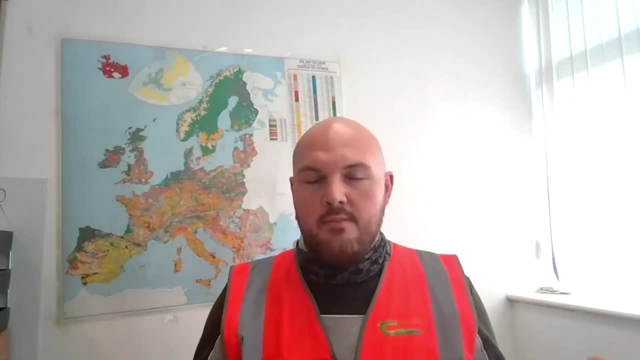 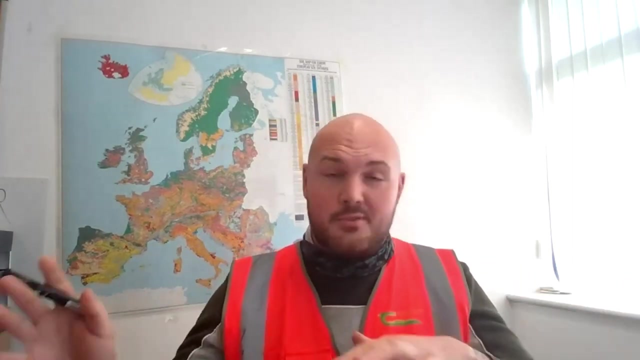 get your soils tested, make sure that you know your nutrient levels, your nutrient requirements, make sure you have all those balances correct so that the nutrients are available when they need to be available and that you know you keep that that good surface soil covered. there's no. 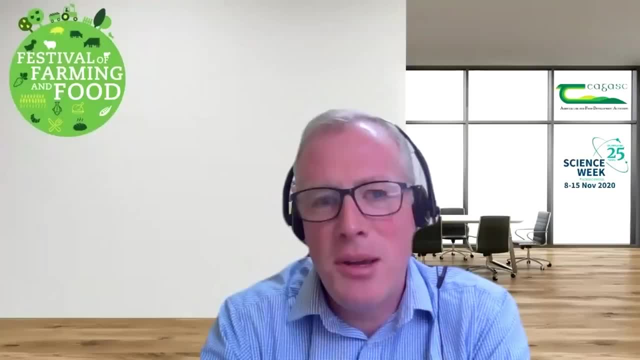 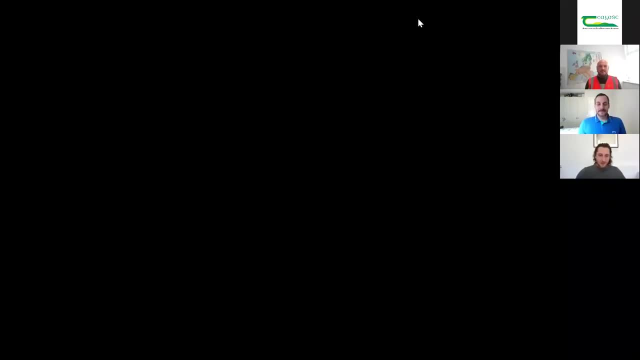 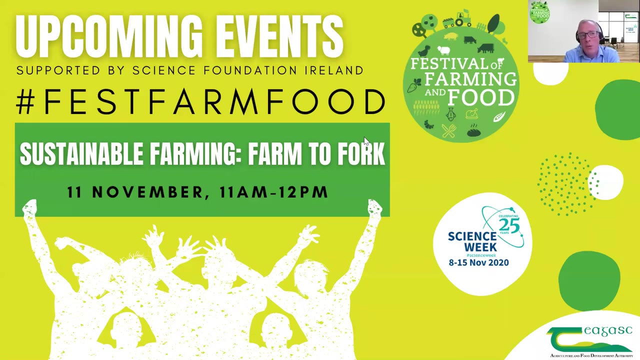 All right, Listen, guys. thanks so much for your time and great work you're doing down there And we've really been very interested in in everything that you've had to say. Thanks to all the panelists. And, by the way, tomorrow researchers at Johnstown Castle will be holding a science quiz. 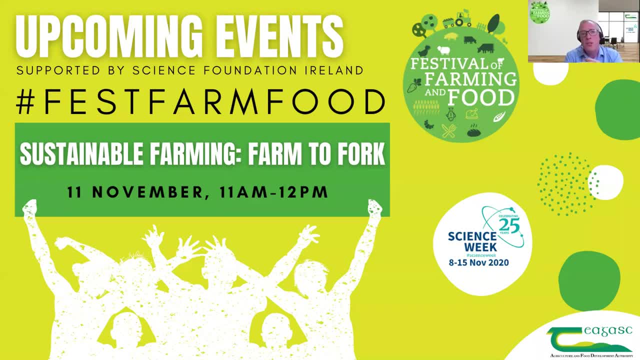 on Zoom for local schools. Also during the week, scientists from Johnstown are going to be taking part in a Zoom call, So if you have any questions, feel free to put them in the Q and A box below. And what it will be. basically that will be a Zoom call with the local schools and then ask the 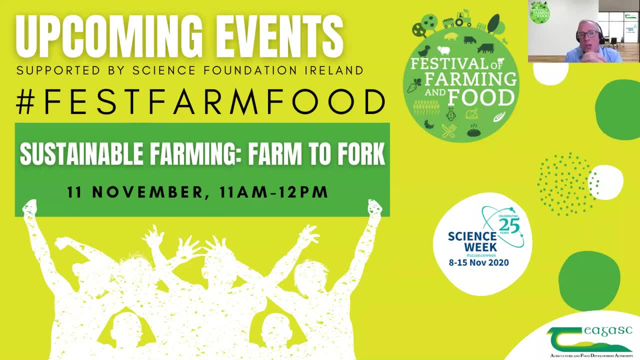 researcher initiative where students can ask them anything, basically. So teachers interested in arranging a speaker for the school should email us scienceweekchaigiscaie If you want to get your students involved in that Now. this event today and all week, has been made possible and free.